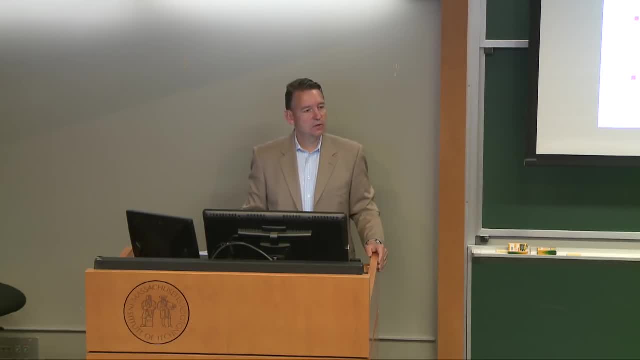 you don't really see those iterations, but they actually exist. So what we typically do at this system requirements review is review and then agree on the high-level requirements, level 0, level 1, maybe level 2 requirements, but not the lower-level ones. 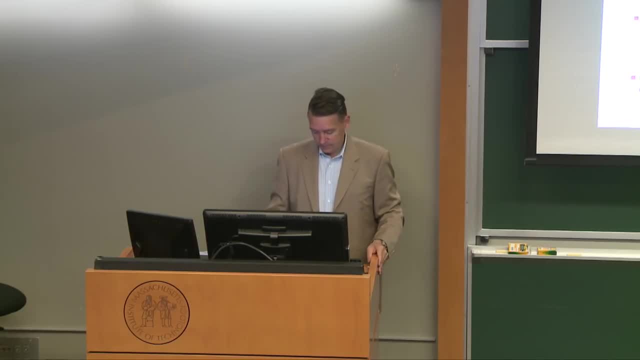 Because you can't, Because you typically haven't done the design yet. The other thing I want to say is: this is really a critical issue And a lot of the problems we talked about last time- schedule cost overruns, really a lot of these things. are traceable back to the requirements. Either the requirements were over-ambitious, you set requirements that were essentially unachievable, or you missed requirements that actually became clear later on, But they weren't written, so nobody paid attention to them. 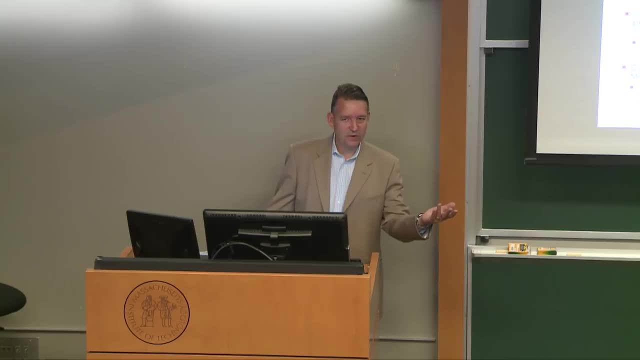 Couple examples, So I have sort of one example of poor requirements and then a good example. So this is a mission that you may have heard about, 1998, MCO. So who was born in? I'm looking at you guys, Justin, right. 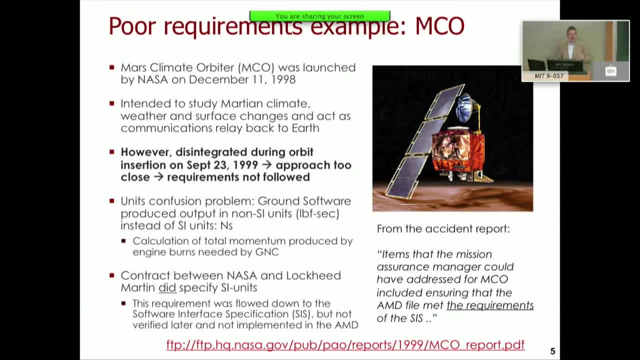 Justice. When were you born? 1998.. 1994, OK, So you're older than MCO by four years. So MCO was a very well-known, just about 20, not quite 20 years ago, a very well-known mission failure. 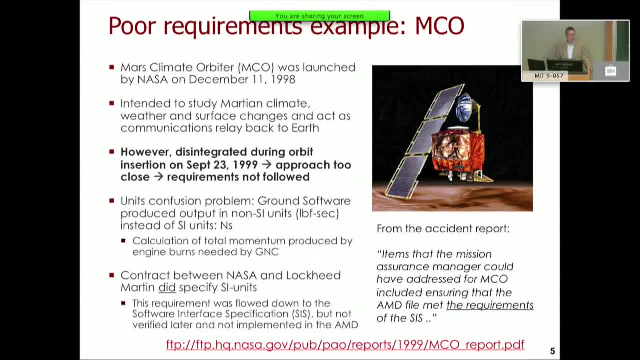 that happened. Mars Climate Orbiter: it was launched on December 1998.. And it had multiple functions: Study the Martian climate, weather and surface changes, And it was to act as a relay satellite for the Mars Polar Lander which came after it. 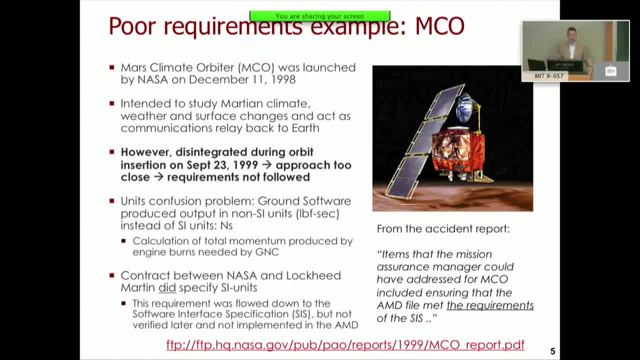 And also failed. both failed And unfortunately MCO burned up. We think it burned. contact was lost with the spacecraft after it basically entered the Martian atmosphere And there was no more communication. so we don't know for sure, But the best guess is that the spacecraft burned up. 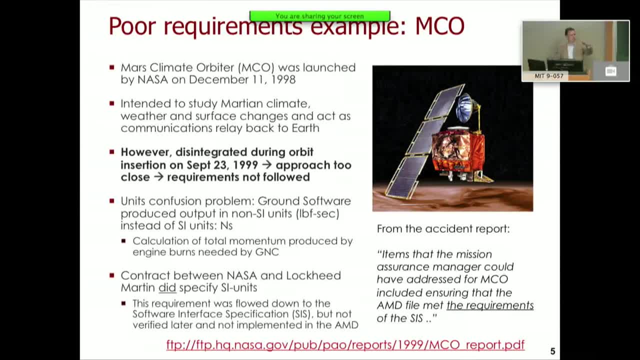 in the approach to Mars That the actual Martian atmosphere burned up. you know, on the Earth altitude at which it entered the Martian atmosphere was about 57 kilometers and it was supposed to be about 220. So, even though the Martian atmosphere is very thin when you enter at 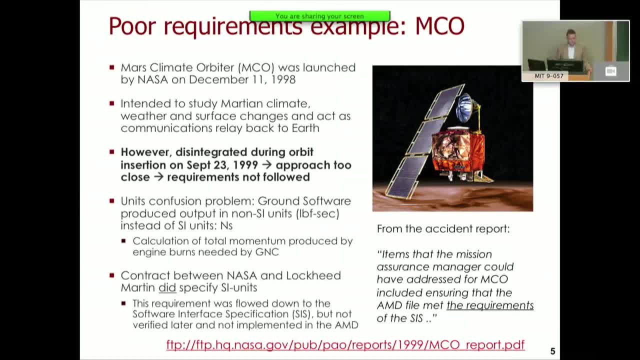 very high velocities. that's not a good thing. This is the very famous you've heard about this confusion of units problem. right, This mission that one part of the team used SI units, specifically Newton's seconds. This is momentum. right, Force, times, time That. 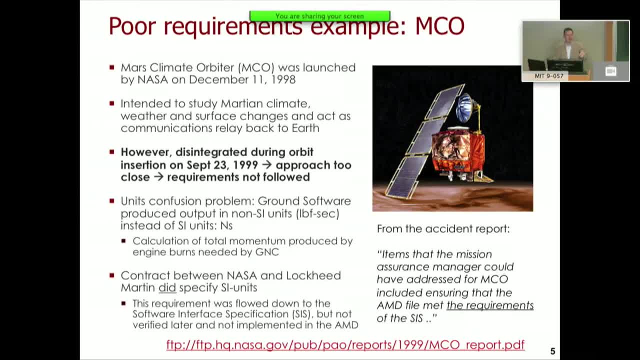 gives you momentum. So when you burn your engines for X number of seconds, the product of those two is your momentum. And then another part of the team used English units, pounds of force, times, seconds. okay, And so that was fundamentally the root, the proposition. 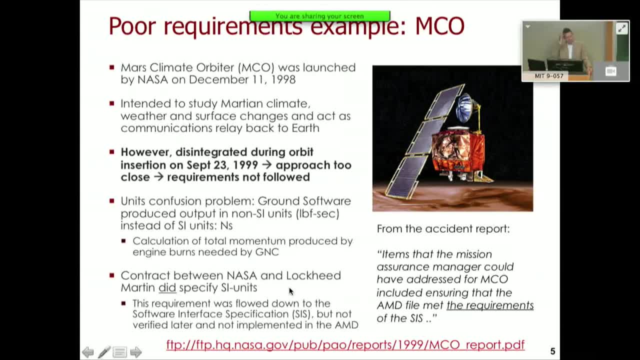 of the mission, the, the problem that caused the burn up. now, um, if you read the accident report- and i have a link here to the accident report- you will notice that the requirements were actually okay. the requirements were written correctly. so, specifically, there was a document called the software interface. 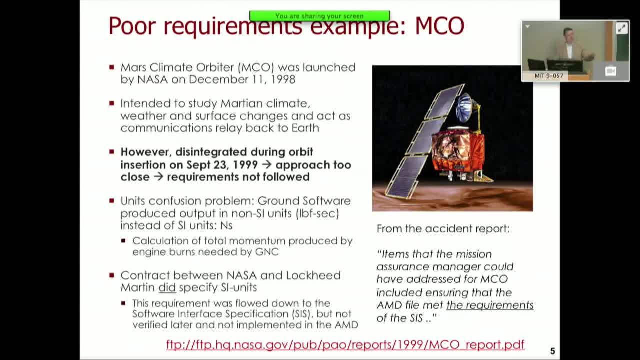 specification sis. that specified everything should be in si units on the ground segment and on the space segment, but the problem is that this was not checked and implemented, and so here's a quote from the accident report items that the mission assurance manager, which didn't exist for this. 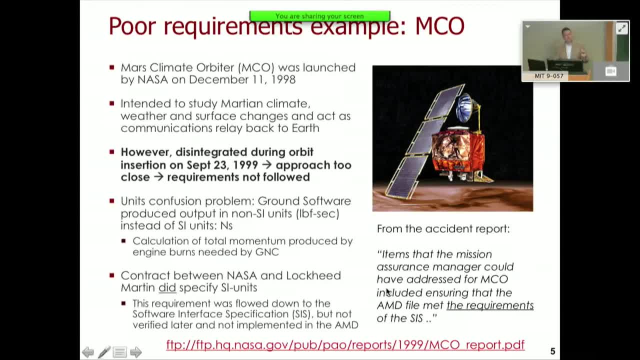 mission. so the mission assurance manager role is to make sure the requirements are actually followed. there was no mission assurance manager on the mco mission, uh included ensuring that the amd file um, which is one of the one of the files put out by the um, by the 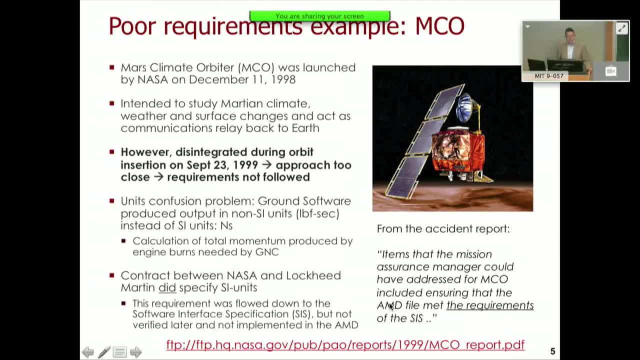 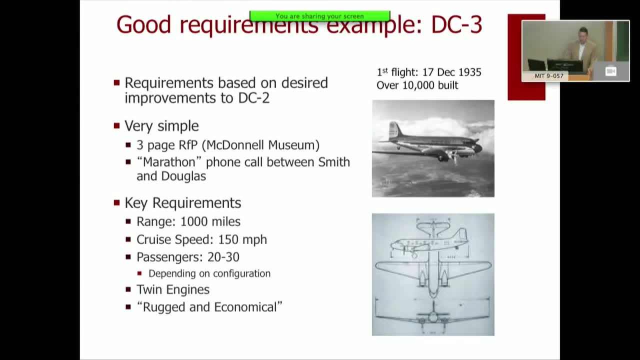 propulsion system met the requirements of the software's interface specification and that did not happen. okay, so that was um. that was sort of the root cause there. here's a a good example for requirements. this is a little bit older. uh, this is the dc3. this is an old airplane, um first flight. 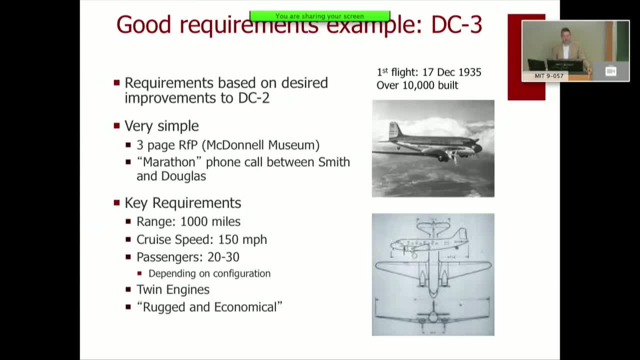 and, uh, december 1935. okay, uh, this, this was, this was really, uh, an airplane that kick-started civil aviation as a commercial service. and so, uh, the first of all, the dc3 was was based on the earlier evolution of the dc2, and i first saw this, uh, when i worked in st louis. 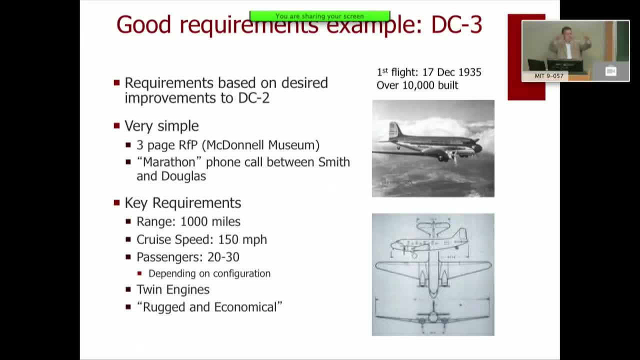 there was a little museum at the headquarters and they had like a, like a nice plaque on the wall with, with, actually a replica of of the contract- you know, the original letter that led to the dc3 contract- and, and the story is that, uh, this, these requirements, these are, this is level zero. 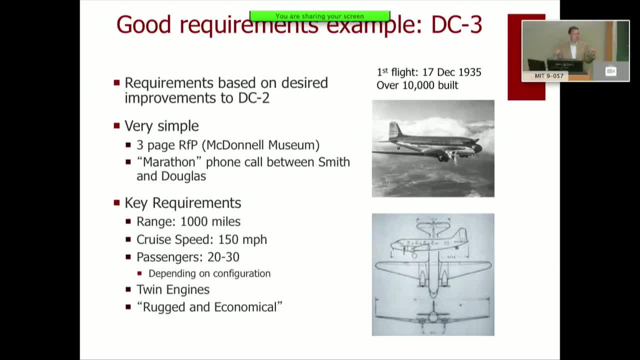 requirements. what's written here was hammered out in a single, quote-unquote marathon phone call between between smith and douglas. so smith was at the time the head of you know what was today essentially united airlines and douglas- who, by the way, is a graduate of this department here at mit. 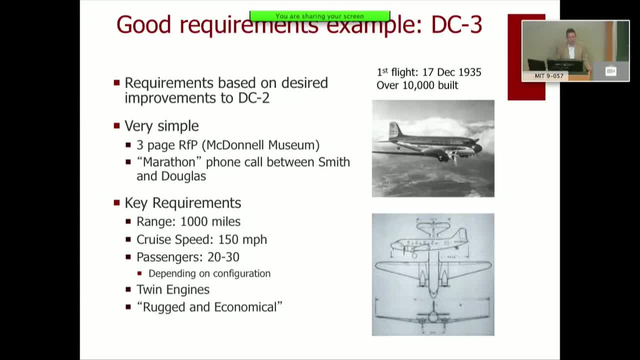 donald douglas- uh, was, was the head of the douglas aircraft company and here the requirements range about a thousand miles. so this means that you don't have trans continental range, right? if you want transcontinental range in the us, you need about how many miles like boston to san diego, seattle to miami? three thousand, yeah. 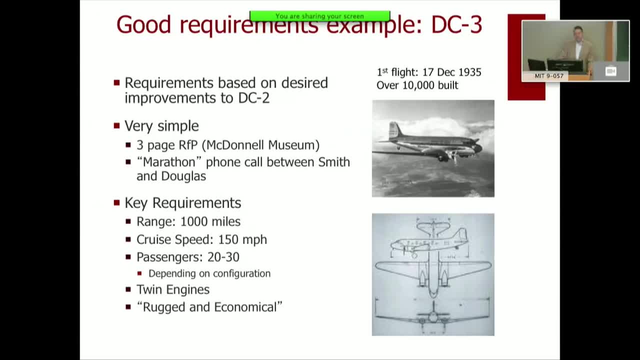 with reserve reserves, yeah, three thousand miles. so this means that if you go transcontinental with you've got to refuel twice, basically, but you know, that was okay. uh, today we we wouldn't, we probably wouldn't accept that, but that's okay. back then cruise speed: about 150 miles. 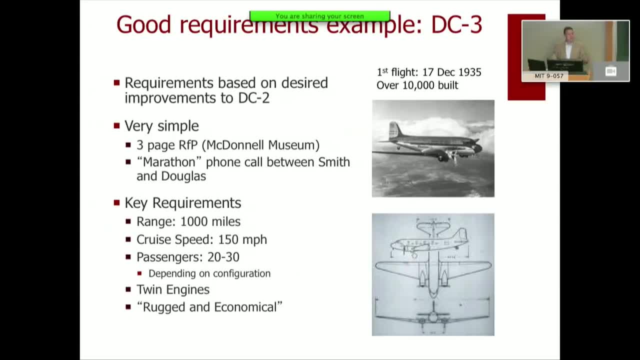 20 to 30 passengers, depending on the configuration, twin engines and then, uh, something that we would say today that's a, that's a fuzzy, that's a- not a well-written requirement because it's fuzzy, but it said it should be rugged and economical, right and and based on this sort of high level. 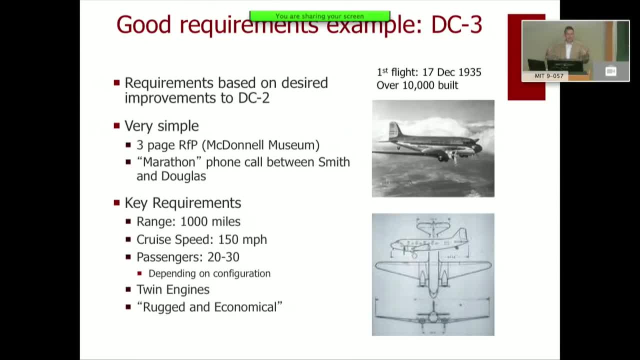 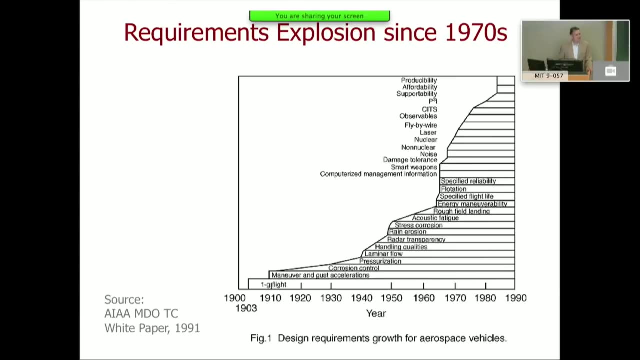 requirements that were pretty clearly defined. the airplane was then designed, built and very, very successful, and over 10 000 copies of this airplane were built. okay, so what happened since then is the requirements explosion. this is a chart from a document called the technical, multidisciplinary design optimization white paper and it's a little dated, but but the 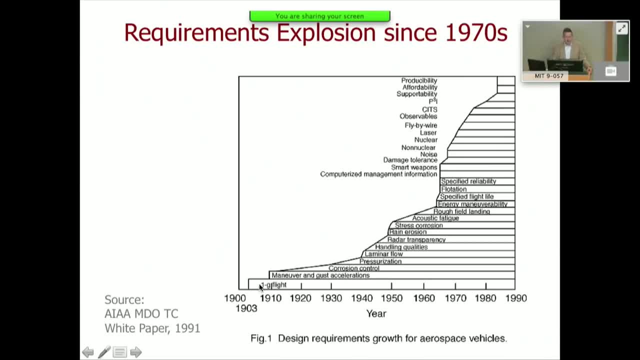 report shows that. you, why, um you milestone? well, pretty clear, after you know, not too long it was. well, we also want to turn. we don't want to just fly straight on the beach and land again. so maneuvering gust accelerations, there's wind buffeting. you got to handle those. 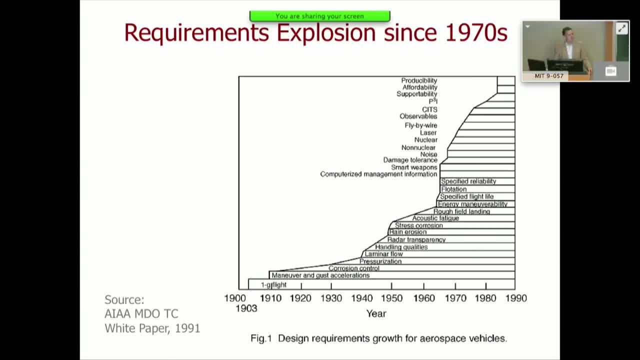 gusts, so that that's important. and then, what were the first airplanes made of? let's, let's see at EPFL guys, what the first airplanes. what materials did they use? would, yeah, what else? canvas, yeah, exactly so. then, very soon after that, maybe in the 20s and 30s, we started using metals- right, metallic structures. 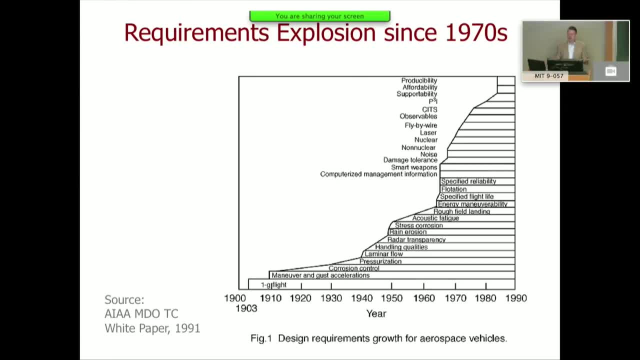 and the big issue there- especially if you're flying, you know, close to the ocean and salt water- is corrosion control. your airplanes can't rust, and so corrosion control is a big issue in the early 20s and early 30s, and so corrosion control is a big issue in the early 20s and early 30s and early 30s and early. 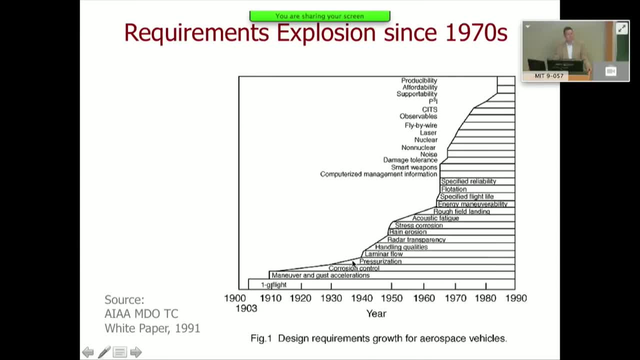 control became important. and pressurization- what is that all about? higher, faster, so at some point you need to pressurize the cabin right. that's a new requirement. the Wright brothers never thought about that. well, they didn't. I don't maybe thought about it, but they certainly didn't have to. 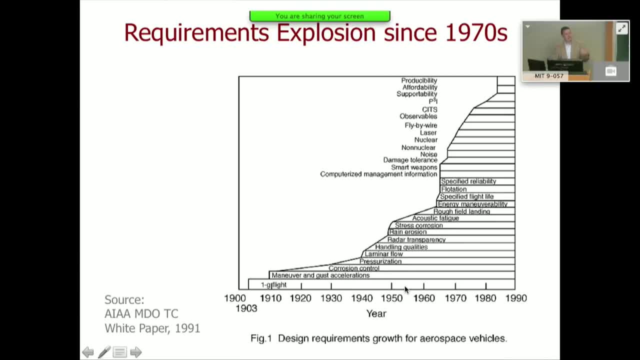 pressurize their right flyer. so you see, you see what's happening is we get greedy. you know we were excited we can fly now, but now we want to go higher, we want to stay longer, so we get greedy and we go to more extreme environments and 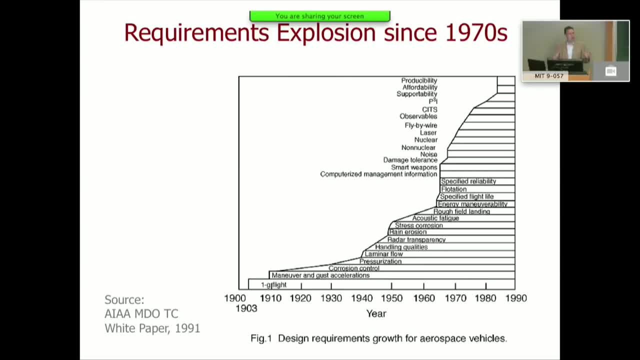 so forth, and as we do that, it gets it gets harder to do and more and more requirements start piling up. and you see a big step here. World War two, right, handling qualities, radar, transparency radar was invented, so now you want to have airplanes that are not as visible. 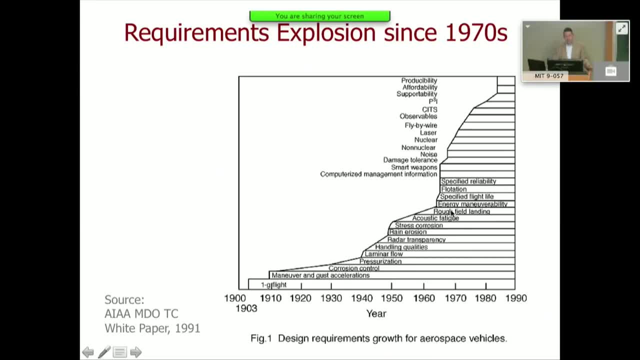 on the radar fatigue, rough field landing. and then we have another big step here in the 60s and 70s- this was during the Cold War- smart weapons, nuclear fly-by-wire right replacing cables with with electronic flight controls, and then a lot of the ilities in the last 20 years- produce ability, affordability. 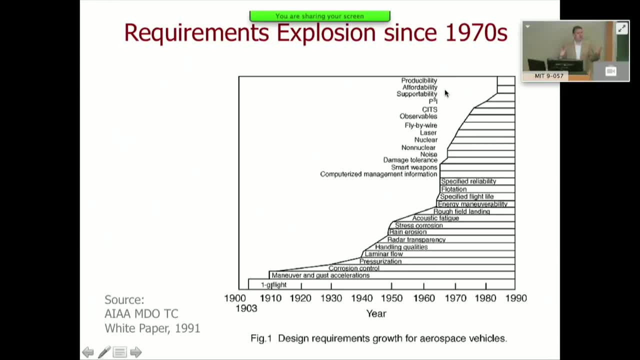 supportability, etc. so if you actually look at the requirements set for the new generation of airplanes, whether commercial or military, it's it's overwhelming. I mean it's thousands and thousands of requirements because because we've gotten greedy and we've gotten good at it, so we keep adding more. 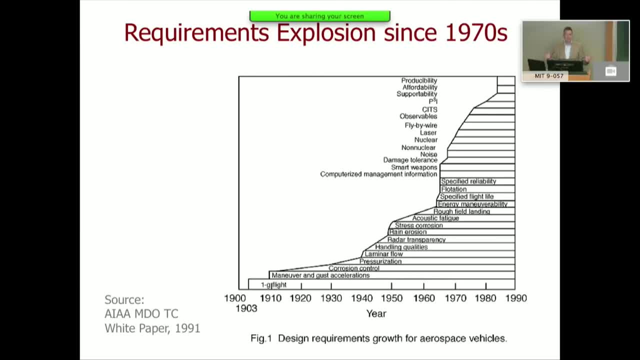 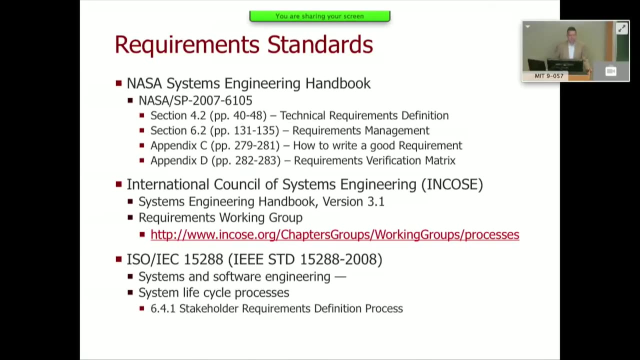 requirements and that's a big issue right now. we'll talk later in the semester about complexity management. but the key message here is: requirements have been growing over time. more and more requirements added as systems growing in performance and complexity. so here's up some standards. I won't go through those in detail, but people 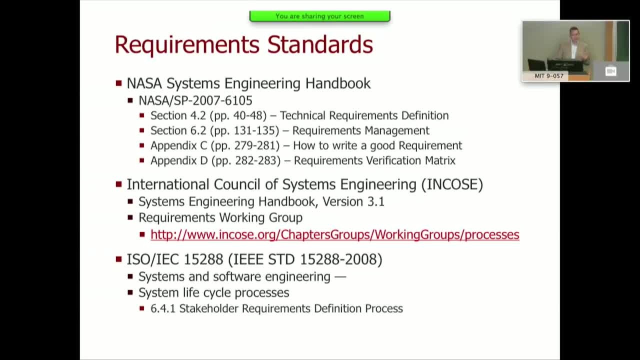 recognize in the system engineering community how important it is these requirements. so in the system engineering handbook there's two sections: 4.2, which is about technical requirements definition, and in section 6.2, which is about requirements management. so definition means that the initial definition of the initial requirements and then management is the 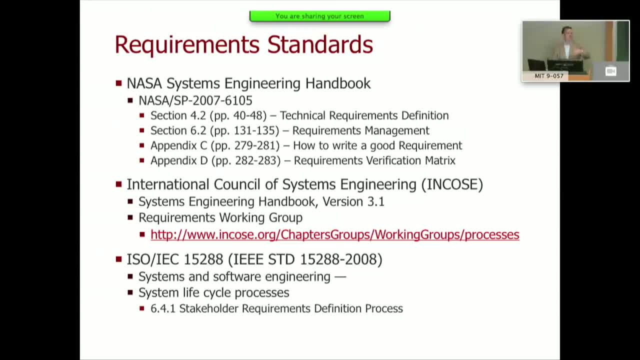 process of app, updating them, you know, adding requirements, modifying them, making sure they're up to date. on those are a couple appendices. in COSI, the International Council of System Engineering, has in the handbook a whole section. there's even a requirements working group, people who really specialize in this, and then as well in 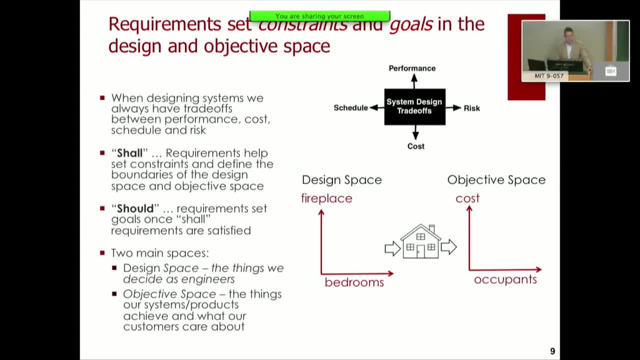 the ISO standard. you have a lot written about requirements, so this is really a big deal. so the last thing I want to do here in this section is to sort of, at a very high level, communicate to you what requirements really are about. what they are about is: 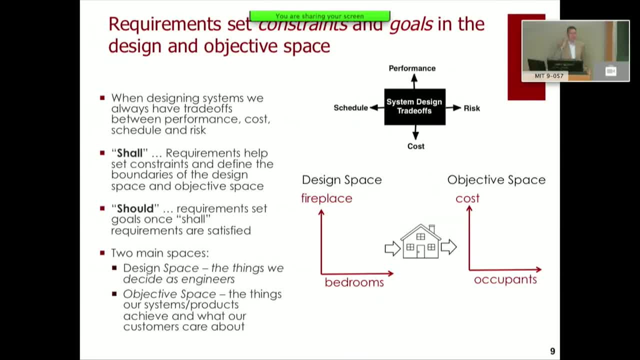 you know, like I said, don't set off in your ship without you don't know what port you're sailing to, right. so requirements set goals and constrain the design and the objective space. so, whatever, whatever you're designing, you're always going to have two spaces that you're dealing with: the design, 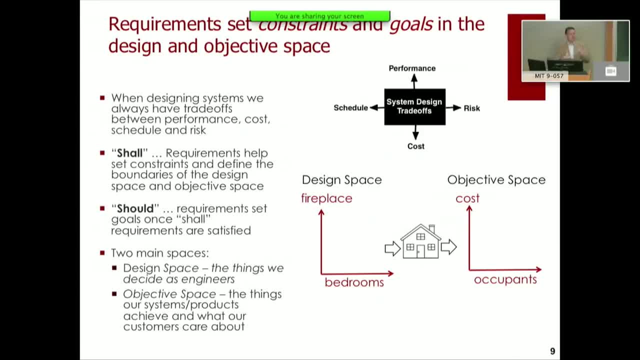 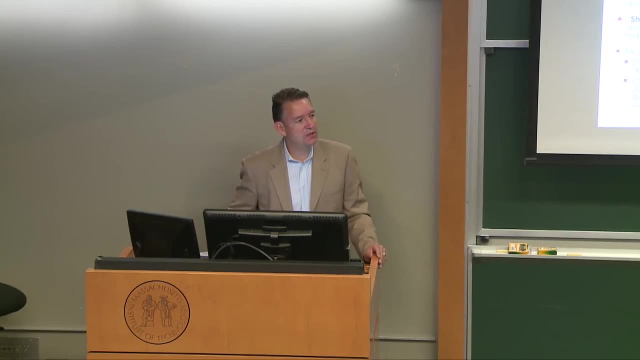 space on the one hand. that's the things you can choose as a designer- right, these are the knobs you can turn, the decisions you can make. and then the objective space, which is the things that essentially your customer cares about. you know, I'll give you a quick example here. so when we use the word 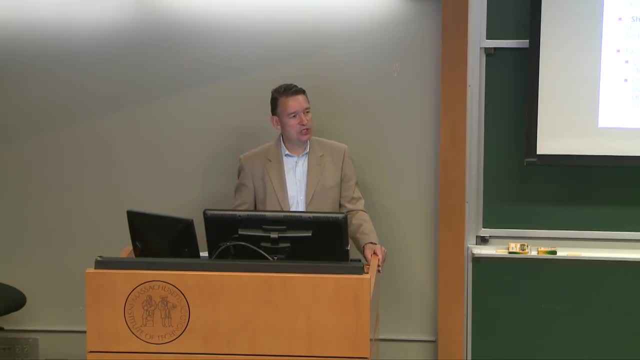 shell, which I'll get to in a minute. the English word shell means this is essentially a constraint. you must accomplish this and if you use the word should, it's more like a goal. it would be nice to do this, but it's not absolutely mandatory. so shell is a hard constraint. should is desirable and as a goal, so let 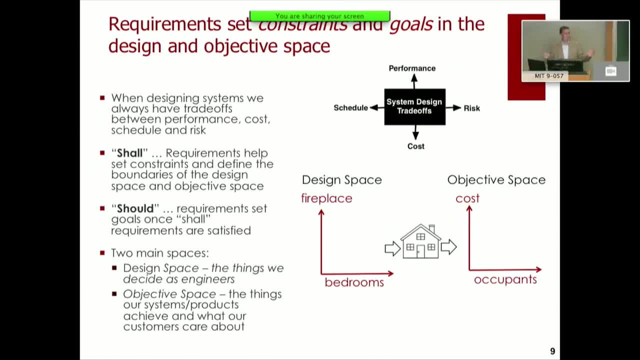 me give you this quick example here. so let's say you're designing a house, you're about setting off to design a house, and what would be some requirements for a house? so I wrote four of them here and and I'll map them to the design space in the objective space. first requirement: the house shall sleep. 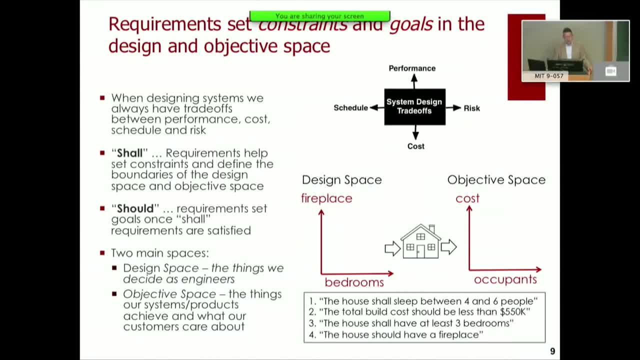 between four and six people. well, is that in the design space or in the objective space? that's an objective space, right? yeah, that's right. so here we have an axis called occupants, right, so four is the minimum and six is sort of the maximum. so that's the upper bound. 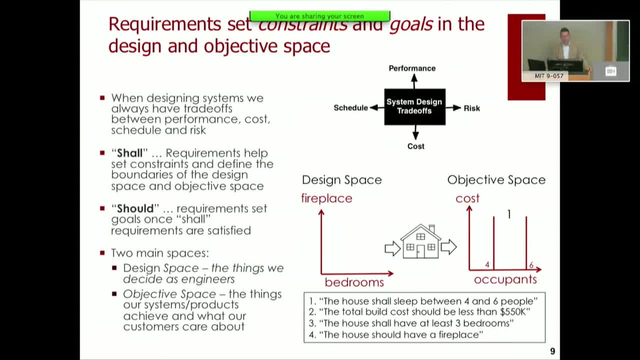 the next one. the total build cost should be less than five hundred and fifty thousand dollars should be. what is that? maybe at EPI FL? it's a goal, yeah, that's right and it's it. is it in the design space or the objective space? objects, objective space. that's correct. so I put this as a dashed. 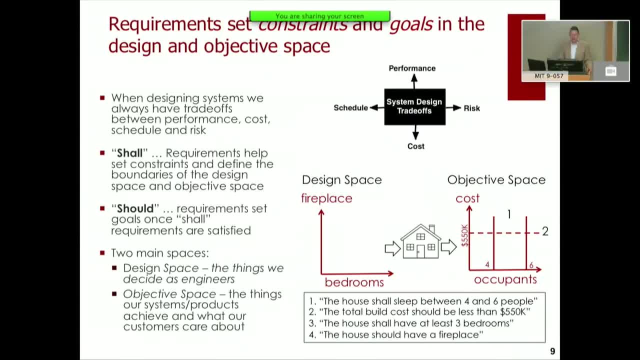 line okay, because it's a should. so what I've done here, just by writing these two sentences, these two requirements, is I've essentially carved out a space right and I can shade that box. basically, what these two requirements do is they put a box around in the objective space, saying 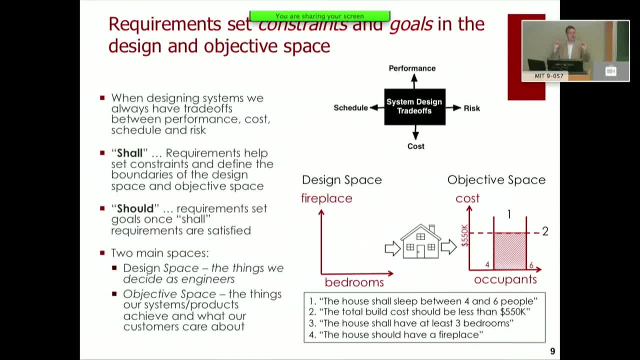 that whatever house you're going to design, it has to fit within this, within this box. okay, then the third one is: the house shall have at least, at least three bedrooms. what is that in the design space, or objective space? design space- right, because this defining a bedroom is a design decision, right? and then this: 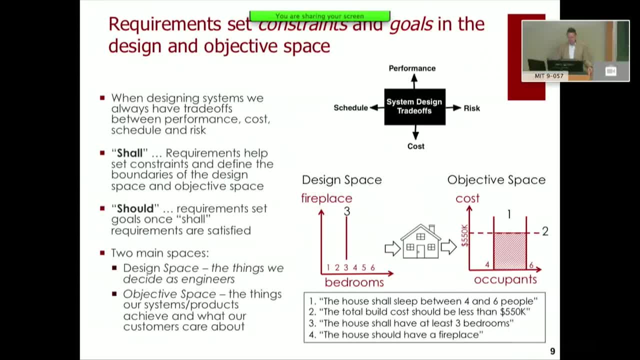 this: the house should have a design space and the design space should have a fireplace, so you can show the the lower bound here at least three bedrooms and then the fireplace is a is. it would be nice to have, but you don't actually absolutely have to have it, so you can sort of draw this. it's more like a line. 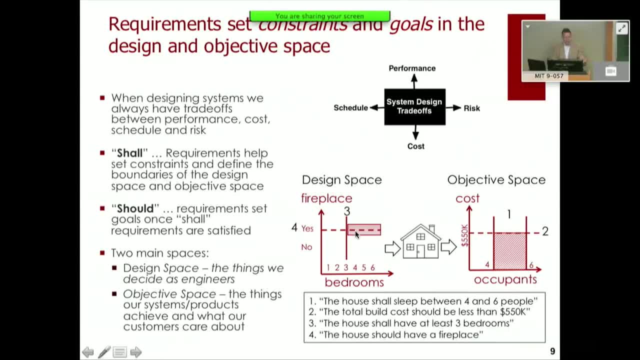 here, right? yes, fireplace, but it's a dashed line. and then at least three bedrooms, right. so just these four sentences. we've now put a, we've defined the space that we're going to be designing it. so we have constraints in the design space and we have constraints in the. 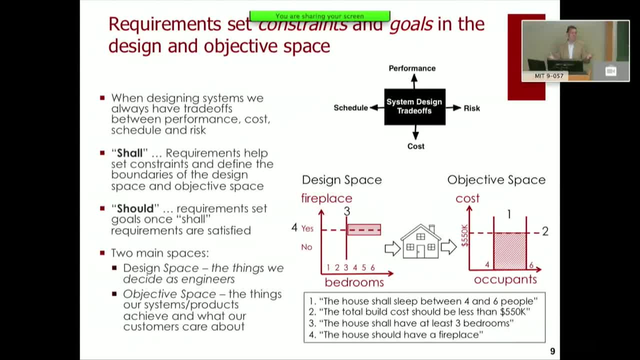 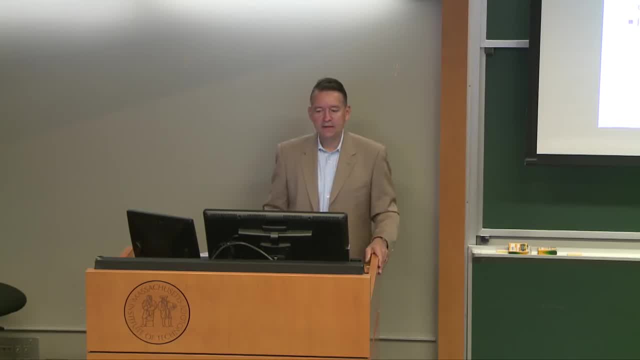 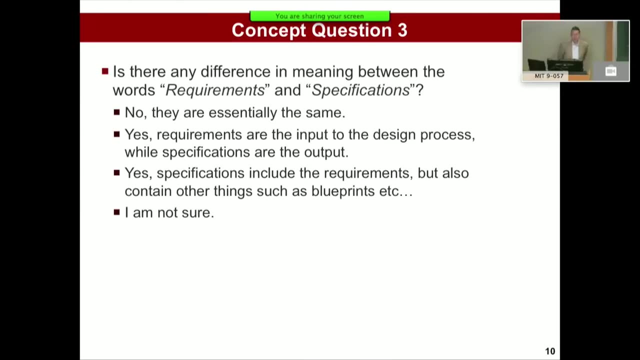 objective space- and that's fundamentally the role of requirements- is the constraint to give us direction as to what we're going to design. okay, so let me, let's do our first concept question for today, and that's the following question: do you think there's a fundamental difference in the meaning? 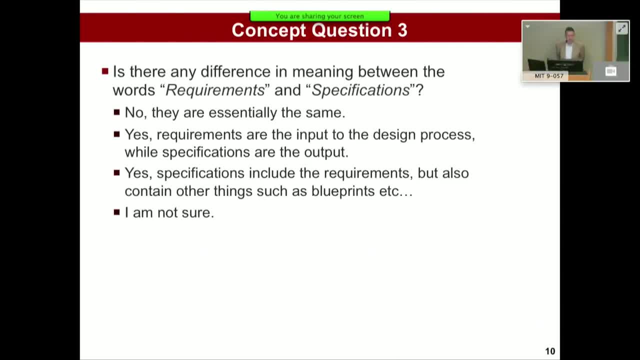 between the words requirements, which we've talked about so far, and then the specifications, which I haven't mentioned yet. so no, you think they're essentially the same. yes, there is a difference. requirements are like the input, and specifications are the output of the design process. yes, you think a. 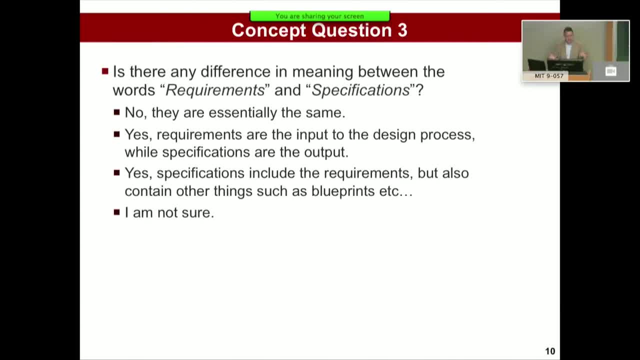 difference specifications include the requirements as a subset, or you're not sure. so think about this and then submit your answers. and as far as these URLs are concerned, for the concept questions, I went to all lowercase. hopefully that's a little easier. so, SECC 3- tiny dot CC. SECC 3: what do you think? requirements? 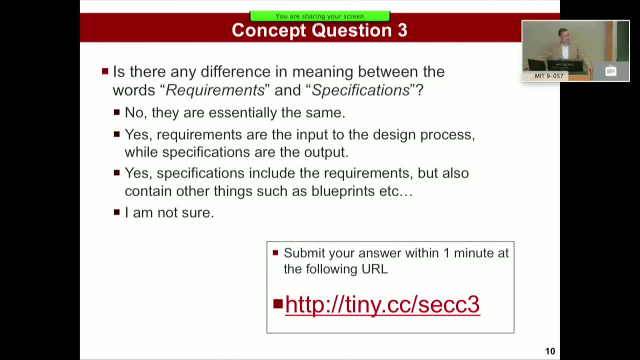 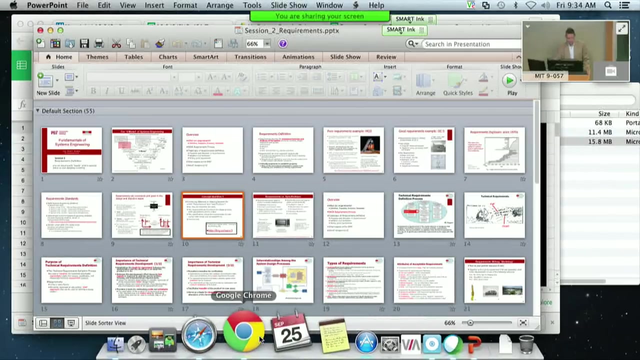 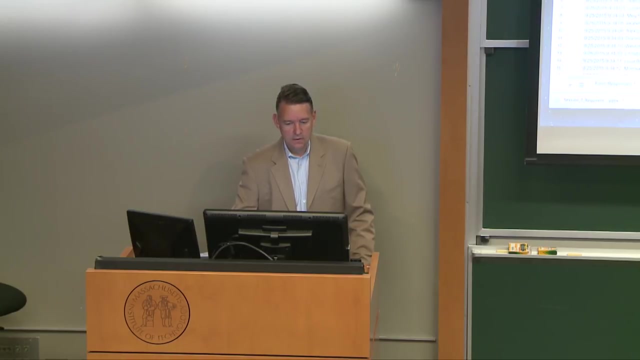 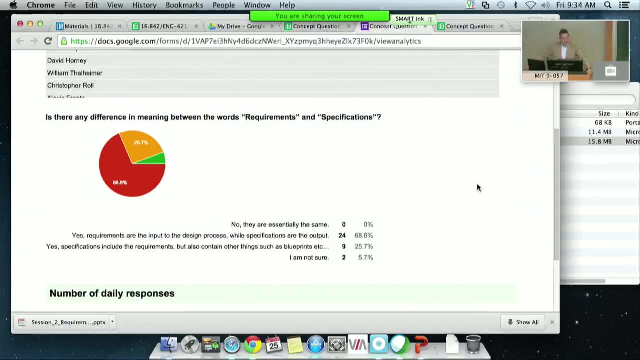 and specifications same thing or not? you need more time, anybody. who needs more time? anybody, okay, Okay, so we have nobody thinks they're the same. two-thirds of you think that requirements are the input, specifications are the output. nine of you think that requirements are a. 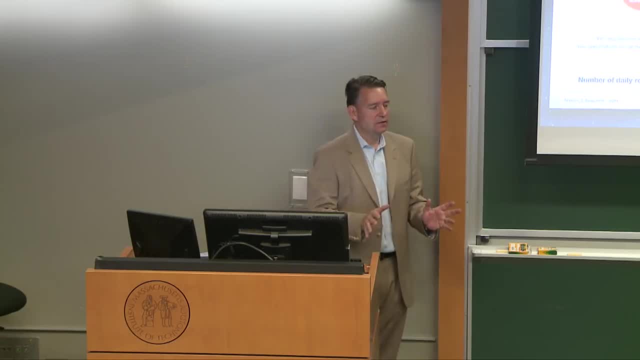 subset, and then six percent are not sure. So that's good. I agree with that. So a lot of people use requirements and specifications as the same thing. they're really not. So think of requirements, as you haven't actually started the design yet. 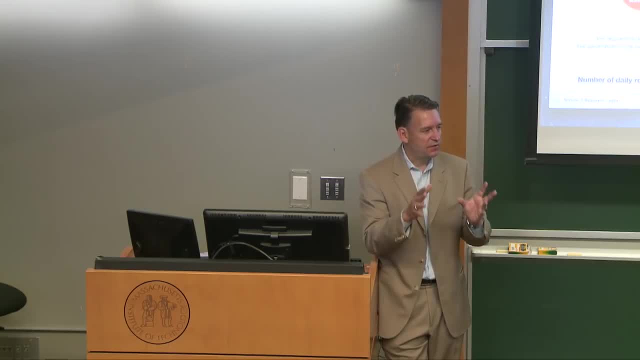 This is your putting constraints of the design space, defining the direction, but you don't actually know what the design will look like. Some requirements may say you must use this box or you must use this sensor, and you might actually find some of those in the CANSAT. 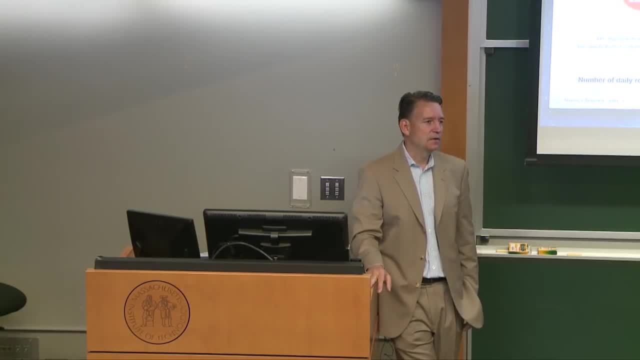 But basically the requirements are the input. So what are your experiences? When have you heard those terms, requirements or specifications used interchangeably or not interchangeably? Has this come up as an issue for you before? Marisa, you've worked on human space. 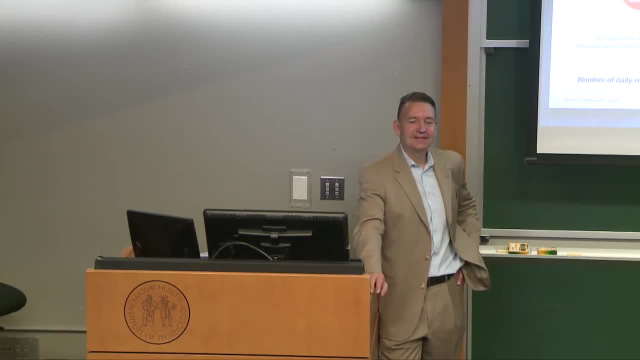 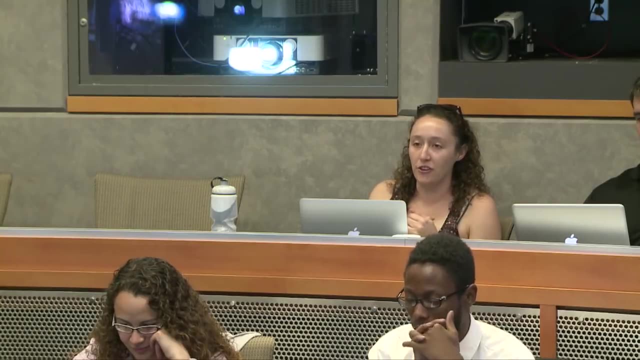 Yes, Space flight right, Space tourism vehicles. So how did you guys do it at Virgin Galactic? Well, I think something that you generally saw was people would look at sensors and there was a specification for a sensor and they would not necessarily compare the requirements. 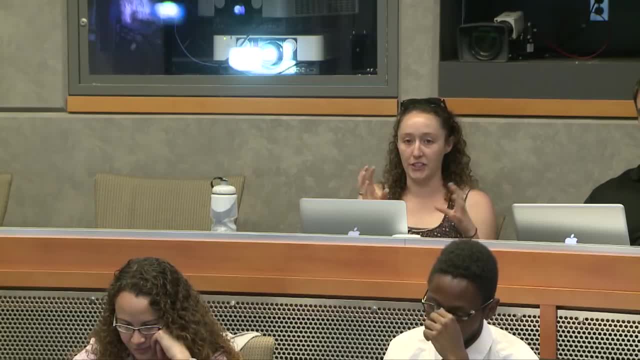 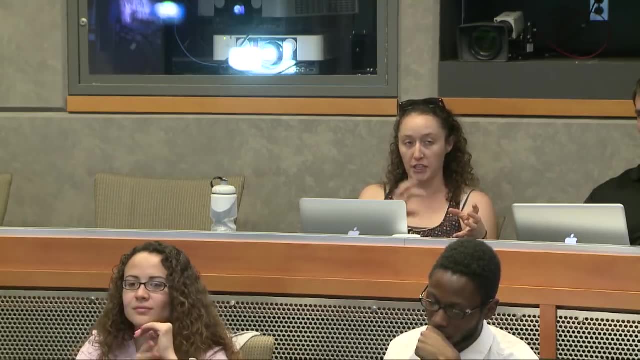 to the specification, Or they'd not understand how the two intersected. so I think there was a bit of a misunderstanding of the difference between what the actual requirements were versus what the specifications were designed to be. Okay, The sensors you're talking about would be sensors I'm assuming that you would purchase. 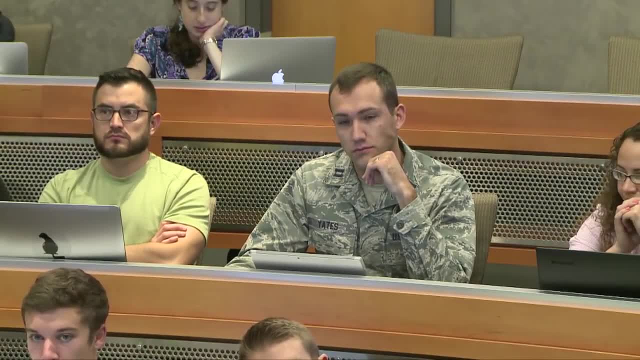 right, Mm-hmm As commercial? Yeah, absolutely So. I think we're buying off the shelf And so I mean sometimes the specifications were broader than what we wanted, sometimes they were narrower. But you know, you can do additional testing. 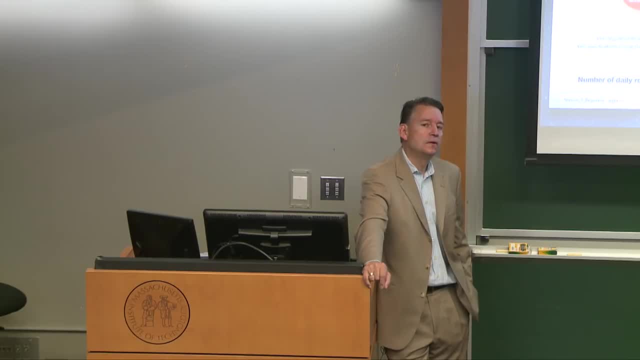 And so there was sometimes a breakdown between understanding really whether the sensor met what we were looking for or it didn't. Okay, Good, What about at EPFL? Any experiences? Volker, you worked on slip rings- right, Slip rings was one of the main things. 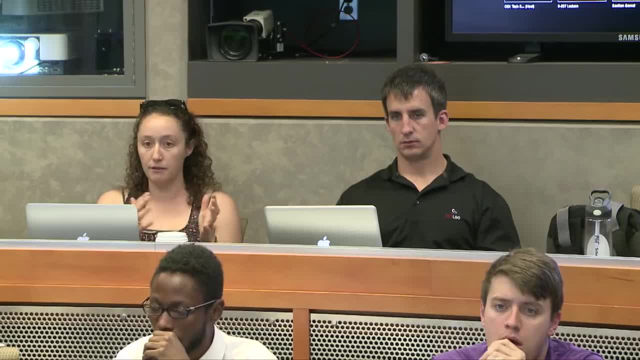 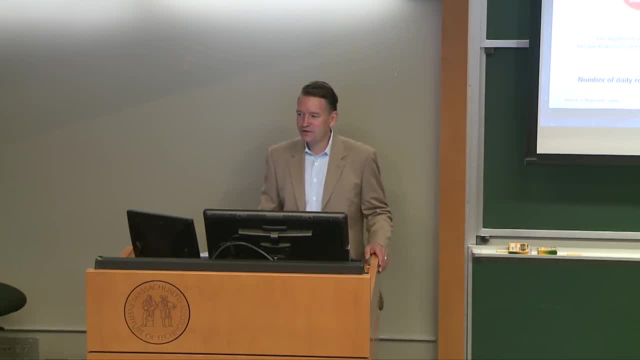 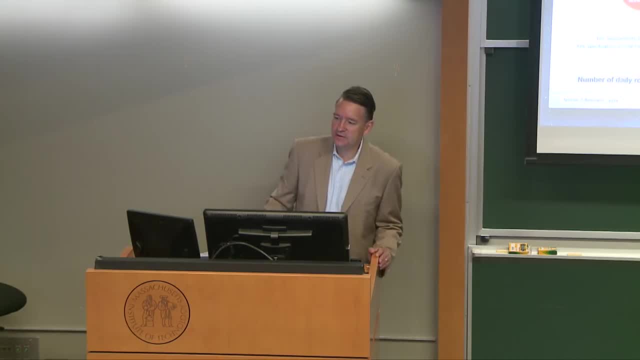 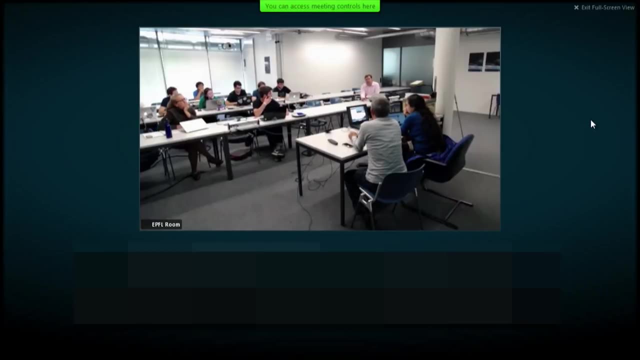 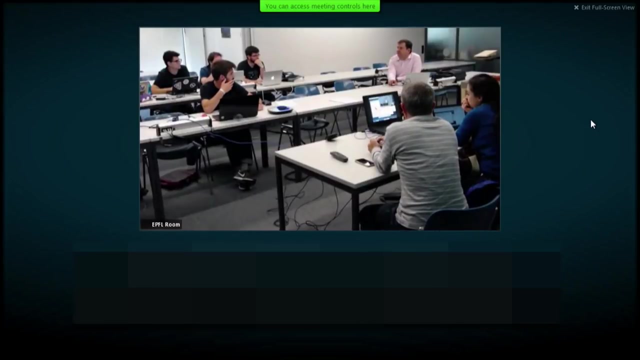 Between requirements and specifications. What are your thoughts at EPFL on this? Well, yes, on our side we clearly had a separation, also on an ESA level. But I was wondering here in the class, has anybody ever seen the difference between specification? 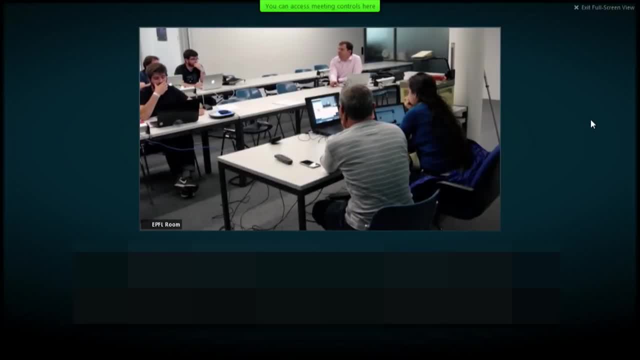 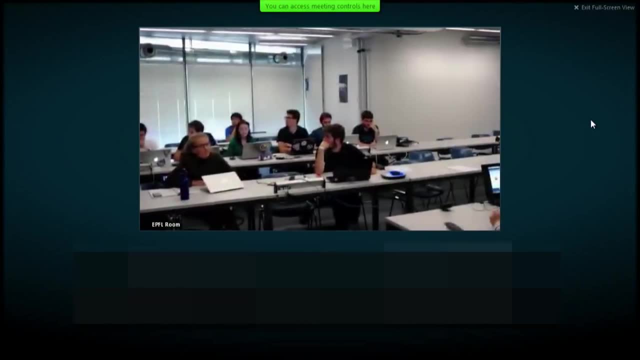 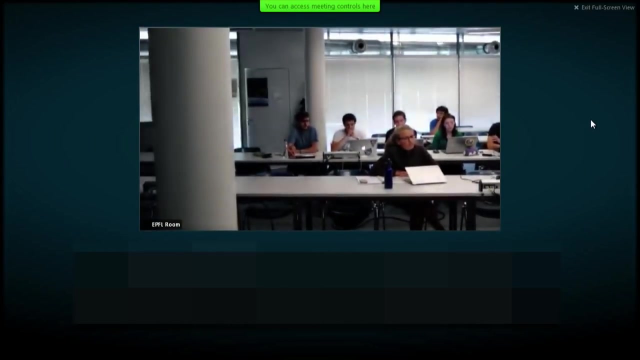 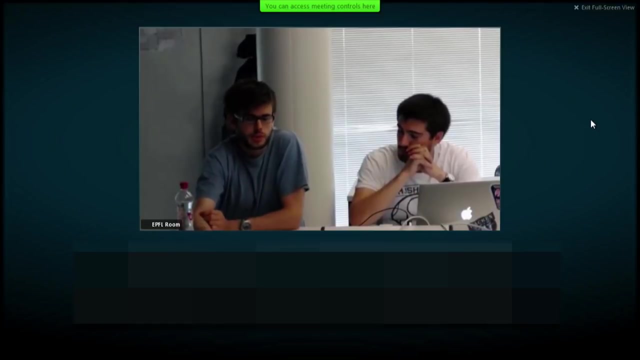 requirements. Any comments? Maybe some of the PhD students that have been around Any comments? Okay, the block is the time when we are just with a design. we work with requirements as an input, specific targets for functions of the nation, and well, we don't speak. haven't spoken yet so much about specifications, but I mean the 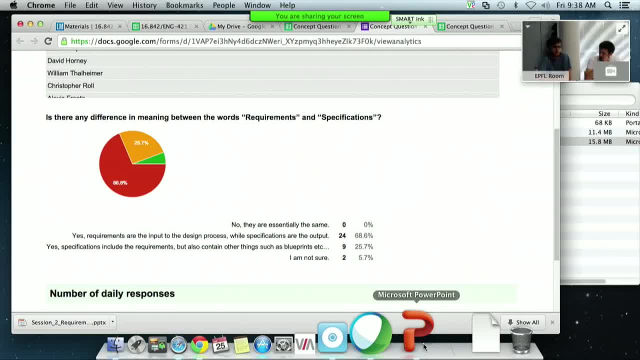 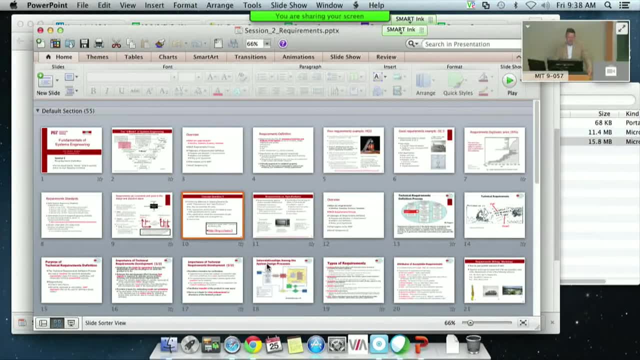 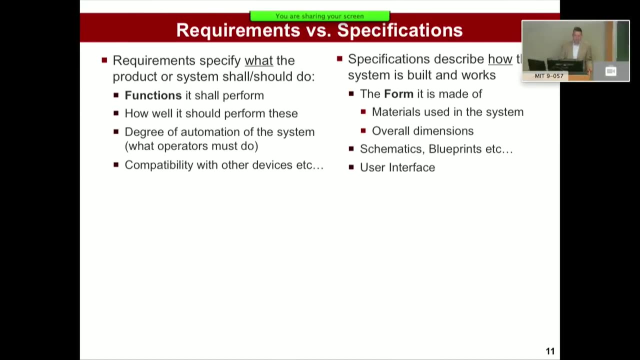 meaning comes somehow naturally. watch your system would be able to achieve: yeah, okay, great. so I found here I, you know, I I wanted to sort of find a real, an example that everybody can relate to very, very easily. so so the answer is there is a distinction. they are quite different, but they're got to be careful. 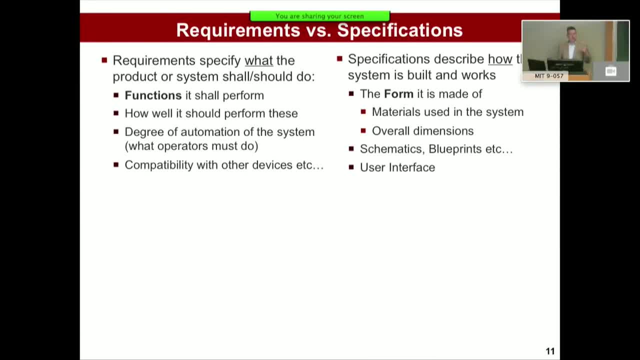 because people mix them up. so requirements specify what the product or system should, shall or should do: right functions that shall perform, how well it should perform. these also maybe the degree of autonomy- you know how automated is the system. so what? what the operators must do when the system is operating, and also 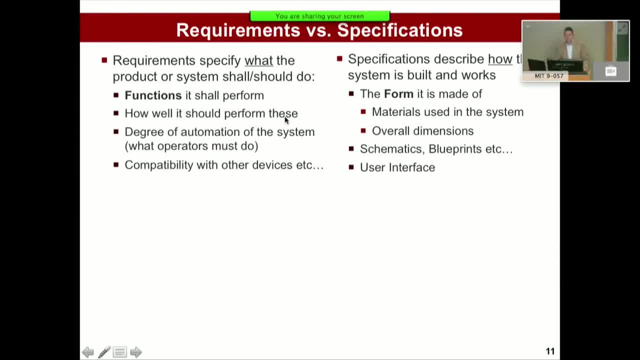 compatibility with other devices. and then specifications are about how, how the system is built and how it actually works. so the form right, what the materials that are used, the dimensions, schematics, blueprints, the details of the user interface, those are things, those are all specifications. so I I try to look up, you know, a very simple consumer product that 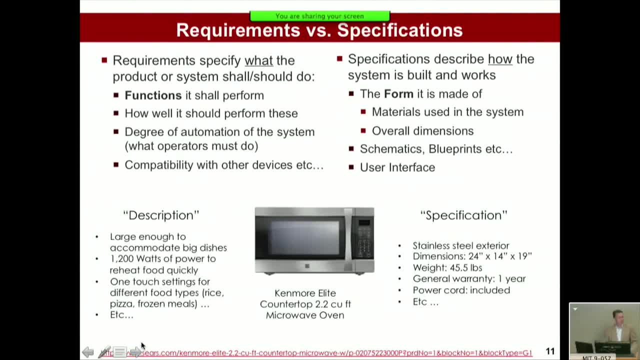 we all are familiar with microwave oven: Kenmore elite countertop, 2.2 cubic foot. you go to Sears website and what's interesting is they actually do a pretty good job. it's actually pretty consistent with what I'm saying here, except they don't talk about requirements. they call it description, right? so what's listed? 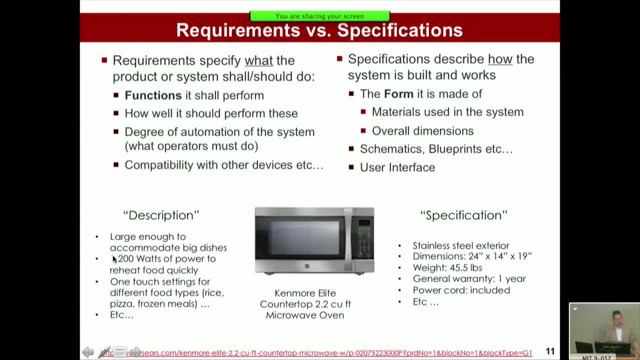 under description and this is- I'm pretty much quoting this here verbatim: this microwave is large enough to accommodate big dishes, right? so so the idea this is sort of family style, right? this is. this is not a small microwave. just for you know, frozen meals this is. you should be able to put a big casserole in it, and 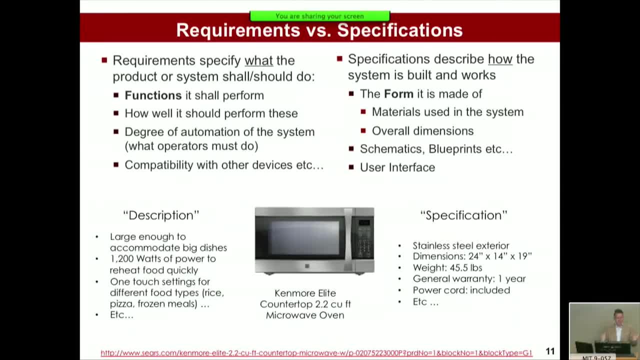 and reheat meals and so forth. so the idea that you know what, what are the things you're going to use in the microwave, what's the use case, right con ops, con ops for the microwave. you know family for kids. both parents are working busy. you know, not time to spend two. 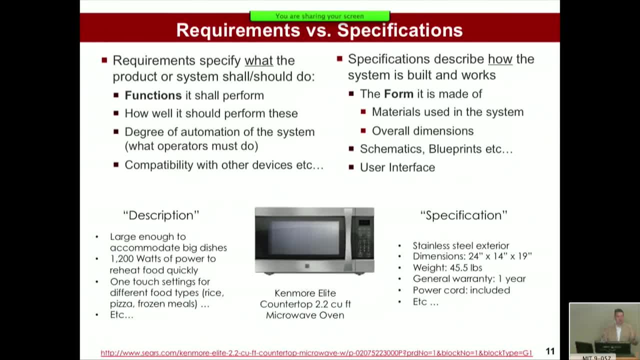 hours preparing dinner, therefore big dishes, a lot of people. it has to be quick, right, that's a, that's a con ops and and the requirements this description is essentially. the requirement is 500 watts of power to reheat food quickly. so time is important. and then 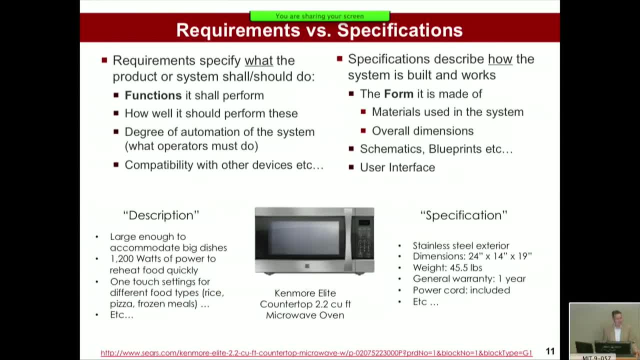 one-touch settings for different food types: rice, pizza, frozen meals and that. what is that? that's automation, right, rather than having to guess how long and at what power level to reheat. there's, there's some partial automation built in. that's. that's. that's essentially requirements. very user-centric, did you? 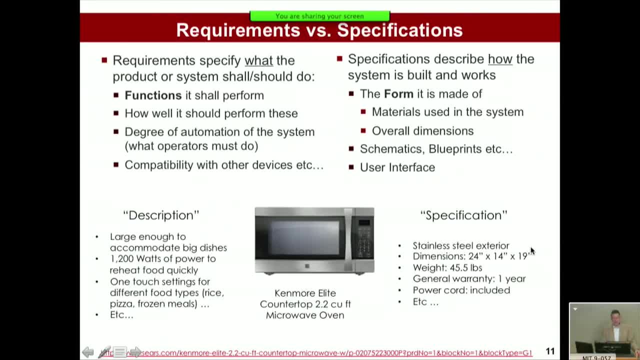 see that. and then when you look under specification, it says the following things: stainless steel exterior- right again, you don't want it to rust- the dimensions, the weight. there's a general warranty for one year. the power cord is included. you see, it's a very different. those are things that describe how it's made, in the form of it. 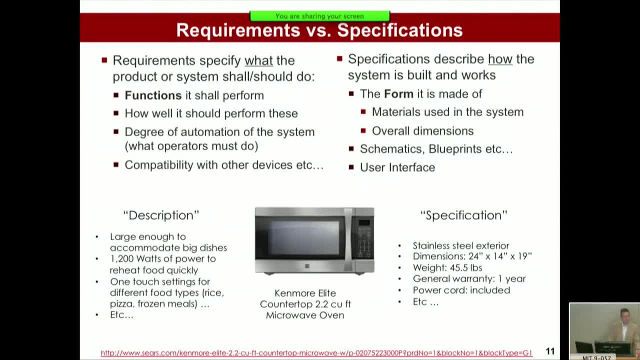 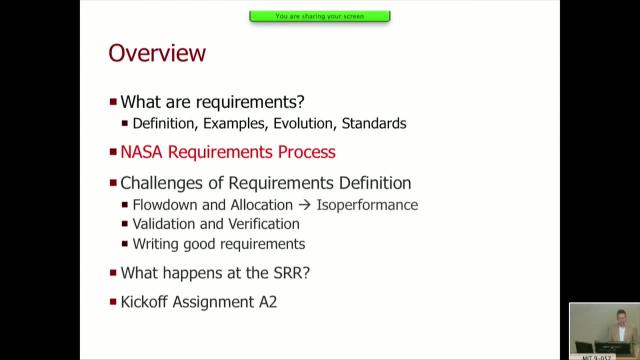 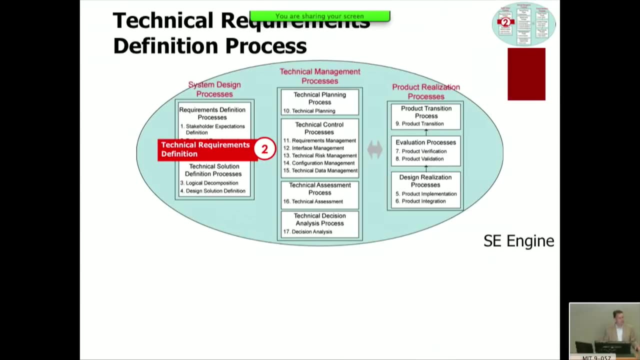 and so forth. so make sure you, you, you keep those separate, okay? so let me talk about the NASA requirements process and then we'll talk about challenges. so, getting back to the system engineering engine, that's that's sort of the heart of of the NASA system engineering process. you remember, this is the this: 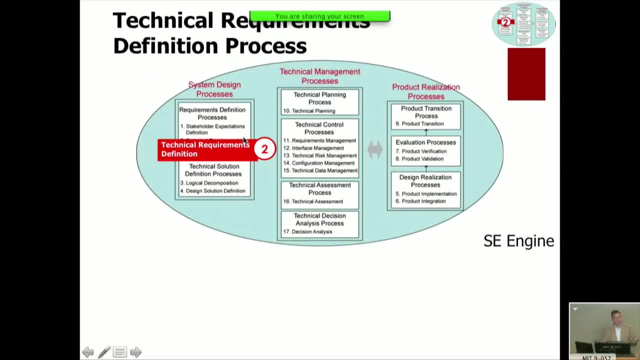 happens at every level of decomposition after stakeholder expectations. the second step is technical requirements definition, and there's some pretty strong language in the handbook that this really has to be done. well, so the center directors or their designees shall be able to do this. well, so the center directors or their designees shall. 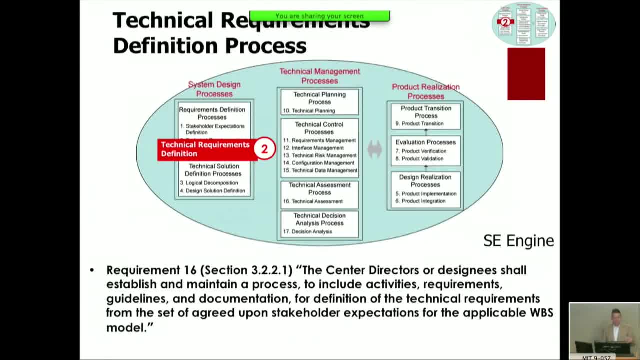 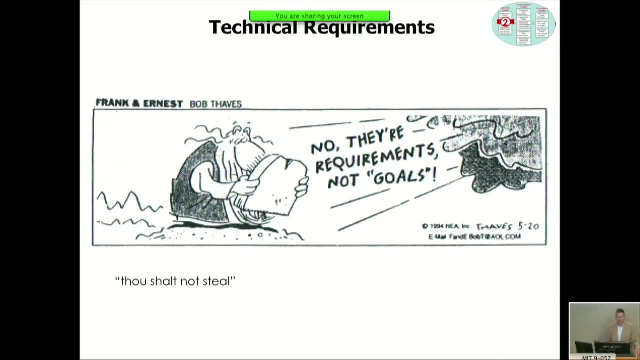 establish and maintain a process to include activities, requirements, guidelines, documentation for the definition of technical requirements. so I think I've already said this, but I just want to make it clear again. this is a kind of I like this cartoon. this is Moses right up on them. Moses just got the. 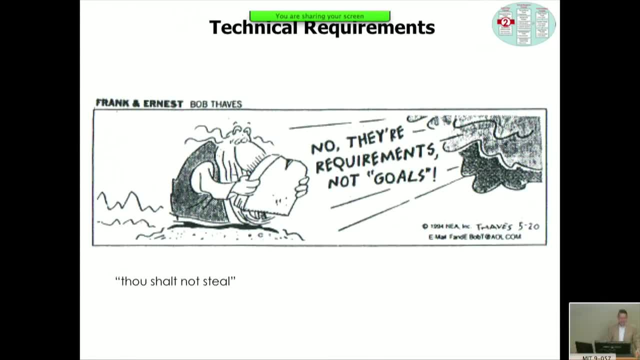 the tablets, right, the stone tablets. they, they tend Commandments, and one of them is: no shalt not steal. and god says out of the clouds, know their requirements, not goals, right, so what? what God is saying is that 10 Commandments are shall and and not sure, even though i think some of us don't always succeeded that, but that's. 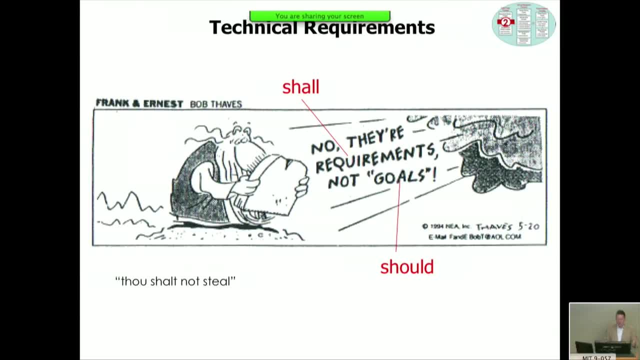 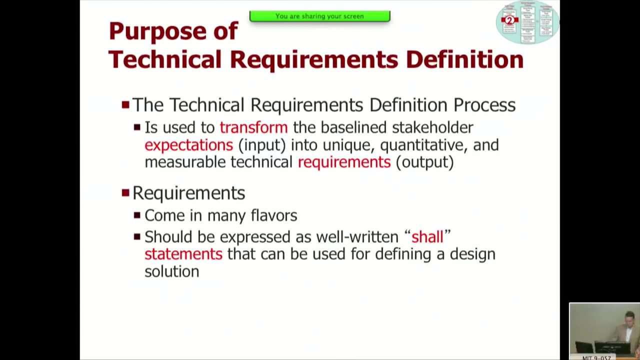 basically, the idea shall is very is a very hard constraint and that's what you will be judged against and should is essentially a desirable goal, but the degree of attainment is somewhat flexible. Why are we doing this? Why are we spending our time writing technical requirements? 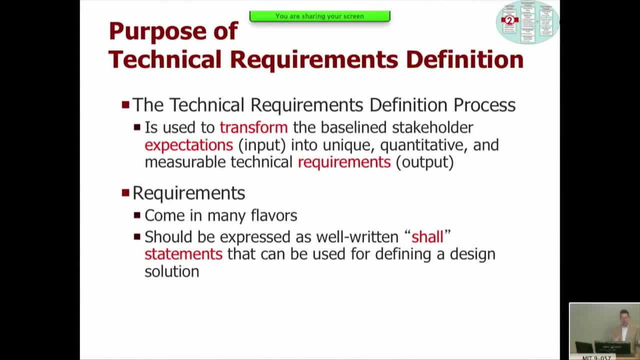 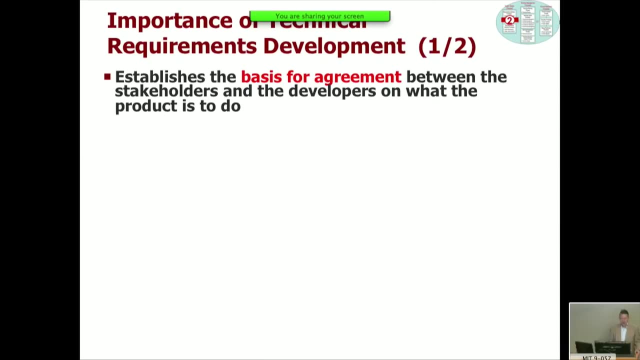 It's essentially to transform those stakeholder expectations we talked about last time, transform them into measurable technical requirements. Requirements come in different flavors and I'll mention those flavors, and we express them in these shell statements. They also provide a basis for agreement among the stakeholders and developers. so you will. 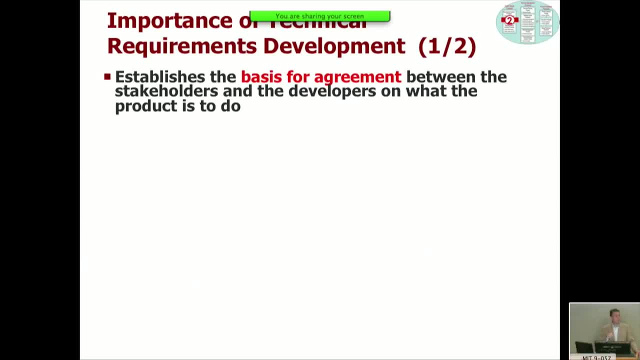 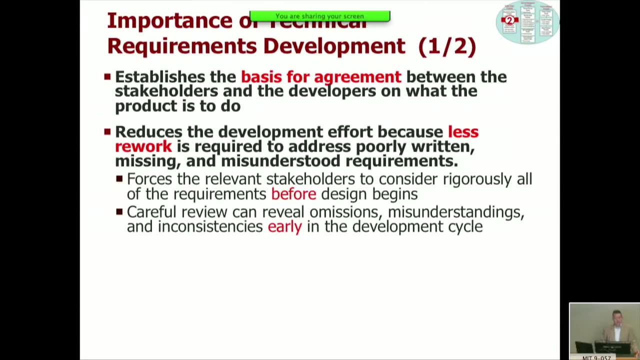 often find requirements part of contracts. right Now it becomes serious. you know, when the requirements set actually has legal implications. You're legally signing up to develop a system that will meet these requirements. That's pretty serious stuff. By writing good technical requirements, 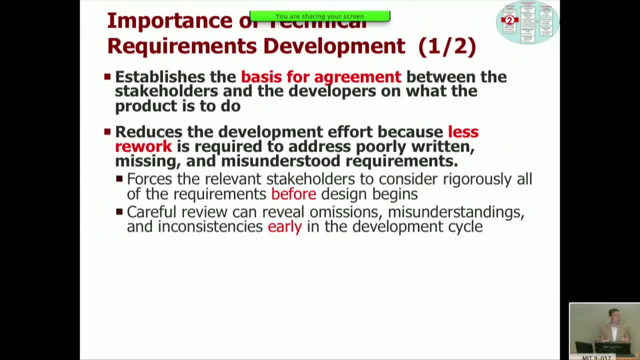 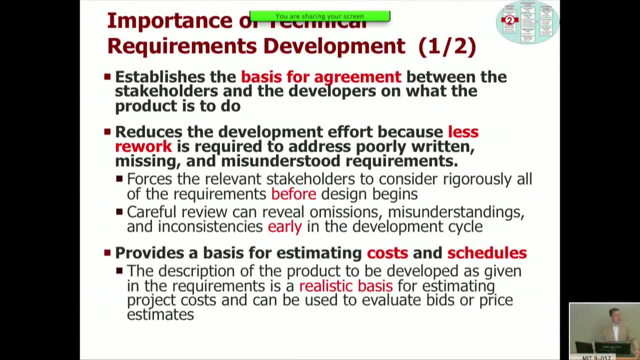 You can reduce the development effort because of less rework. so a lot of rework and iterations and confusion is based on missing or poorly written requirements right and writing those early and before the design begins is helpful. A requirement set is also a basis for cost and schedule estimates, and so some of these 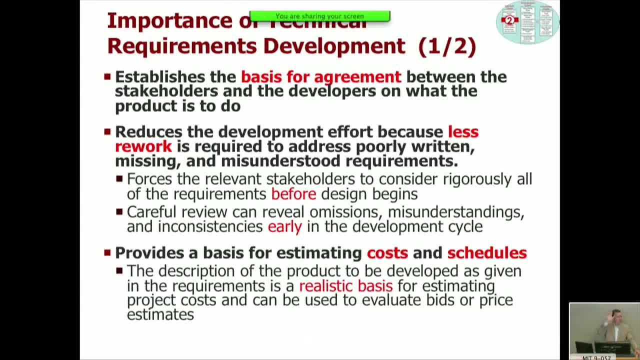 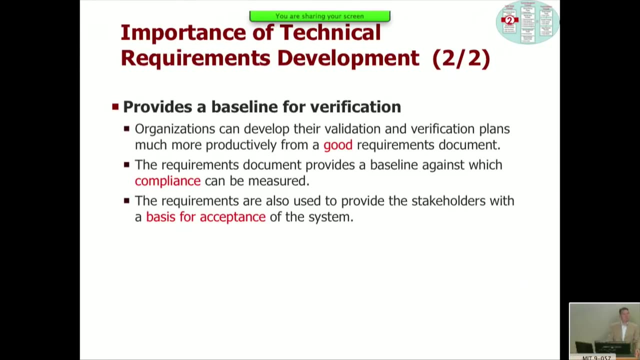 missions that overran. do you remember I showed you this chart last time. We analyzed 40 missions. We did a comparison of the success rate for the Marathon space science missions Like 20 percent of them were responsible for 80 percent of the overruns. 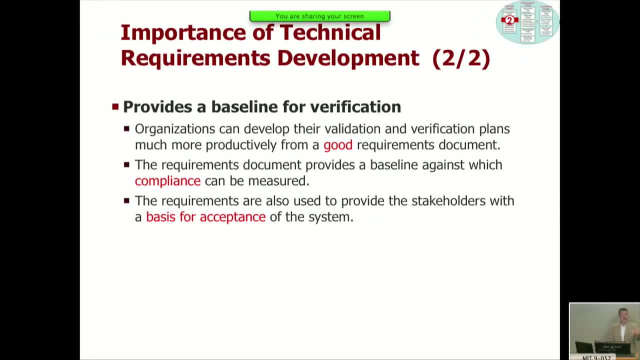 A lot of that had to do with unrealistic goals or expectations and requirements. And then the next point here is that the requirements provide the basis for verification. In other words, the better, the more crisp, the better written your requirements are, the easier it is to test the system. 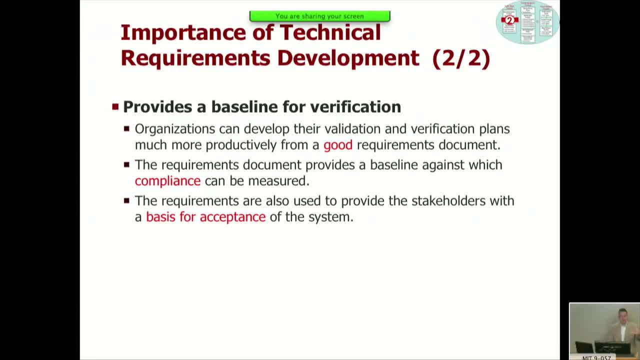 So that's a good example. So I'm going to stop there, Okay, Thank you, Great, Thank you. Bye-bye, Have a great day, Bye, Bye. and to check whether the system is in compliance with the requirements. 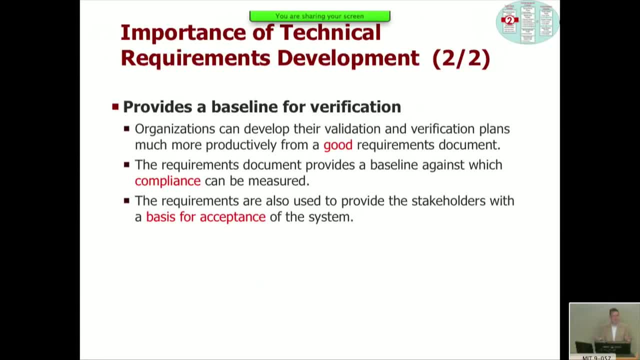 And then eventually the basis for acceptance. Acceptance is also a big deal, right? It basically means I accept your design, I take ownership of it and I say: you, as a developer of the system, have done your job properly And there's a legal transfer of the asset. that happens. 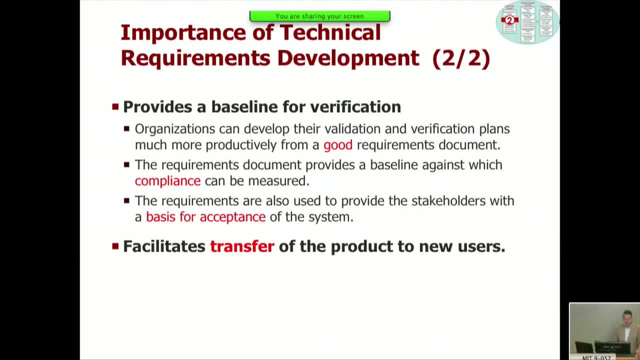 So it facilitates the transfer of the product to the users And then, even later, if you're going to do like a version two or a block upgrade, a next generation product, it's much easier to do when you have the clear requirements because it tells: 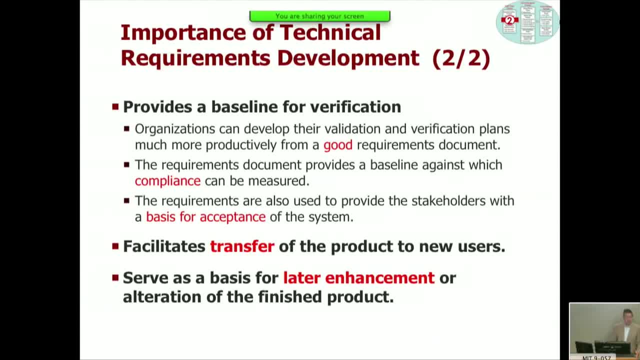 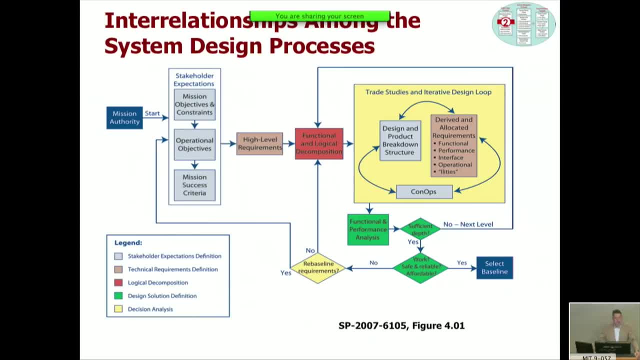 you what the original system or the earlier version was able to do or not do Graphically. so this is figure 4.0.1.. I briefly talked about this last time. We start essentially here at the development. We have mission authority. 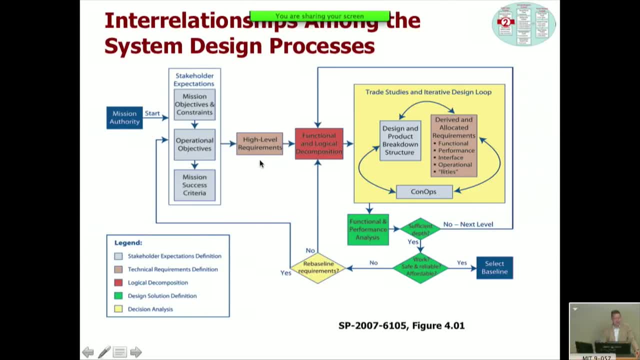 We do the stakeholders, We do the stakeholders, We do the expectations. Talked about that last time. And then here right away, comes high level requirements. So that means your level zero, level one requirements, And then, as you try to get more detailed in the requirements, 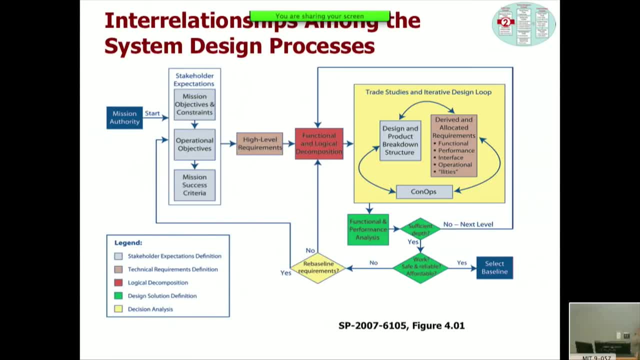 what do you think happens? Let's say you ideally want to write all the requirements up front. right, That would be great. But you try to do that. you hit a wall. Why is that? What's the issue? Why can't we just write all the requirements? 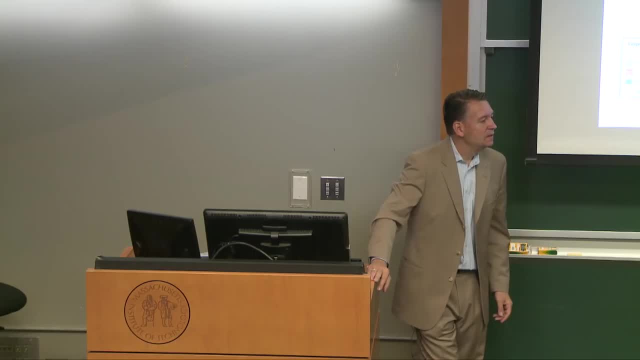 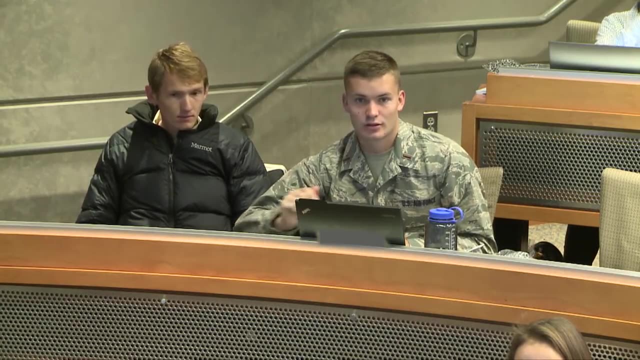 and then be done with it in one shot. Yes, go ahead. Your system changes over time And some of the requirements clash And you can't achieve all of them simultaneously. Yes, so there's two things you mentioned. So one is the sort of, and I'll talk. 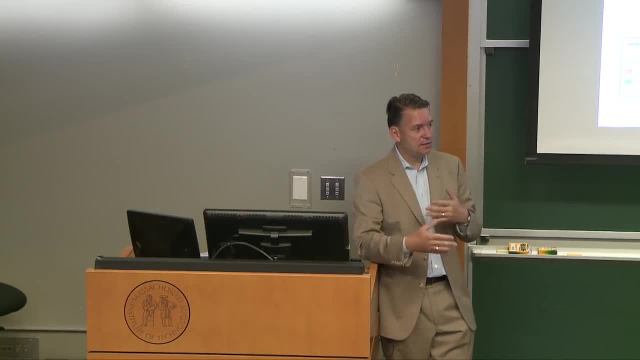 this is known as requirements volatility right. The requirements are changing as you learn more about the problem. And then the other is: you detect conflicts between requirements And you have to clean those up. OK, So those are two very valid issues, But it's not quite what I was going for. 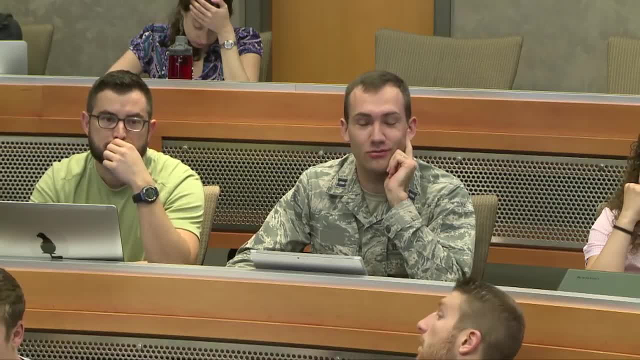 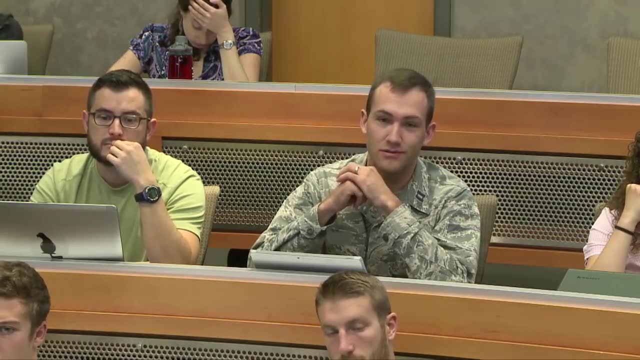 There's another one: requirements creep, in which your customer levies new requirements on you once you've started the process. Yes, so new requirements get added. Hopefully you get more budget too. That doesn't always happen, right, So that's another issue. 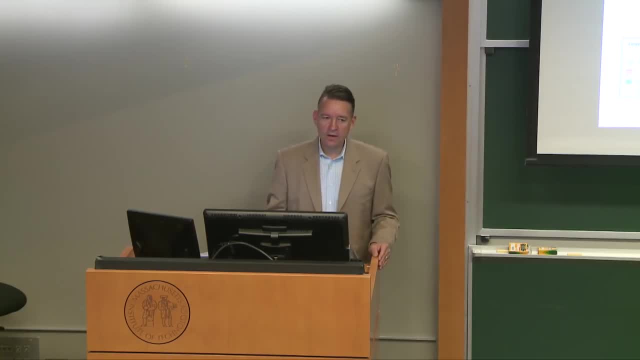 But it's a little different. Let's say, at EPFL, you guys, why don't we write all four or five levels of requirements all at once? Why can't we do that typically? What do you think? Usually, some of the requirements aren't clear. 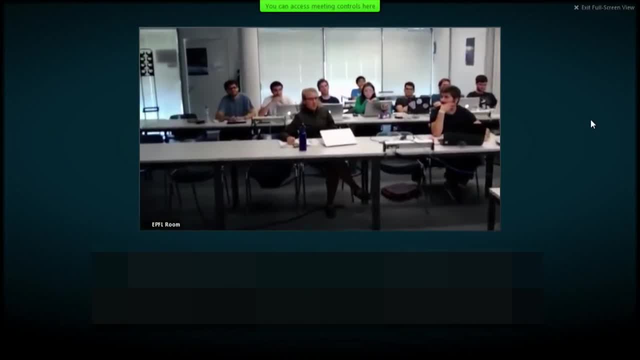 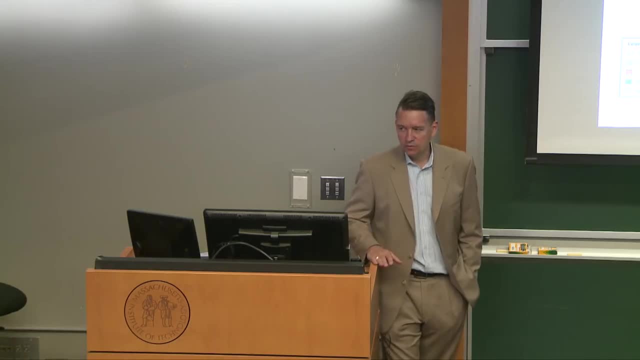 They don't exist yet. Later on in the process they become clear And you start to realize the details, which I personally don't. Yeah, I think that's pretty close to what I'm looking for. So the issue is: you do your level 0, level 1 requirements? 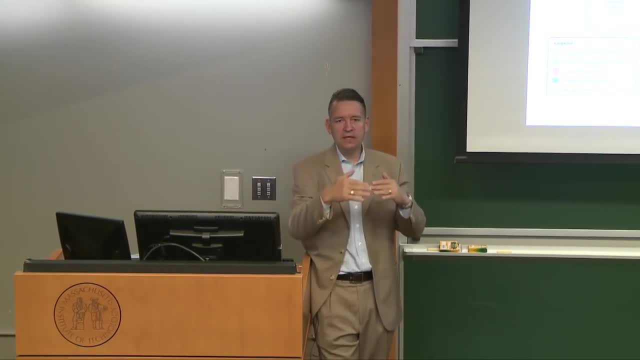 And then, sort of as you get to level 2, you can't really write a level 2 requirement, You can't really write a level 3 requirement until you've made some key design decisions. Are we going to use electric propulsion Or are we going to use chemical propulsion? 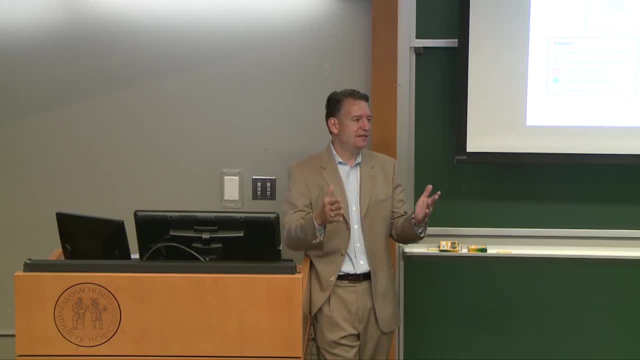 That's a huge decision in space system design And unless you've made that decision, you can't really write lower level requirements, Because the fundamental working principles of chemical and electrical propulsion are quite different. So that's the key issue Is that 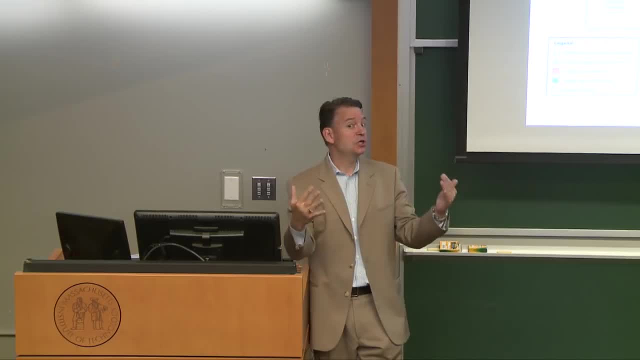 You can only do. You can only do in a solution-neutral space. And then you hit the wall because you've got to make some key concept technology selection decisions And that's shown here by this red box called functional and logical decomposition. I don't like that nomenclature a lot. 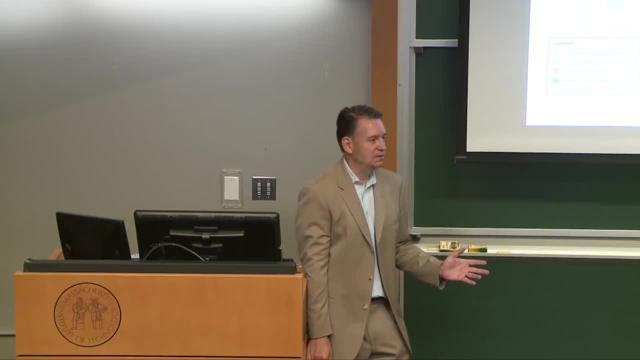 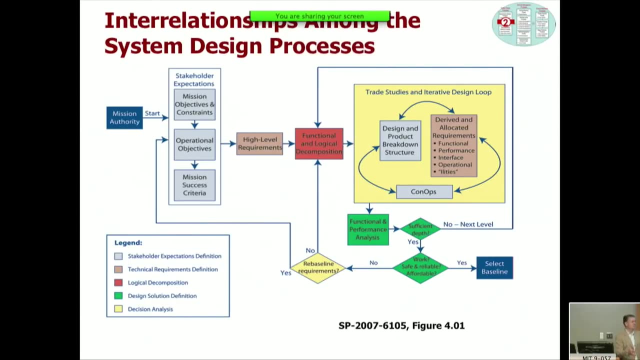 This should really say system architecture or concept selection, which we'll get into in the next couple of weeks. Once you've chosen a high level architecture and concept, then you say, OK, we're going to go for ion propulsion. Well then you can write the requirements for the ion. 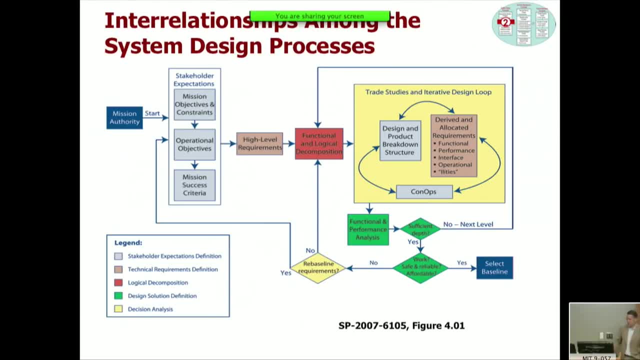 propulsion system, which are defined in this yellow box here. So this is your design and product structure, derived and allocated requirements at lower levels. You see that That's the fundamental. All the things you said: requirements, creep, requirements, conflicts. All those things you said. 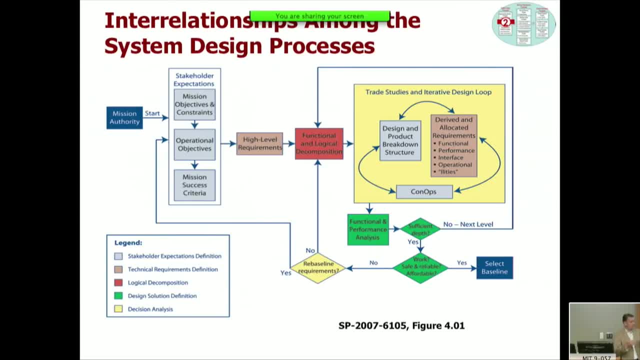 Requirements creep, Requirements conflict, Requirements conflict. All those things are true, but the fundamental reason why we can't write all the requirements up front is because at some point the lower level requirements depend on design decisions you make. That's the fundamental issue. 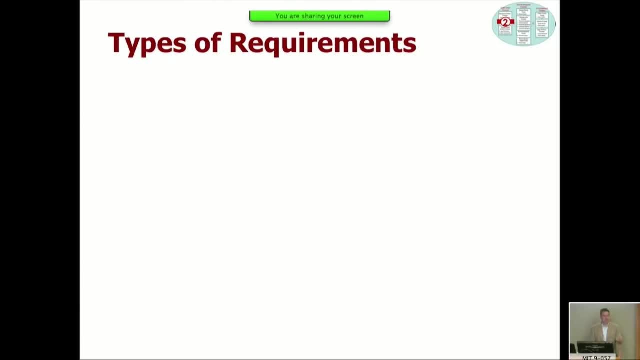 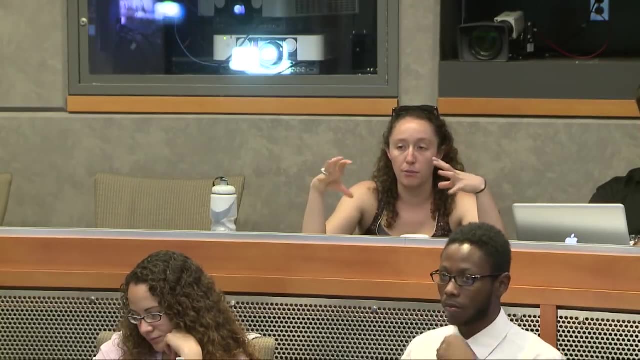 OK, Any questions about that point? Yes, It's not totally about that point. So, requirements versus specifications. So if you're buying a component from a vendor, some piece of hardware, and you want to identify, like the specific locations where, 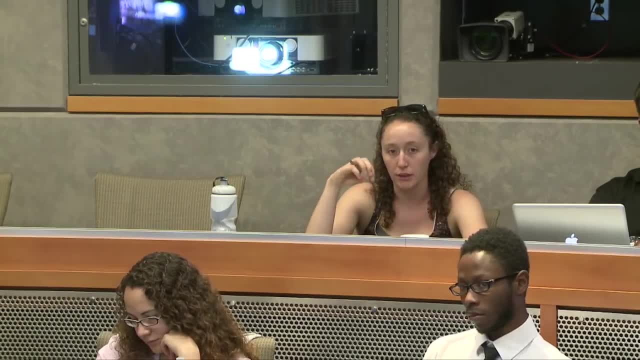 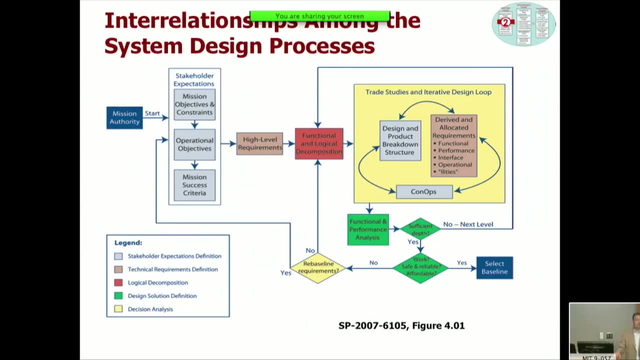 it should attach to things. it's more of like a form as opposed to really, so does that fall into requirements Or is that like a specification? Great point. So there are. what you're describing is a particular type of requirements that we call interface requirements. 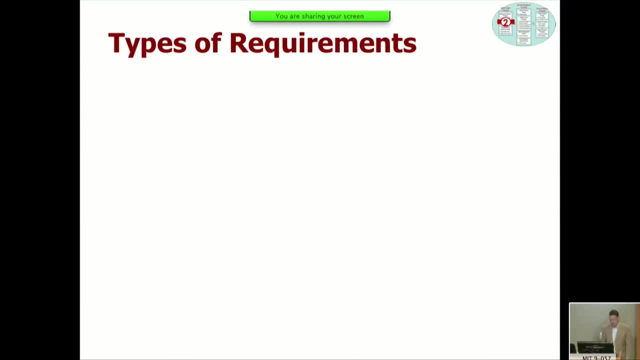 And it's a perfect segue to this. next, you know, if I could only include- like I don't know, five slides in this lecture, this would be one of them. This, basically, is: what are the different flavors of requirements or types of requirements? 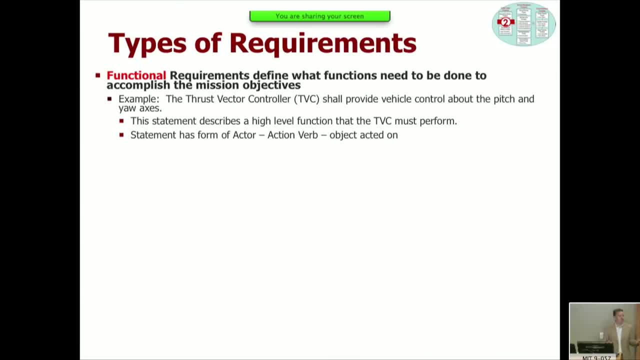 And there's six of them here. So first of all, the functional requirements- I think we've sort of talked about those right Define the functions that need to be done to accomplish the mission objectives. There's some examples here around thrust vector control. 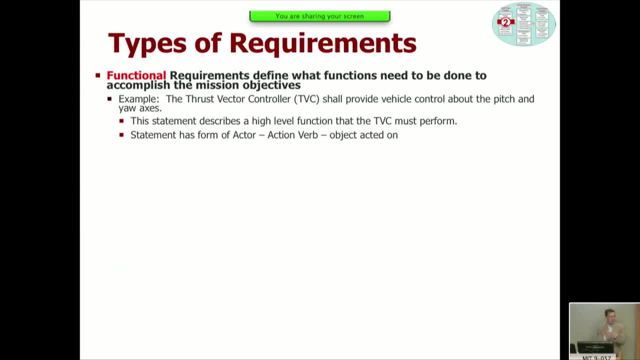 So basically, the idea here is that you have a thrusting system and it has- you can actually direct the thrust And in this case you should control the thrust. You shall provide thrust control around pitch and yaw axes. OK, So this statement is a high-level functional. 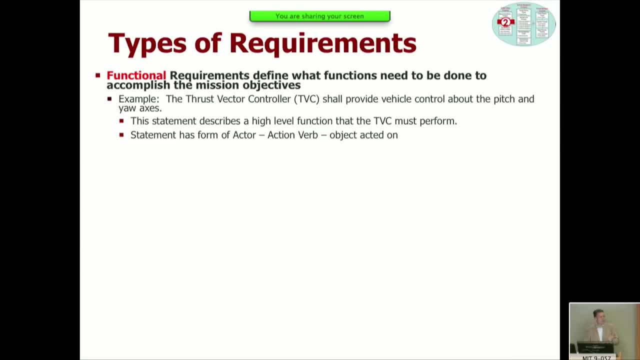 statement and it's written in the actor-verb-object form, right? So that's sort of the classic, you know, the classic requirement of a functional requirement. And then we have performance requirements. The performance requirements are in a sense qualifiers. 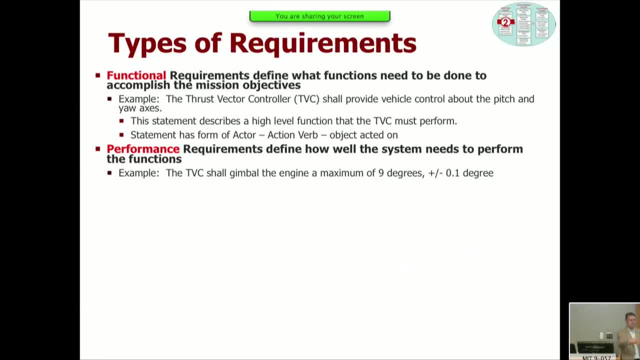 on the functional requirements. So a performance requirement will specify how well the function should be performed, How fast should it fly, How much thrust You know? this is where you have to actually put numbers in. So in this case, this thrust vector controller. 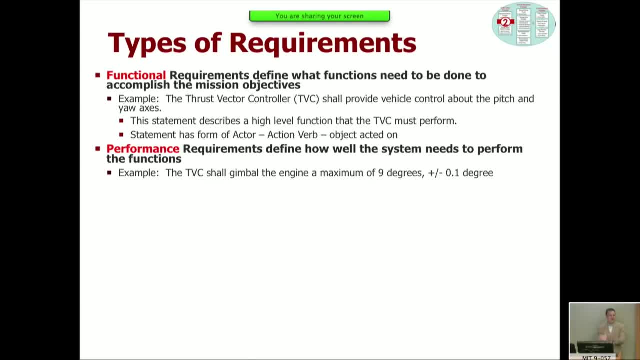 shall gimbal the engine nine degrees- right, That's the deflection angle. at least nine degrees, plus or minus 1 degree, 0.1 degree. That's a performance requirement. Then we have constraints. OK Yeah, Isn't the performance requirement, I guess, the most important thing? 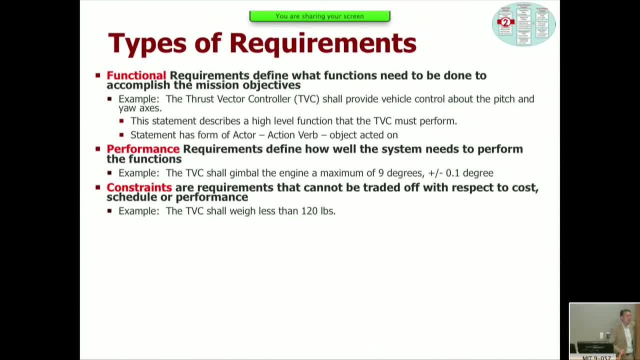 Yeah, Is the performance requirement saying the engine has to gimbal nine degrees? Isn't that kind of pushing towards the specification, Or is that? I mean, I guess it can also be a requirement, but isn't that Right? In this case we haven't said, we're not specifying how. 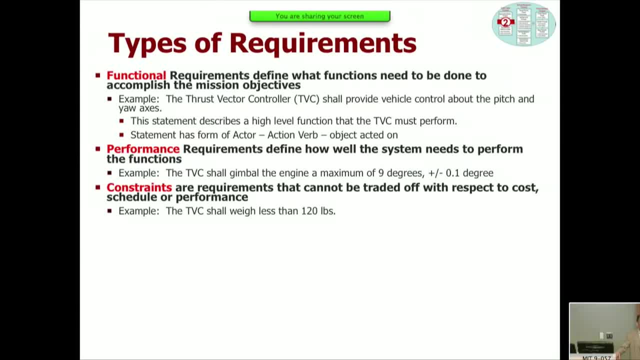 those nine degrees are achieved, whether it's through a gimbal or you know. the actual mechanism or how is not described here. All that's described is the angular range, essentially, And that is a performance requirement. But you'll see, there'll be some examples of things that are putting limits on the form. 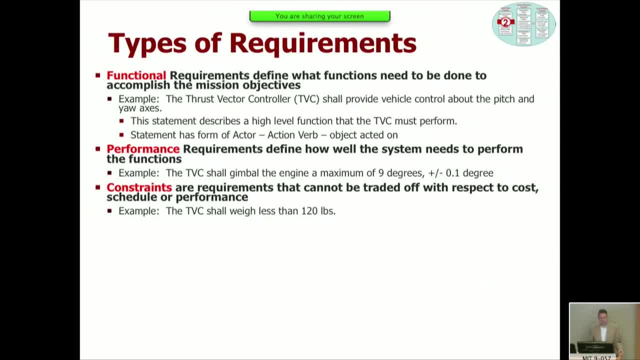 which looks more like a specification. So then we have constraints. Constraints are things on, like you know: weight, mass, power, things like that. So constraints are requirements that cannot be traded off with respect to cost, schedule or performance. 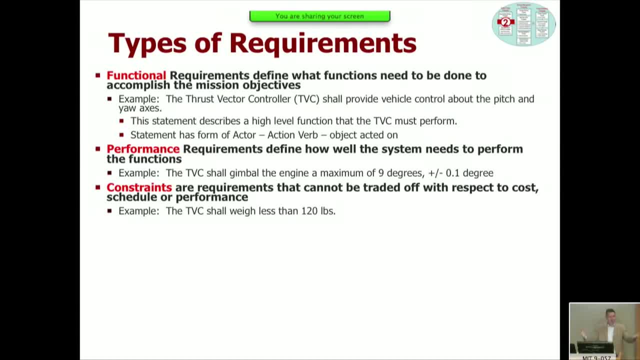 So, for example, the thrust vector controller unit module and the engine, and you know the module shall weigh less than 120 pounds. So that's a, that's not. if you think about it, that is not functional, right. 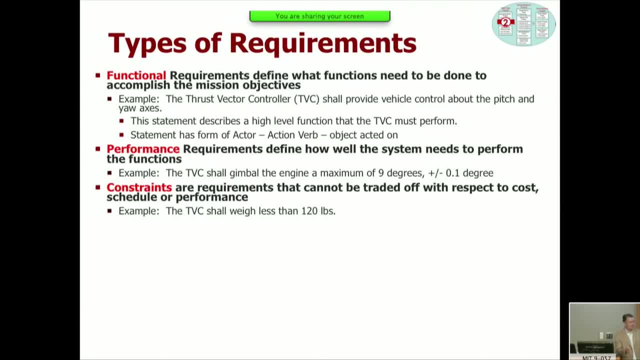 The weight of this thrust vector controller shall not be more than 100.. That is not performance, It's not functional requirement, but it's a constraint on the form essentially right. So this looks more like what we would call a specification constraint. 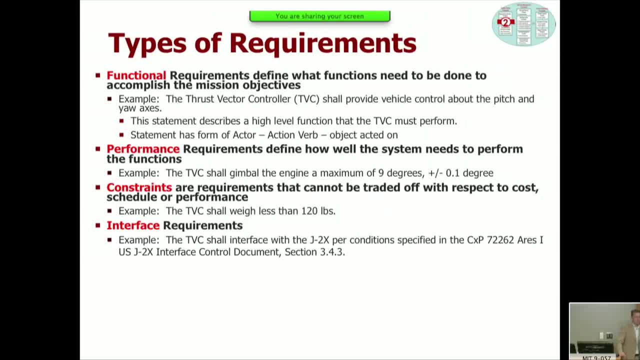 The fourth one is what Marisa brought up. This is an interface requirement. okay, So our, in this case our, thrust vector controller shall interface with the J2X. This, the J2, is a very famous engine and J2X is a kind of this is sort of this was. 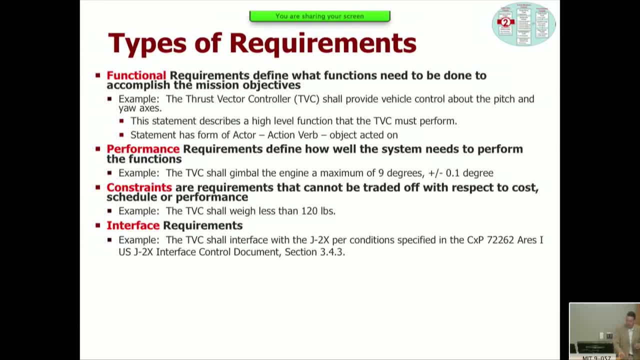 written during the constellation days of the constellation program at NASA is the idea of a new generation of the J2 engine. So the idea is that, whatever you do, however you design your thrust vector controller, your thrust vector controller, it must be able to interface with the J2X engine according. 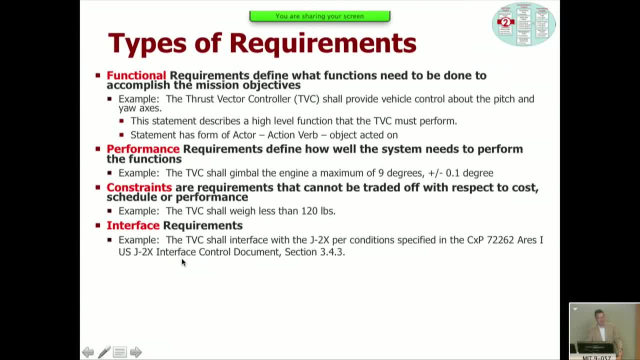 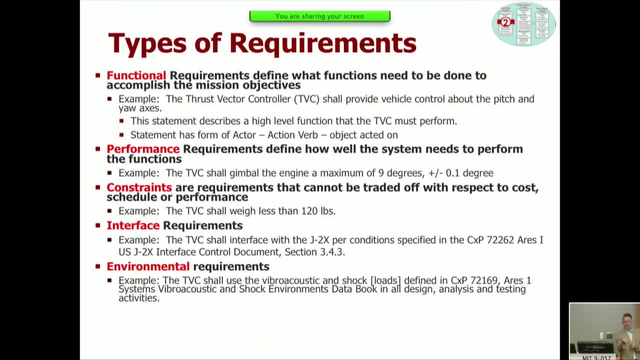 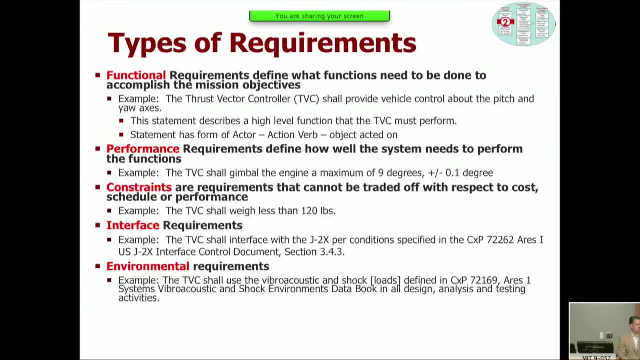 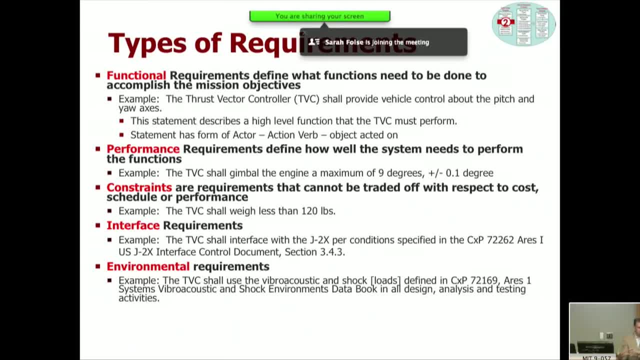 designing airplanes, you know whether you're flying in a small mountainous country like Switzerland or on the ocean off of an aircraft carrier. those are very, very different environments and they're going to influence. you have to specify the operating requirement. the bigger the envelope that you make for the 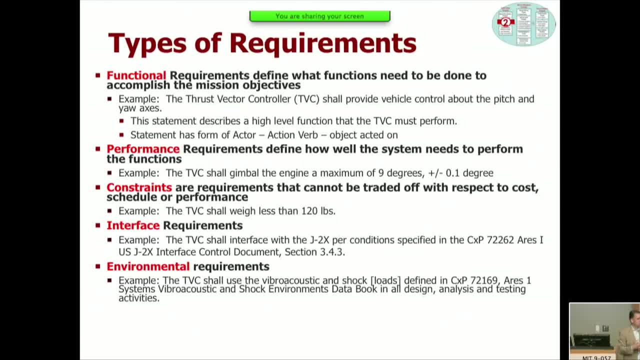 environmental requirements, the more complex the system will be also medical. anybody working on medical devices here, EPFL, anybody medical devices, so in medical devices, it's the same thing. you know our. is this medical device going to be used in a hospital setting, I know, where everything is kind of clean you? 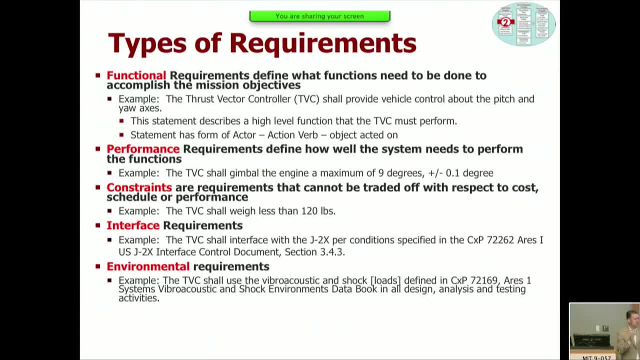 have clean power, the nurses, everybody is very well trained. that's one thing. or this medical device going to be used in the field. you know, Africa, in India, in a rural area where people are not, maybe not trained medically, professionally and so forth, very different. the function may be the same, but the environmental 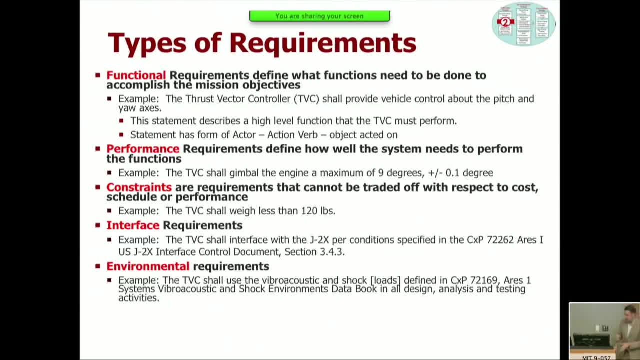 conditions are very different. you have to really specify those. and then we have, you know, the last category is kind of other, it's sort of a catch-all, but it this can be very important. so this includes a lot of the human factors, reliability and safety requirements. those are and, and you know, 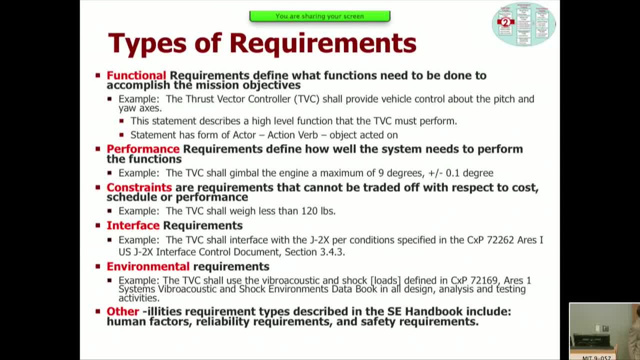 they're listed here as other, and I think it's really important to say that just because they're listed here doesn't mean they're less important. these are often neglected, unfortunately, and it really can hurt you in the long term. so pay attention to those human factors, reliability and safety requirements. so 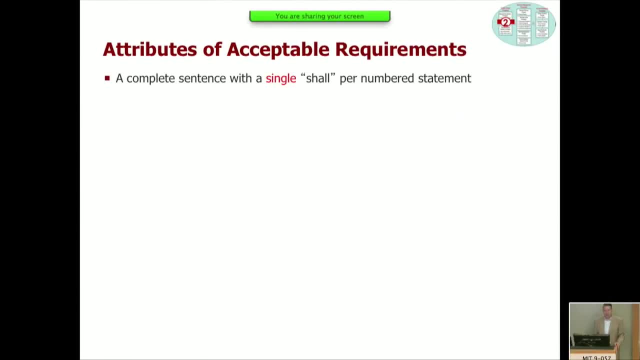 six types of requirements. so let's let's talk about what makes you know good or acceptable requirements, and there's a distinction here between a single requirement statement and then sets of requirements. so a first of all, requirements should be written in natural language. they should be complete. 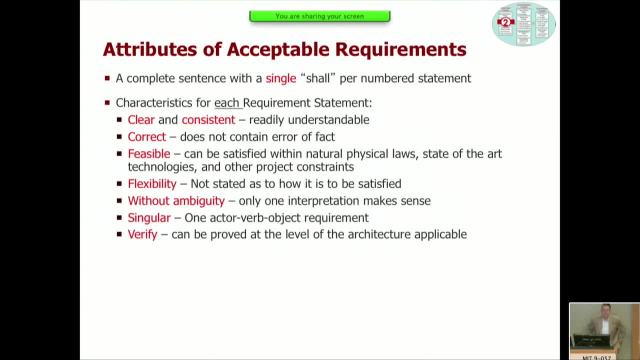 sentences and each of the requirements statements should be clear and consistent, meaning that you know it. it's not. it's not a novel or it's not a poem, but but it's clear, it's understandable, it's well-written, it's correct, there's no errors in it, it's feasible. now, that's a really tricky one, that's that's that's. 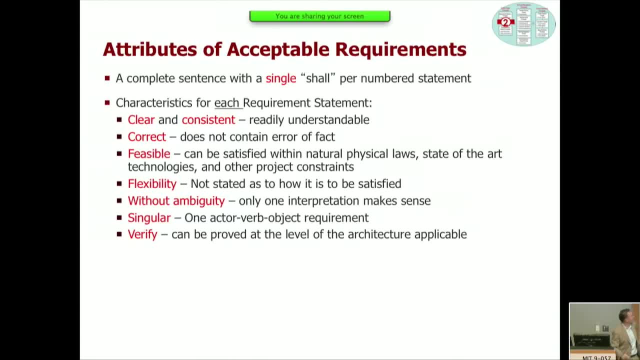 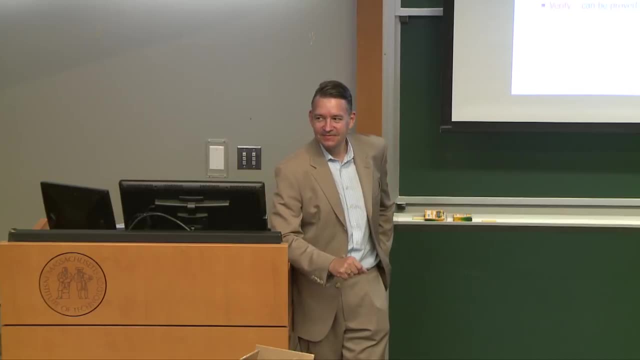 the first thing here. that's really tricky when you think about it. feasible means what it means. this requirement can be satisfied within, you know, the laws of physics and state-of-the-art technologies and other project constraints. so why? why is that a tricky one? go ahead. I was gonna mainly ask a question regarding that, in terms of how? 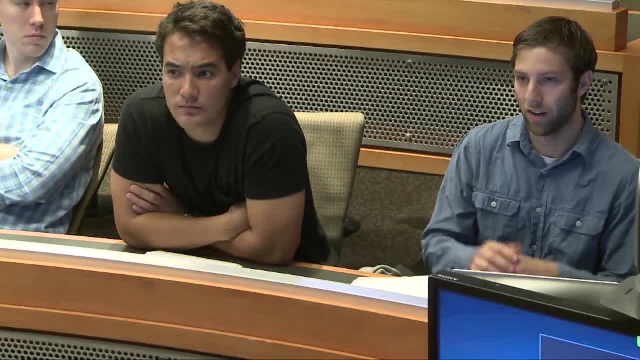 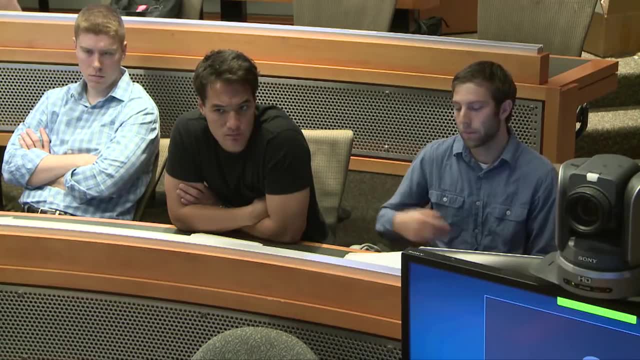 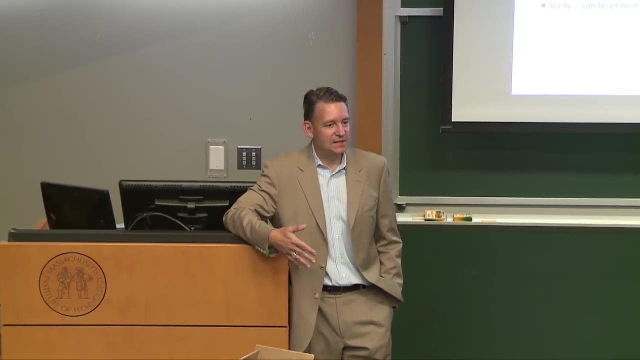 do you deal with a program where you're working on things, where you're trying to actually, you know, maybe define the state-of-the-art or figure out what is feasible, right? so if you're basically designing a product or a project or a system that's a repeat of what's already been done, then you can have pretty good. 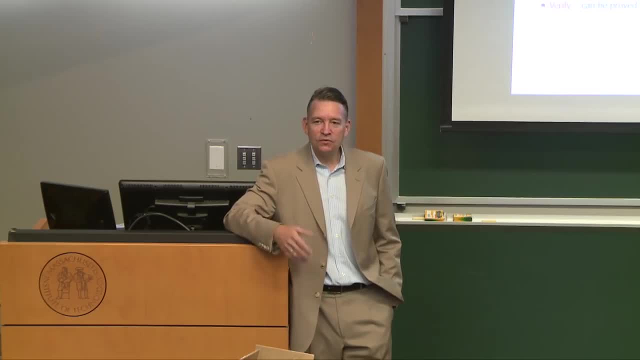 confidence right, that those, those are feasible. but what if you're you doing? you know the- let's say the- I think I mentioned this last time. you're going to Europa and you're going to drill through the ice and you're going to explore the ocean under the ice sheet in Europa. it's never been done before, you know, can we? 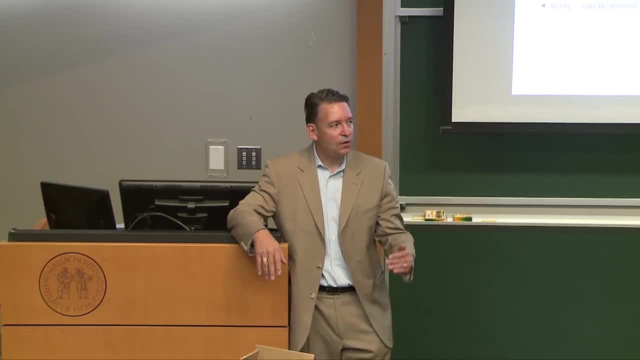 actually do this. so this is the tricky thing: how ambitious, how ambitious can the requirements be and you still can claim feasibility? and that that's also one of the big reasons why programs get in trouble is when, when they're actually defining requirements that are not really feasible within. 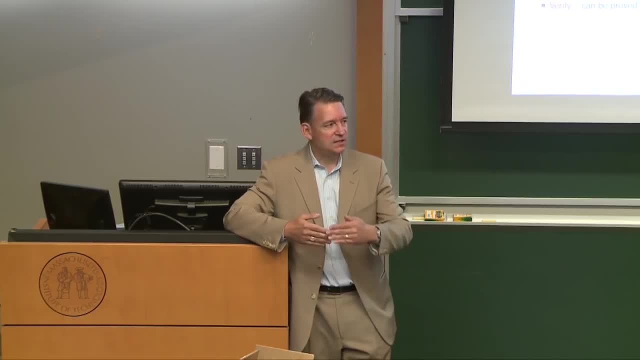 they're definitely way beyond the state-of-the-art and within the time frame and budget allocated. you can't get there and many, many programs that run into this problem are the ones where the technologies that you're going to use are not really ready yet. you know there will talk later about technology readiness level scale. you're 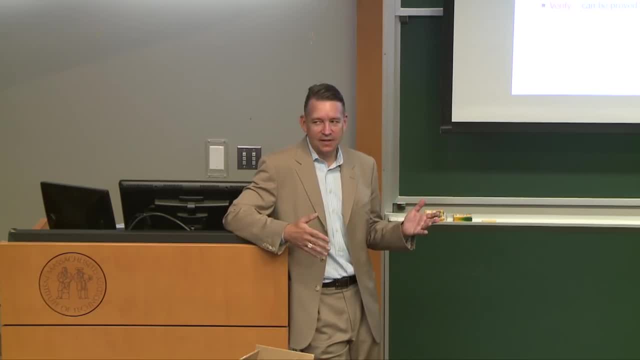 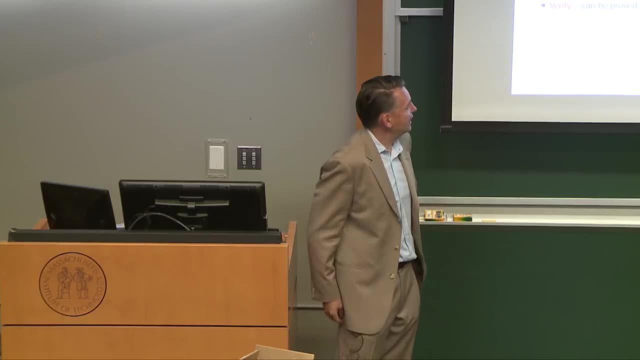 not really ready yet to do this, but you're going to try anyway. so that's a tricky one. feasibility, flexibility is, is you know. don't over specify how things should be done, so don't state how it should be satisfied without ambiguity. that means you know it. 10 people read this requirement. they should have the same, or? 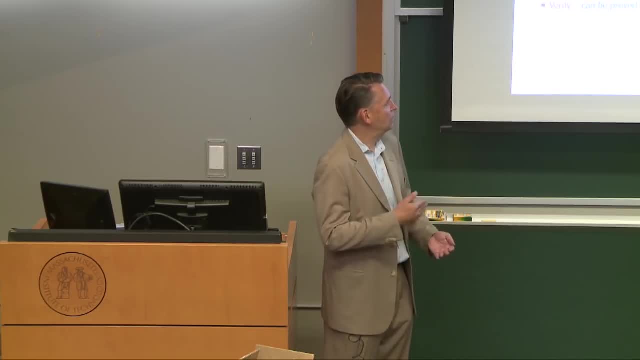 very similar interpretation: a singular statement, one-actor, verb, object. and then the last point here is verifiability. how are you going to check whether or not this requirement is in fact satisfied with regard to the, the feasibility again for some of these programs I had, you know? 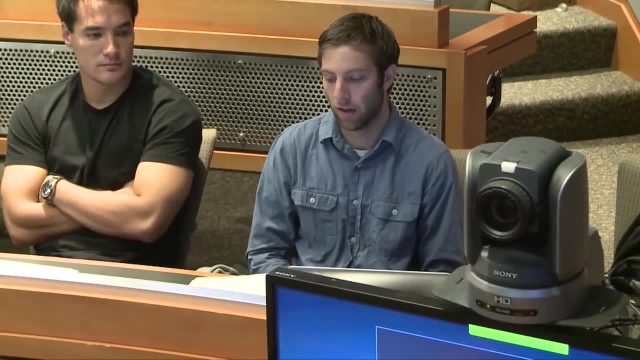 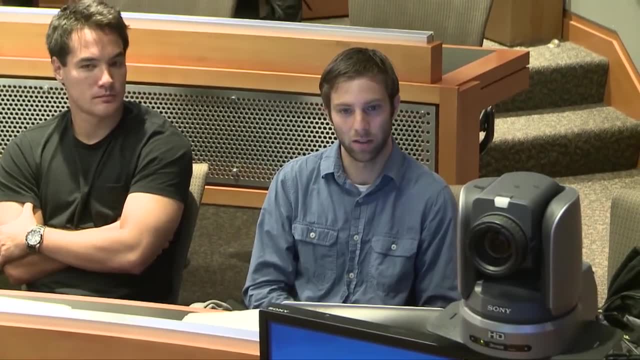 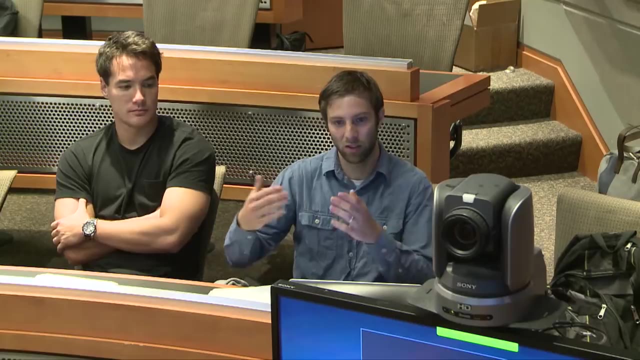 large. you know overruns, you know schedule overruns. I mean, would it be almost better, in a sense, to have some of the requirements be almost shells like oh gosh goals. in other words, you know if you can do, you know this, go for it. but if you're. 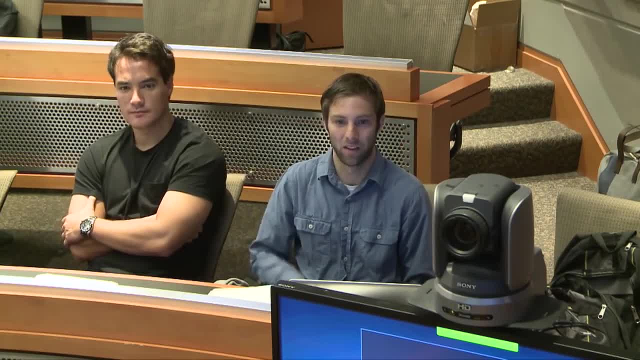 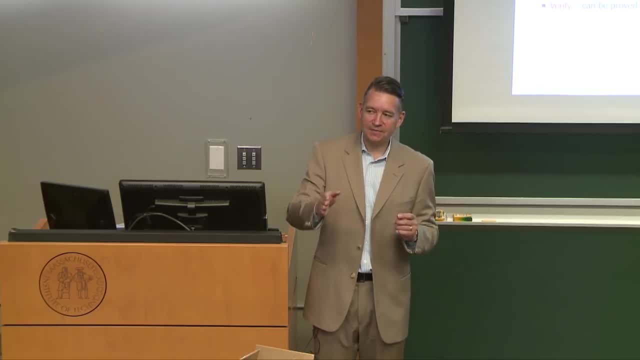 going to run over 10 years. maybe you'll back off a couple percent, that's right and what? we'll talk about this a little bit. but if you, if you, if all of them are shell statement, they're all heart constraints. the objective space you know, that I showed you may in fact have zero feasible space, right? so really knowing, 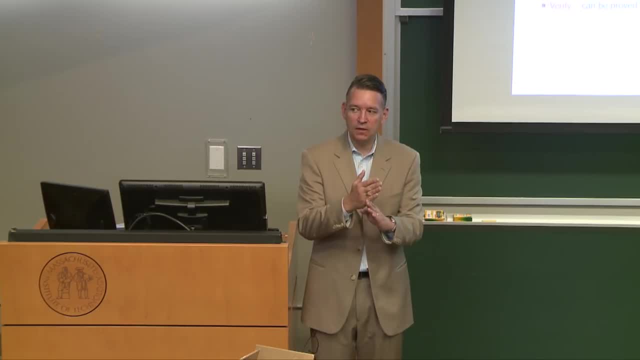 where, what? what is the heart constraint? what is a heart requirement and what's flexible? that's that's very tricky and that's that's why that's why it's important to actually not just accept requirements. you know, if you're going to run a project, every requirement, you want to really understand it and if you think 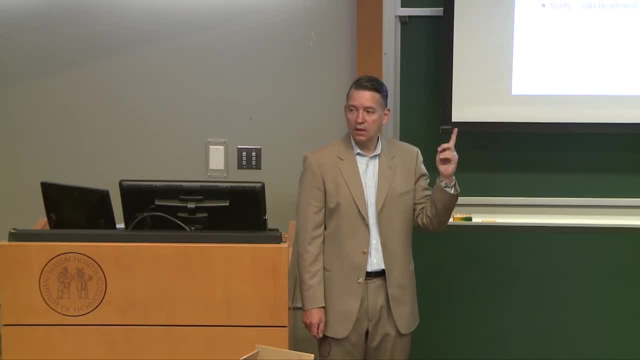 this requirement is infeasible. you have to negotiate. that's where the upfront negotiation becomes really important. did we lose our EPFL? okay, go ahead please. all right, whatever, I would have a comment here. maybe please go for it. so in 1990 we got the requirements from NASA to build a space bioreactor. 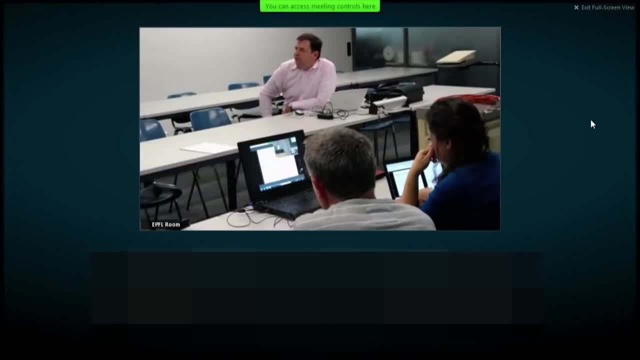 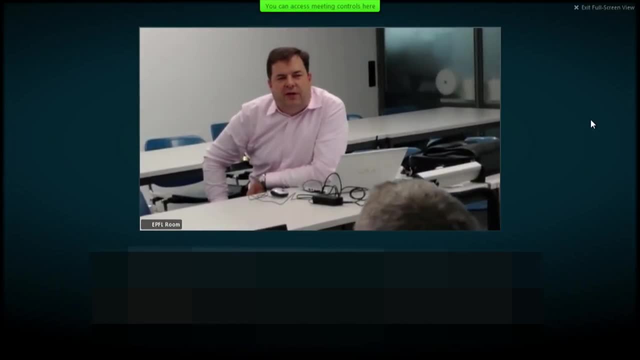 and all you students will love this. it was the smallest brewery that ever flew in space and the initial requirement was that all fluid containers had to be fallen with double walls, and this meant that we had another solution with bladders中共 drum. we had a real fight up front in the proposal phase to demonstrate the compliancy to the. 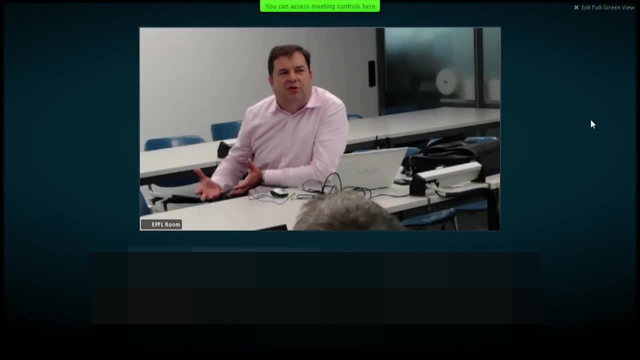 to the requirement of doing the cell culture, yeast cell culture, and still being non-compliant actually to to this requirement of hard, double walled fluid containers. and so this is exactly the point. finally, these flew, and they've been, they've still been flying now since the last. 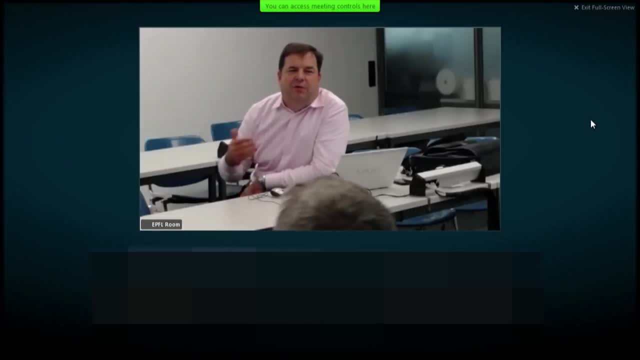 uh 15 to 20 years, and this was a breakthrough in technology. and there you will always have these challenges with the agencies, with your customers, because they are used, set in their ways and and you have to demonstrate the feasibility and then to make them a change in requirements. 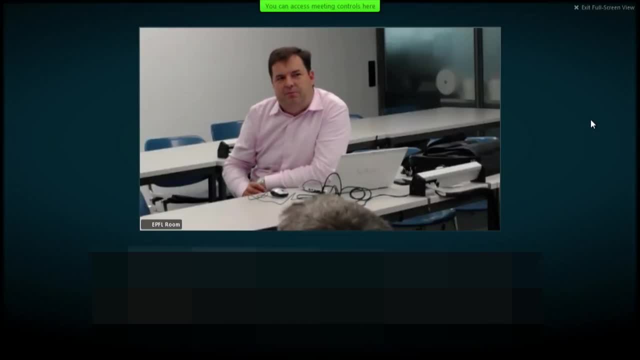 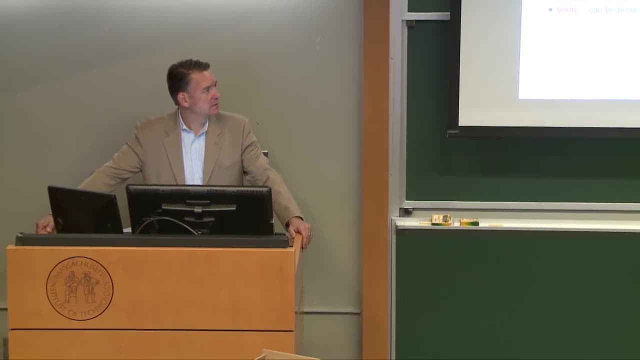 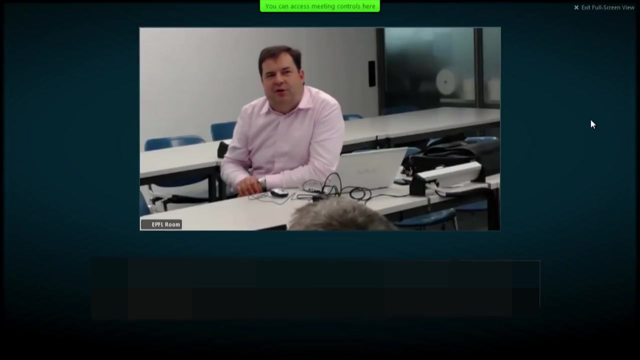 that allows you to change the specification now. i think that's a great example. so in the end, you were successful to argue for the bladder, the bladder solution. well, the bladder was just how to keep the fresh medium and the used medium, meaning the beer. the technology we wanted to put in there was men's technology for space. 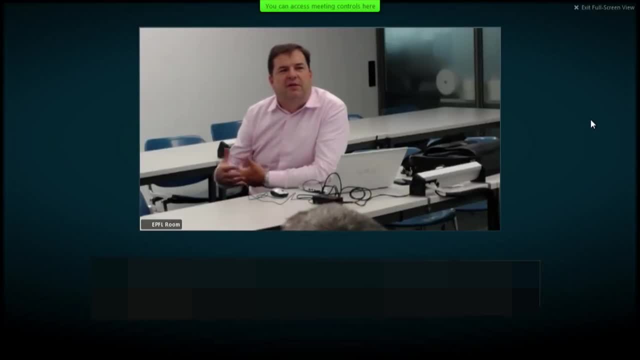 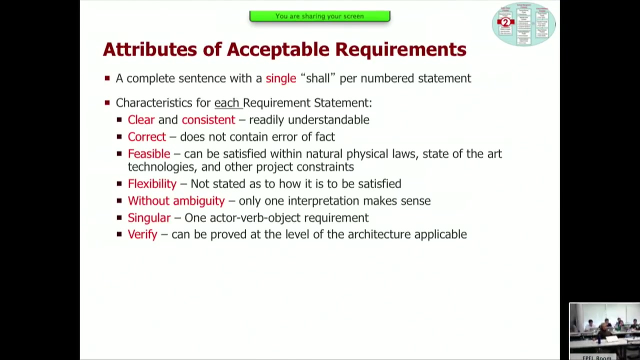 and actually it needed to have flexibility on the, on the pressure in the reservoir. that's why the argument to put men's in space finally won the day and allowed to relax the other requirements. yeah, thank you. thank you, the great example there. any any other comments? okay, so so all this is a pretty long list and this applies to single requirements, and then and then. 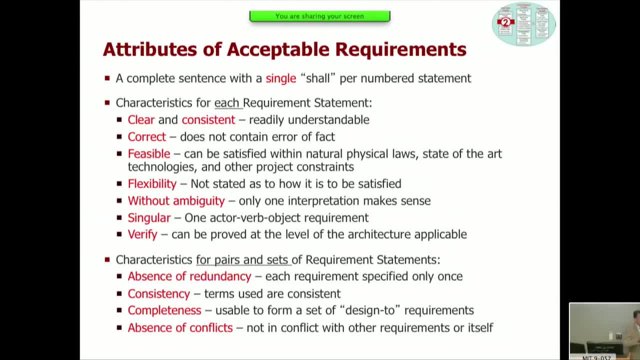 there's a set of this is really important. then there's a set of characteristics that we want to see. uh, when you look at sets of requirements, groups of requirements, absence of redundancy. this means that each requirement is specified only once. right, you don't want to have redundancy. 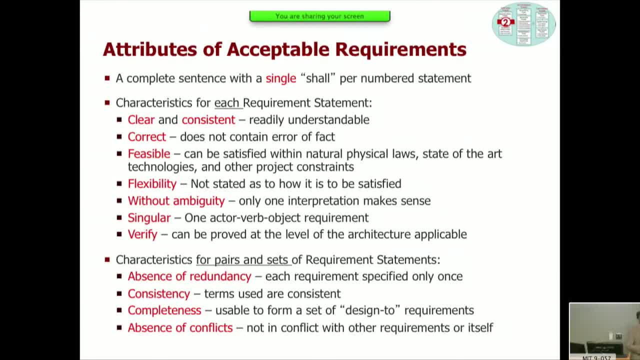 redundancy can be good in system design, but not in the system design, but not in the system design. but you're not going to have redundancy in the system design but you're not going to have redundancy in the requirements. okay, consistency, using terms, completeness, and this basically means not missing. 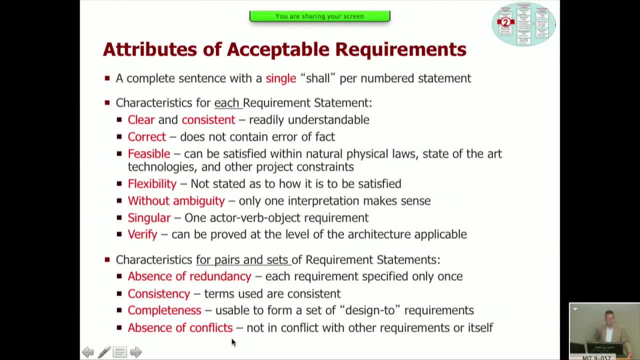 key requirements, and then this idea of absence of conflicts, and this is also similar to the feasibility. this is a tricky one, uh, requirements can be in tension with each other, particularly if they're there should write goals, but they they shouldn't be in direct conflict with each other. 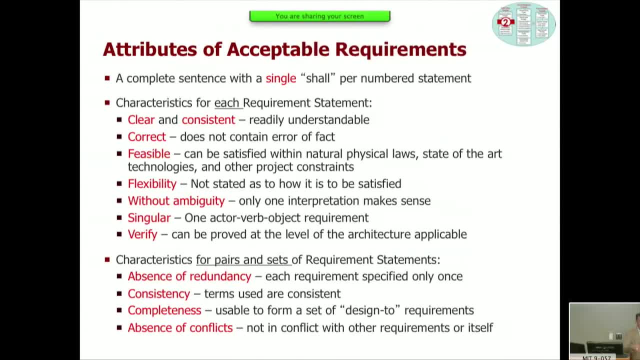 like you know, you shall use uh, aluminum, for this unit. and then another requirement says: no more metals are allowed to be used in this unit. but that's you can't. that's that conflict is not solvable. that's a direct contradiction. that's different from having competing requirements or requirements intention. so let's do a. 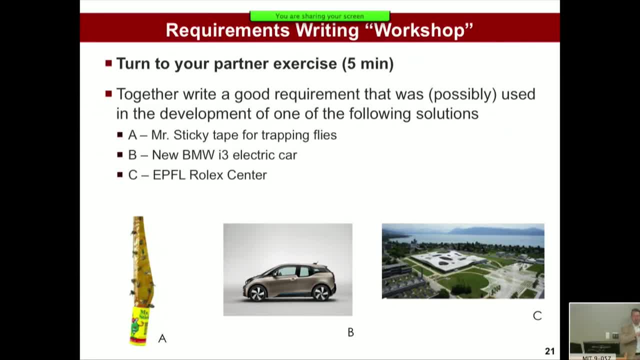 quick exercise and then we'll actually take a break as well. so this is a turn to your partner: exercise, and then we'll we'll have a break and we'll restart in like about seven minutes. so here's what I'd like you to do. I have three systems. 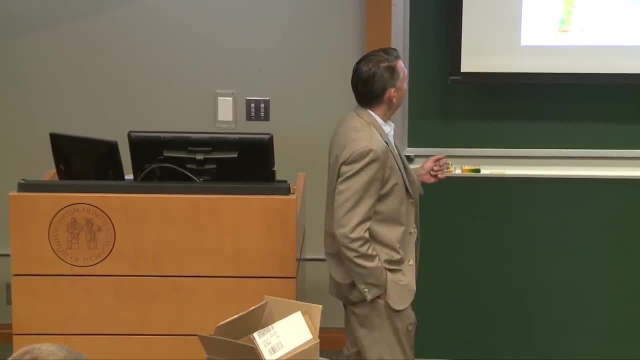 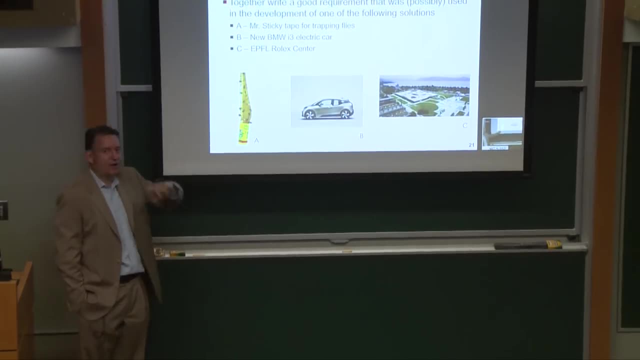 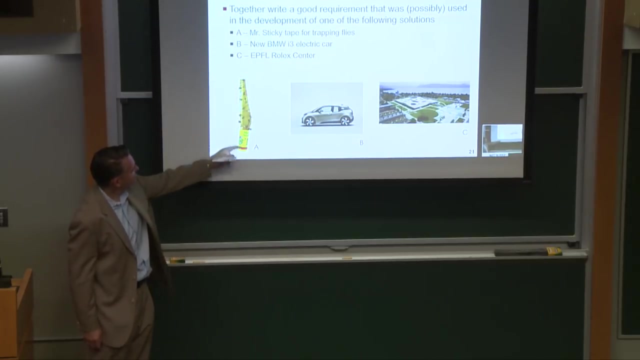 here. they're very different in scale and complexity. so a is a sticky tape and I'll tell you the quick story here. I grew up in in Switzerland, surrounded by farms, you know, and I spent all my times at the farms and you know big tables, big families, and this is they have these things here. this is basically. these are. 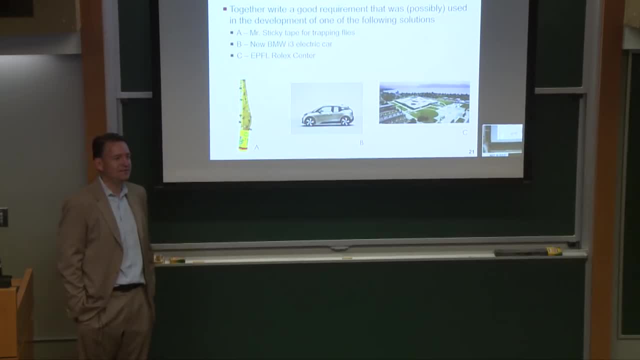 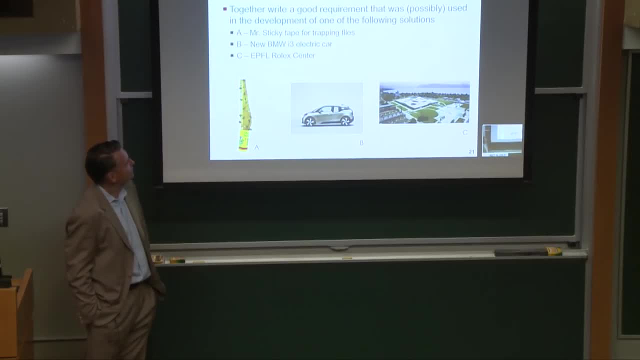 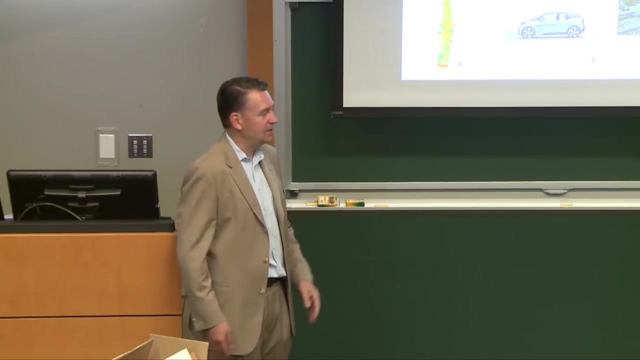 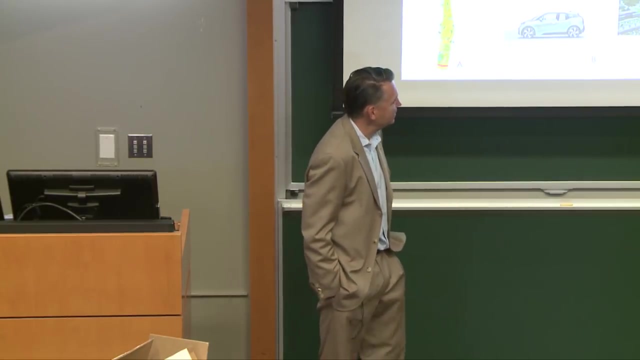 dinner table. it's called mr sticky tape for trapping flies. really kind of gross, but I remember it. B is I just a couple of weeks ago had test drive and the new i3. this is the BMW small electric city car- very cool. and then C is something that at EPFL you guys know very well. this is the Rolex Center. it. 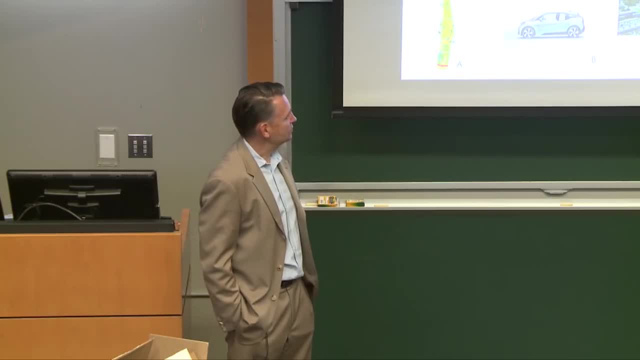 looks kind of like Swiss cheese when you look from the top. this is the sort of equivalent of our w-20 here at MIT. this is the Student Center, so there's, there's a library there, there's, there's cafeteria there, and so forth. so what I'd like you to do is turn to your partner. pick one of those. 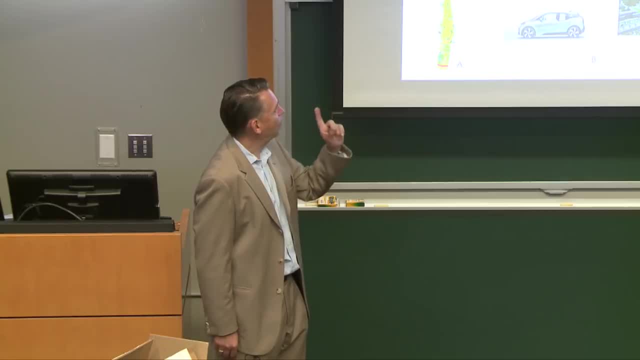 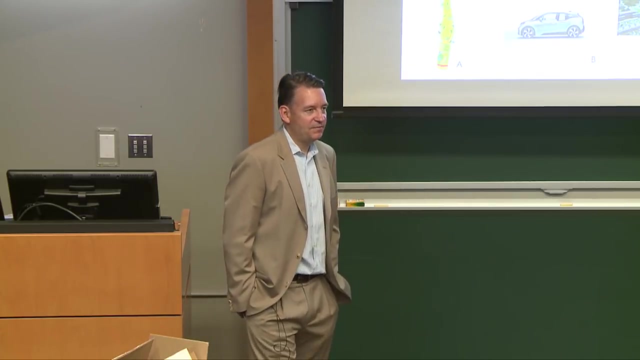 three and come up with one, one single statement, one good requirement that you think was possibly used in the development of that solution. whichever one you pick. okay, so pick one of those three and then jointly discuss and write a requirement that you think led to this design. okay, so take about five minutes, take a break and then. 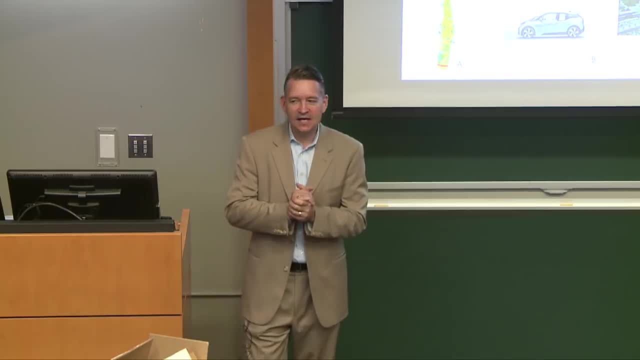 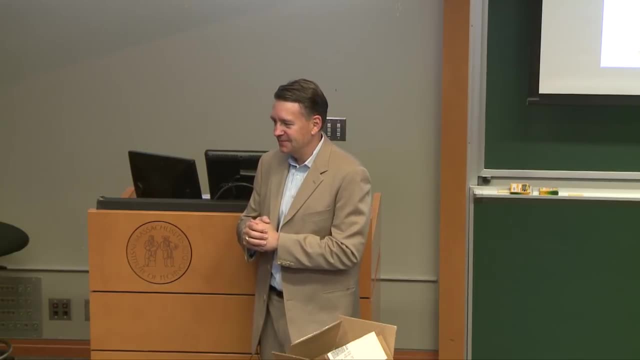 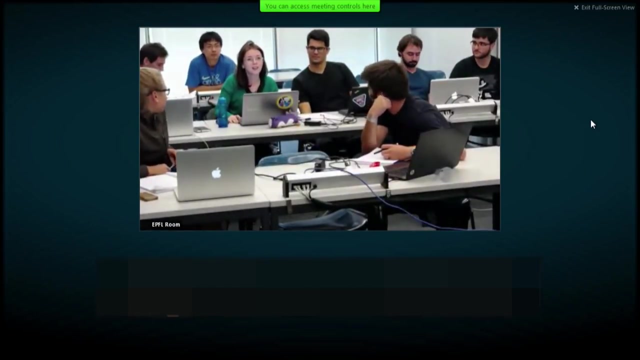 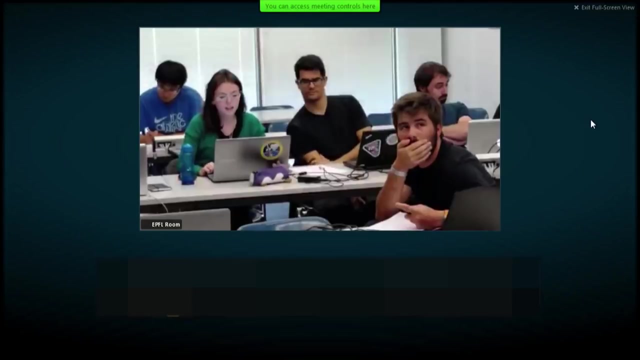 we'll. we'll sample what you came up with. so let's, let's hear from EPFL first. who did? did anybody do a? okay, go for it, speak up. we have four requirements for you. okay, go for it. all right, so the tape shows six flies, the cost of the tape. 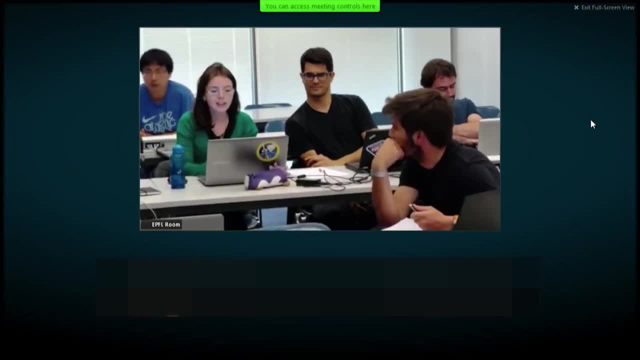 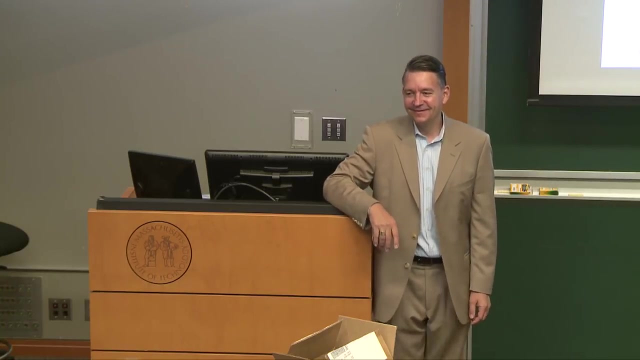 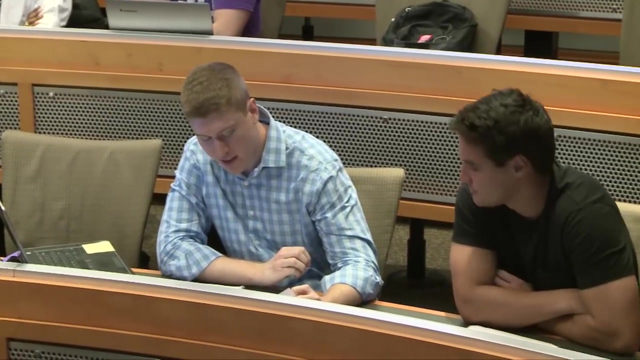 should be less than four grand. the tape shall be able to catch up up to 50 insects and the sticky tape shall not be toxic for humans. okay, I like. yeah, the toxicity. that's good, excellent, very good. who did A here at MIT? anybody A go for it? we said if 10, if greater than 10 percent of the surface area of 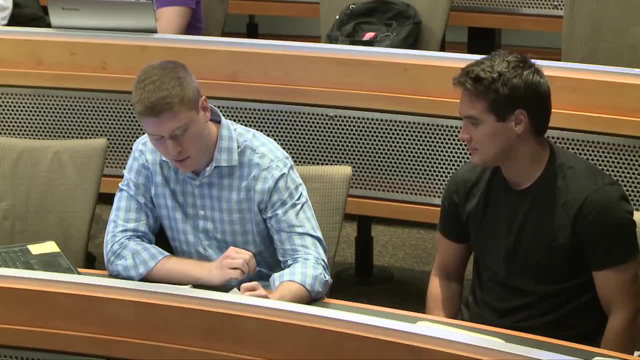 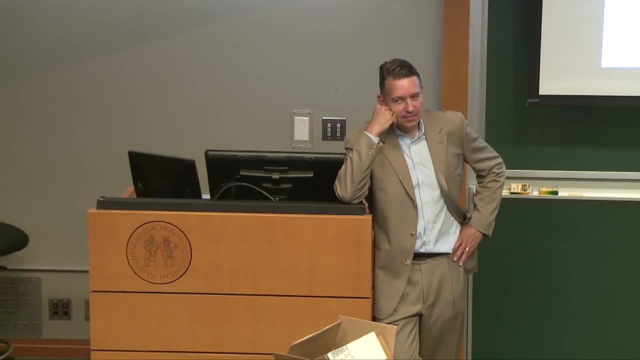 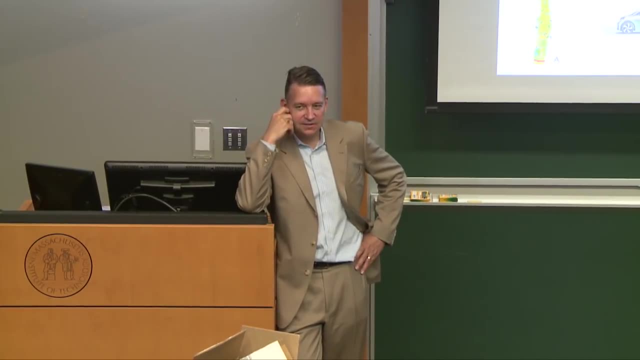 the fly contacts a paper, it shall not be able to release itself. I see, so this is a trapping requirement. yeah, how effective should it? there are different, very different flies. right, there's like these little dayflies, and then there's the huge horse flies. so which flies should be the most effective flies? 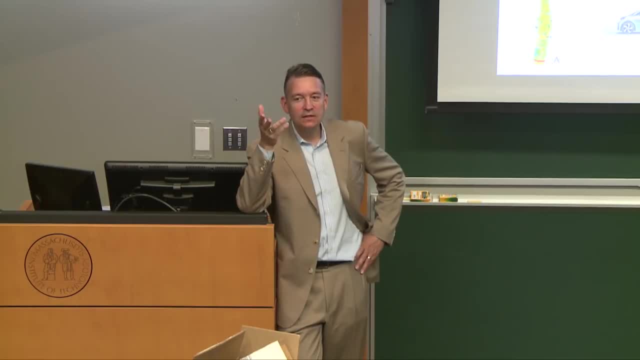 What type of fly does this apply to? We said 10% of the surface area of the fly, Of any type of fly, Of any type of fly, Any of the different fly species. Yeah, Okay, All right, Cool, So good. 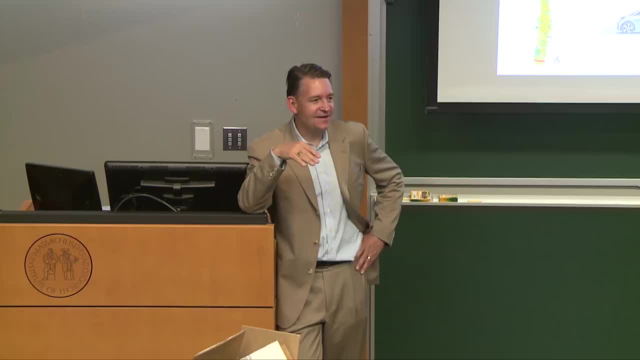 Well, you know the point of this. you get the point of this is right. A is, like you know, this sort of, you think, trivial system, But once you really start thinking about it, it's pretty tricky, right. 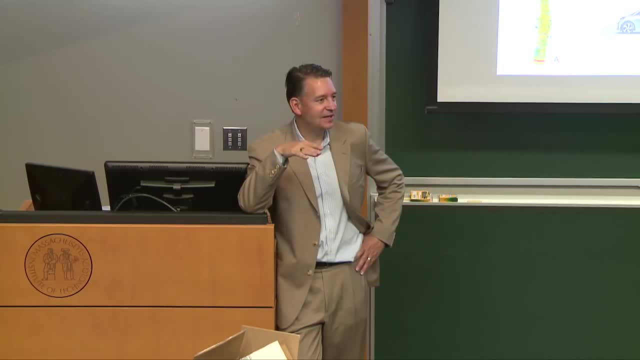 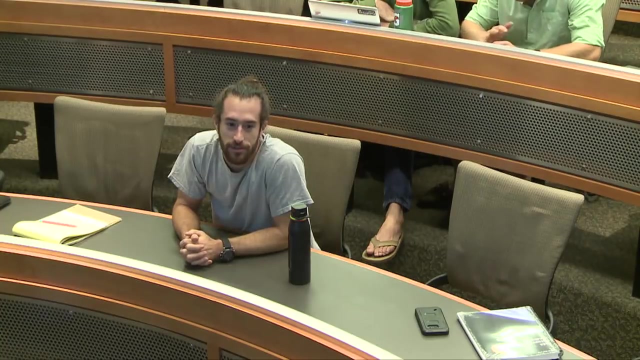 Who else wants to A something that hasn't been mentioned yet. On A Sam, go for it, Just push. make sure you push the button. Yeah for the sticky trap. we said that the product shall fit on a store shelf when packaged. 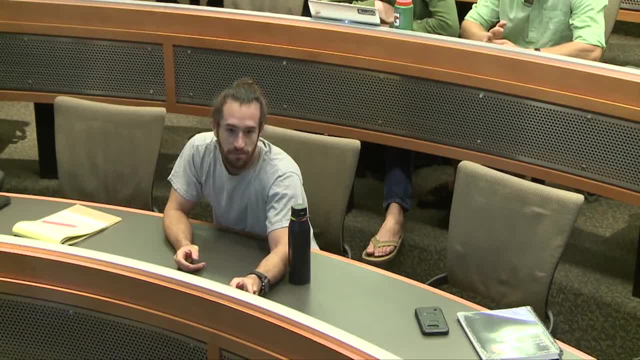 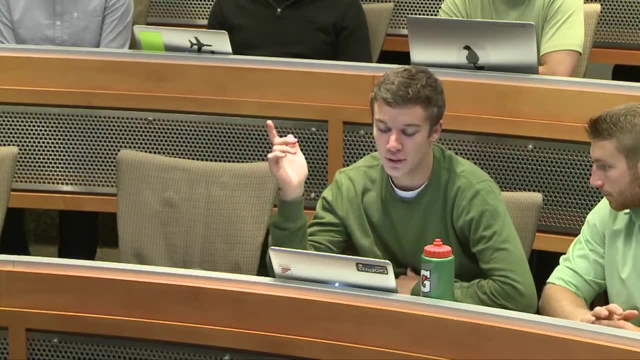 Okay, So that's kind of a packaging logistics distribution requirement. Very good, Mike, They kind of already touched on it, but the sticky tape shall not be toxic and allow for allow for removal, Removal of human skin without bodily harm. 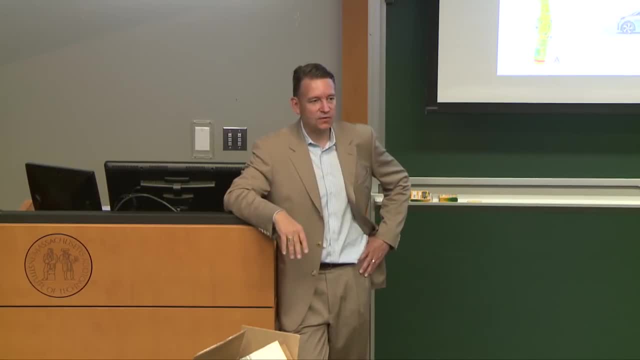 Okay, Great, So that's in the same. you know human factors requirement. basically, Yeah, Very good. Anything else on A at EPFL? No, Well, just keep in mind here that we could say that the sticky system should be installed. 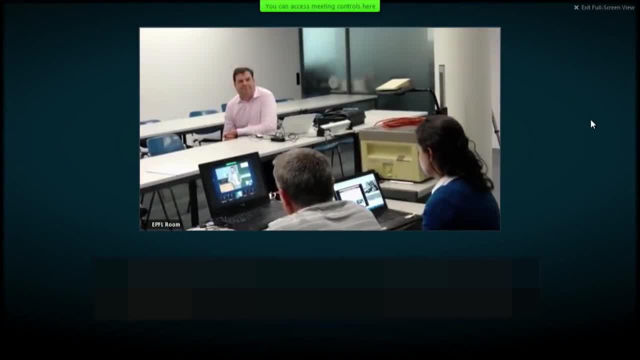 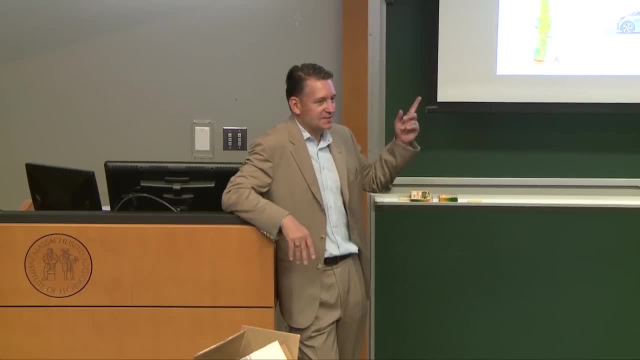 without getting the mess on your hands. Okay. So installation requirement: Okay. Okay, Nobody mentioned The ones I remember as a child are bigger than this. They were really long. So capacity: right, You could sort of have a length or capacity requirement as well. 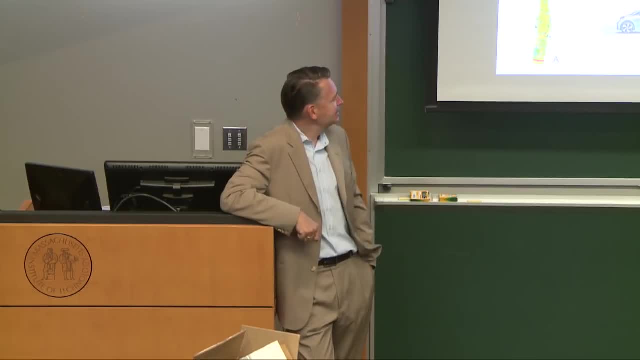 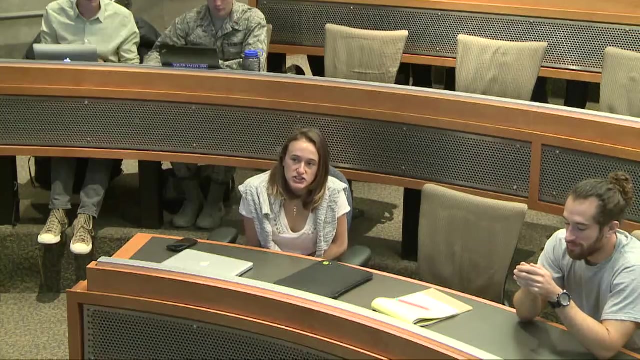 Good, All right, I think we want to move on from the sticky flies to BMW i3. So we had a little discussion here during the break. Lucy, go for it. So the car shall meet environmental regulations through. So the car shall meet environmental regulations through mechanical. 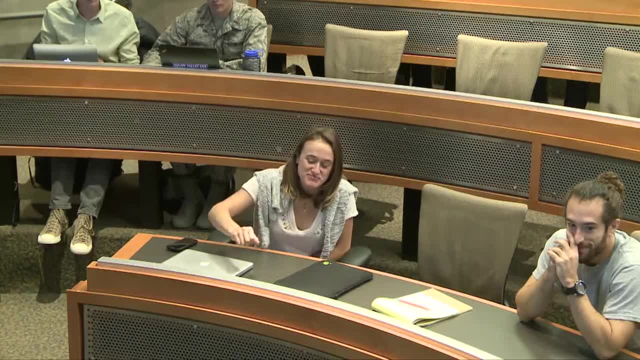 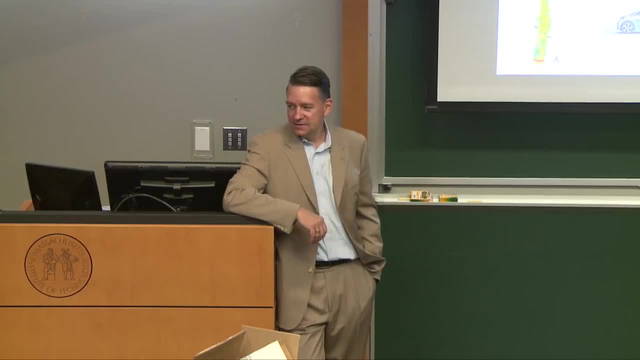 or software tweaking was a proposal. Did you guys hear this at EPFL? You've been following the news right with Volkswagen. So what happened? Why did folks? the CEO just stepped down, right, That's kind of a big deal. 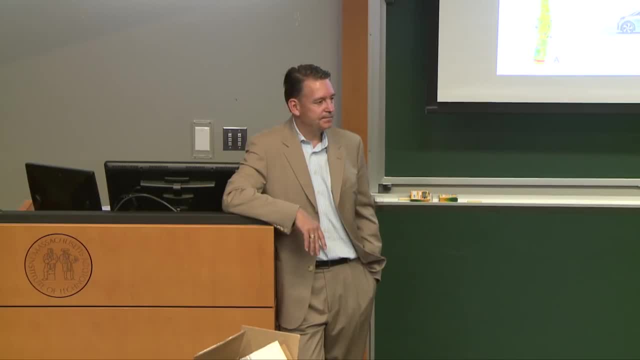 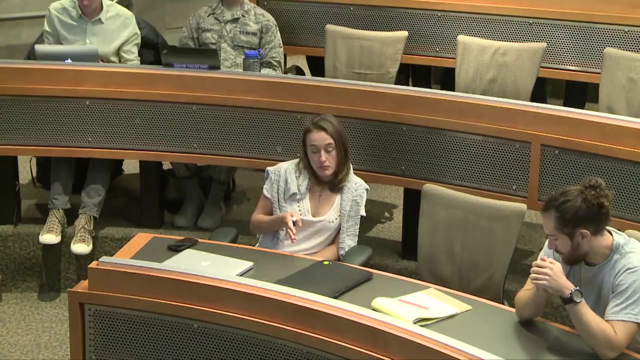 Trust in the company has eroded. What happened there? So the requirements that were set at the start of the year? So the car shall meet environmental regulations on emissions. This requirement was probably not met, but the realization that it wasn't met was probably too late in the design process. 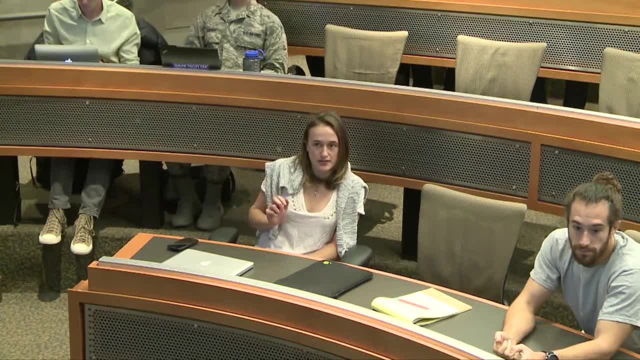 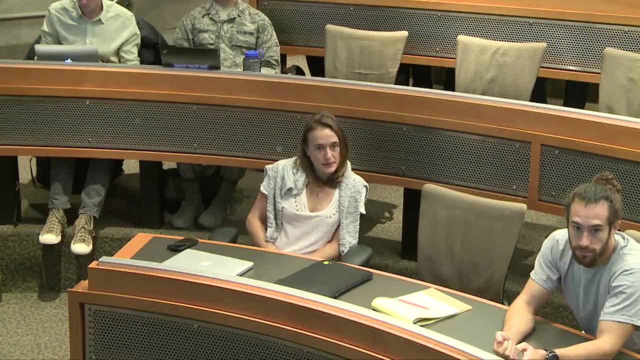 such that it cannot be changed, And so the easy or cheap way to meet environmental regulations in that case was to tweak the software, I guess Right. So, by the way, this is kind of interesting: How do you measure environmental compliance of emissions? 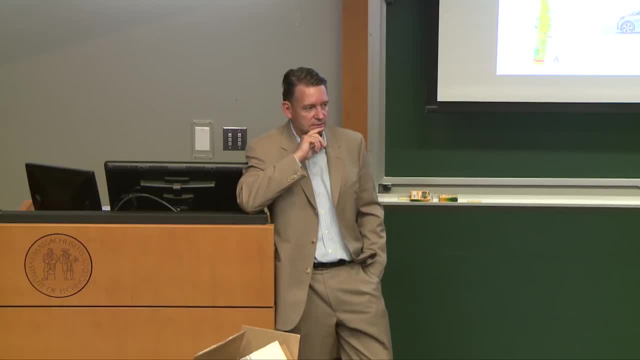 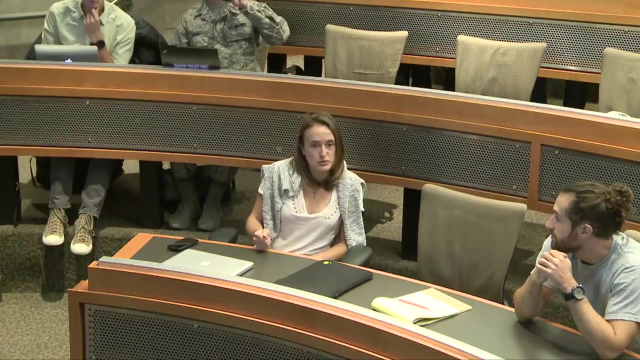 Do you know how that's done in practice? Do you guys know? So it's having the can run on a, having the. yeah, the engine run, but the car's not like rolling And there's behind the exhaust. Behind the exhaust you measure whatever is emitted. 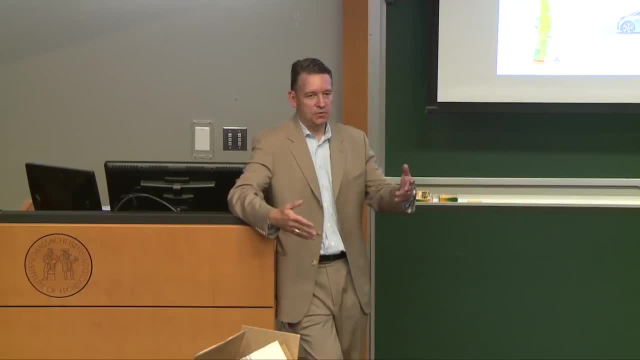 And it's like on a rolling carpet right, It's a dynamo, basically. And Yeah, Yeah, Yeah, Yeah, Yeah, Yeah. And the way they do it is they have so-called drive cycles, Like there's the FT FP6 drive cycle. you know the highway. 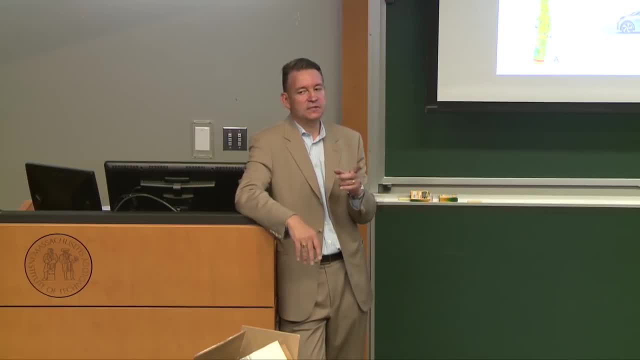 the city cycle, which is a lot of on and off, And those drive cycles are actually different in Europe and the US and other countries. Every country has different drive cycles. So that's and what is a drive cycle essentially. 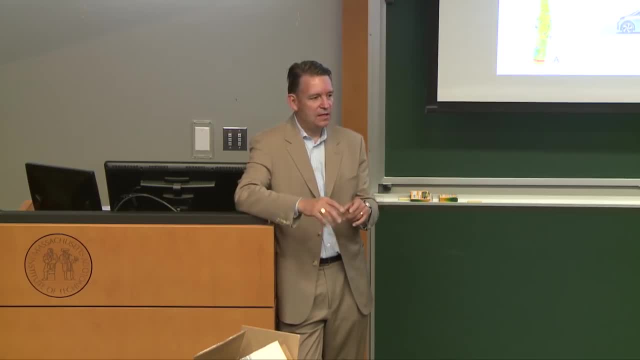 What word would we, as systems engineers, what word would we put? Con ops? A drive cycle is just a over time accelerations, velocity of the car right, It's a con ops. It's a con ops. A drive cycle is a con ops. 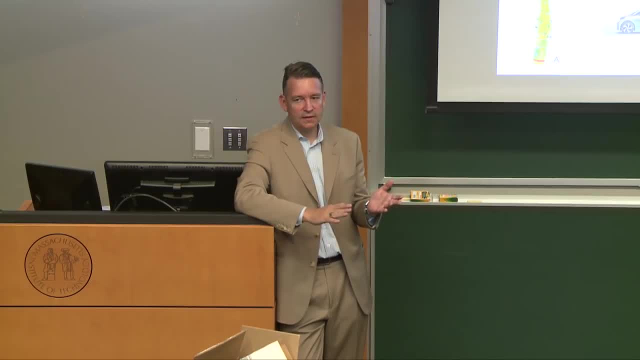 And so for diesel engines, this issue that happened with Volkswagen. it's only an issue with the diesel, the TDI engines, right, Not the gasoline engines. So the issue is that the con ops the drive cycle in the US with TDI engines. they couldn't meet it, So they came up with this trick right, Whereas in Europe they didn't have to do that because the European drive cycle- there's a lot more diesel engines used in European cars. They didn't have to do that in Europe because the con ops the drive cycle that's used. 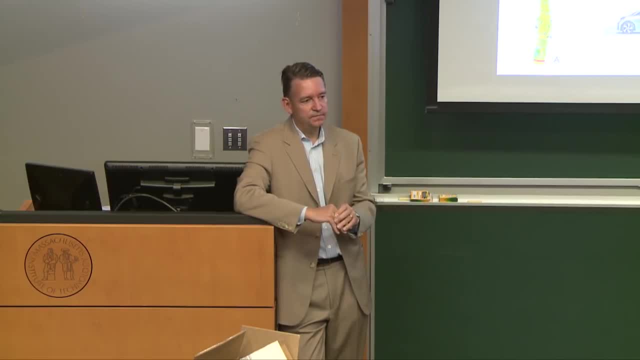 for checking the environmental compliance is different in Europe, So great. Anybody else on the i3?? Now, the i3 is interesting because that's actually an electric car, right, And once it so it doesn't have an engine, a diesel engine. 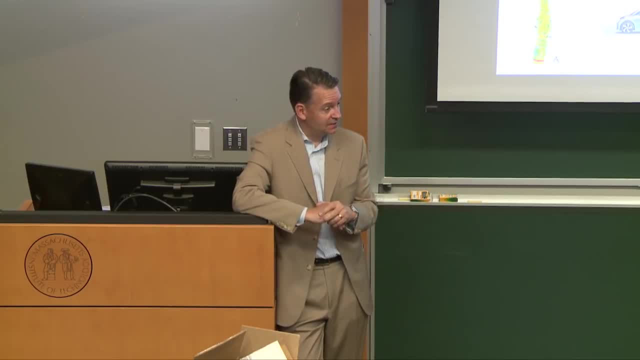 Right, It doesn't have an engine or a combustion engine, except if you get the range extender. So it's all electric. but you can actually- it's an option- get the range extender which does use fuel. Okay, EPFL, the i3, any other requirements there? 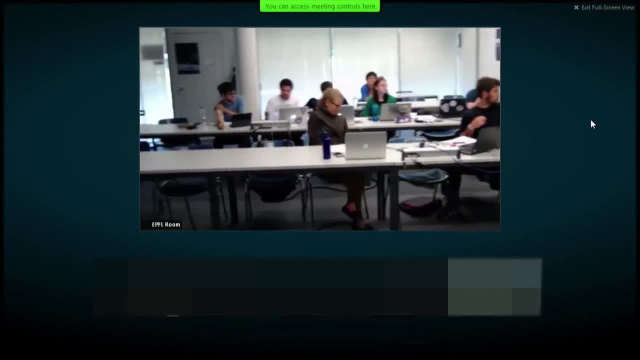 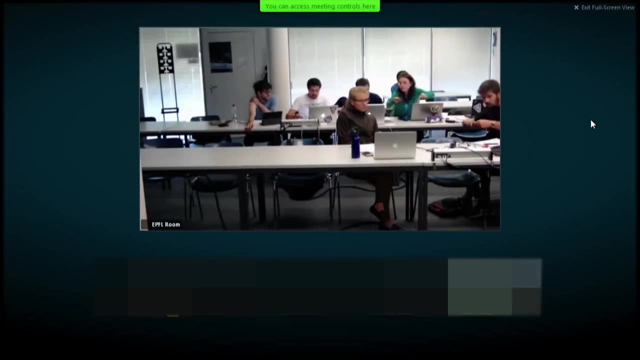 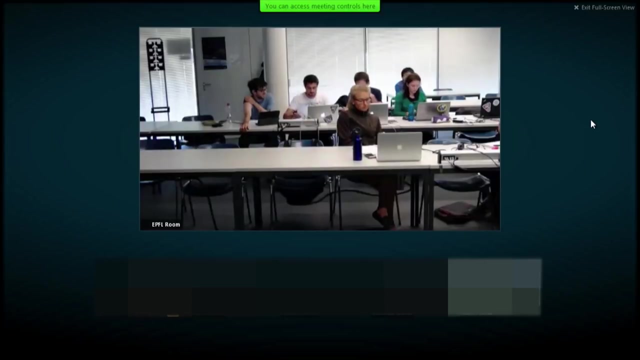 So we have four, beginning with, like the car shall rely on electricity as unique force of power. Then, apparently, the autonomy for the car, should it should drive at least 150 kilometers in city driving conditions, like the cycle we just talked about. 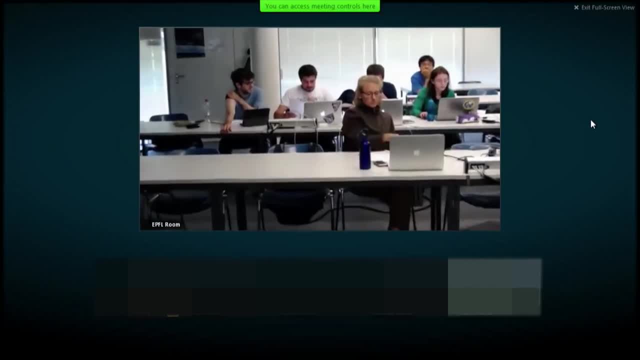 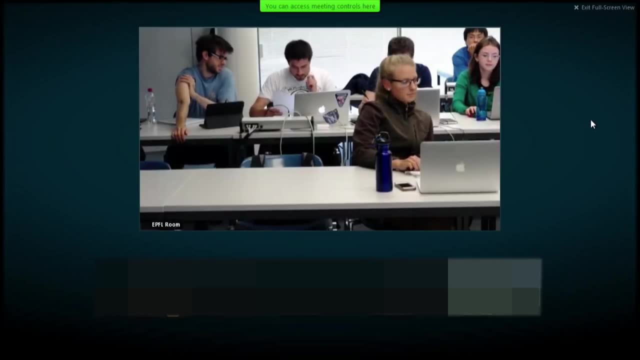 Yeah, And the third one: the car shall carry 45 percent of average fuel. And to finish with, the car should be fully recharging less than a given amount of time. Okay, So recharging. The third requirement is interesting. 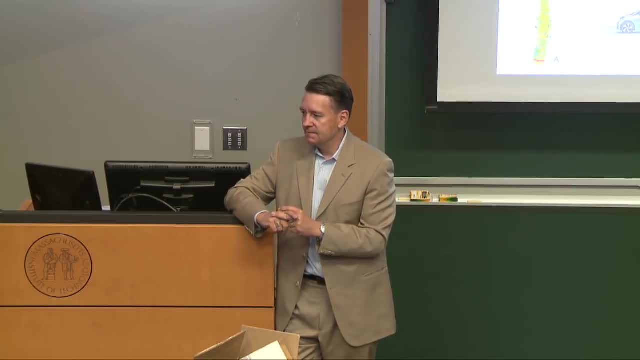 You said of average build. right, That's the word you used. Yes, Now that's great. That's a human factors requirement. Now, of average build is a little fuzzy, right? How would you make that? make that more verifiable? 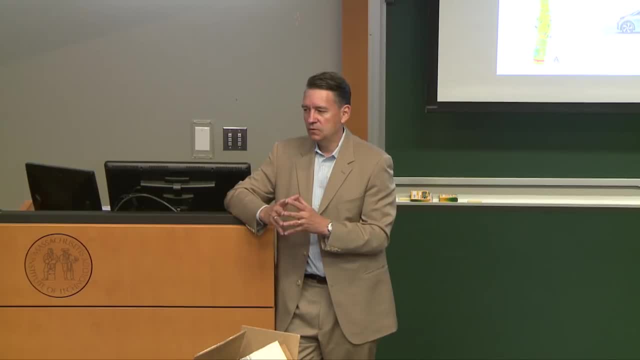 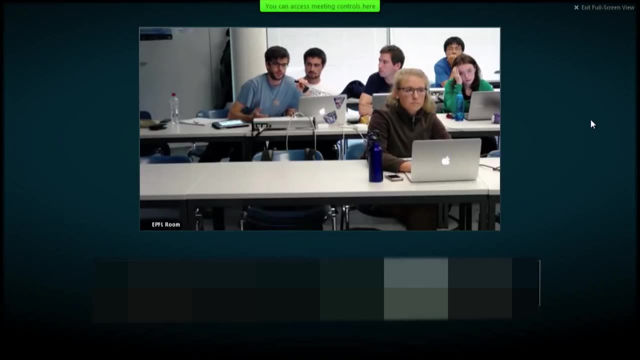 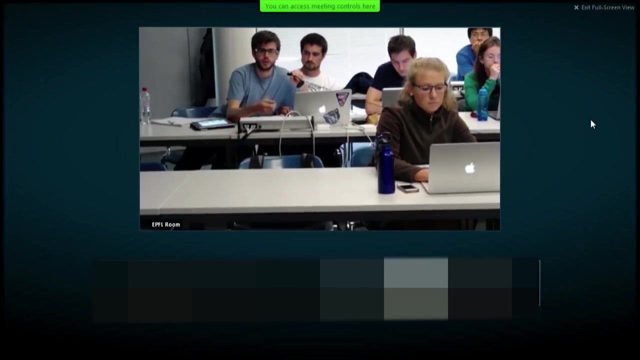 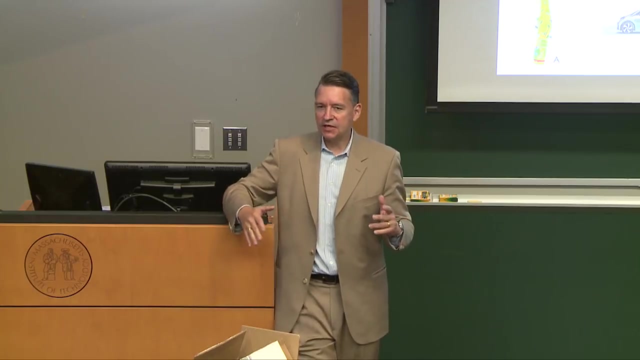 The thing is that if you just say it's four to five people, it's very broad. You could have someone who's very large and very small. You have to be more specific. Maybe you could be more specific, But the Yeah, So there's actually people that you know the size distribution- male, female- you know weight. 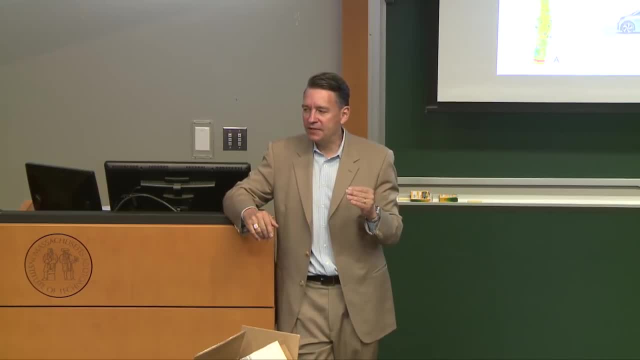 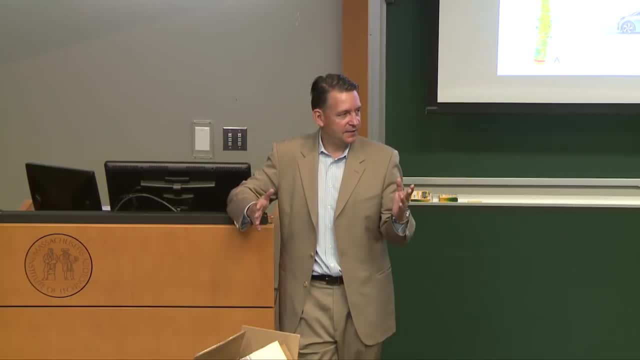 world people are getting heavier. we know that right. so the way you would write that third requirement to be verifiable is the: the car shall accommodate four passengers, a male or p5 female and a p90 male, right. and if you write it that way then you know the actual weight and dimensions of the human body can. 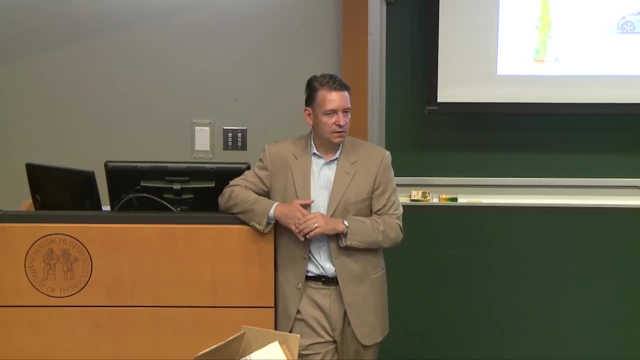 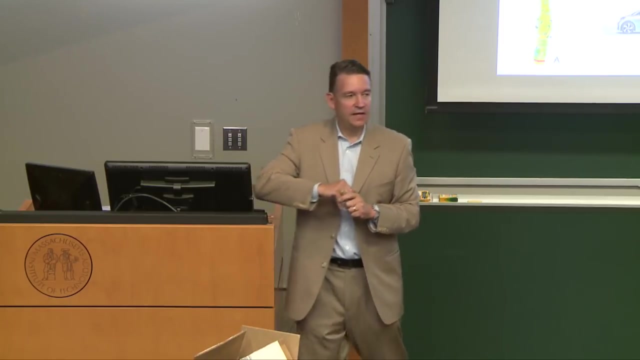 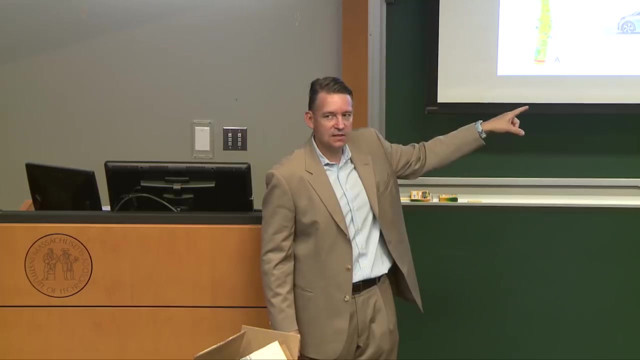 actually be traced to a database that's pretty well known. so then, instead of saying average, build you, you say it's a peak, p50 male, p50 female, and that's, that's something that's very verifiable. does that make sense? okay, great, so what about the last one? so, by the way, here at MIT, anybody's been to EPFL into the 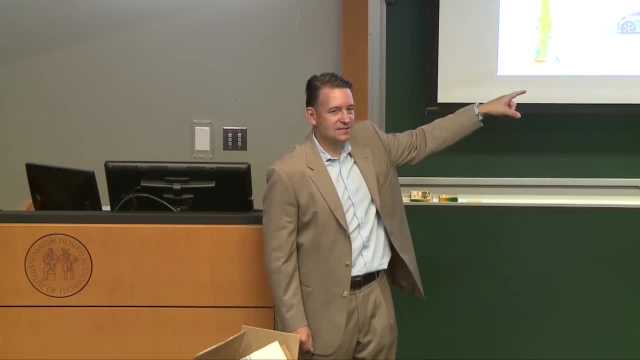 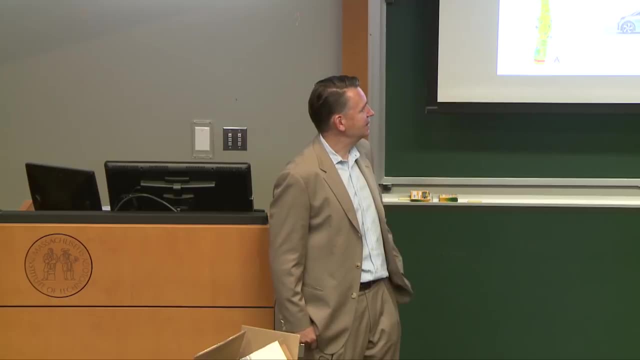 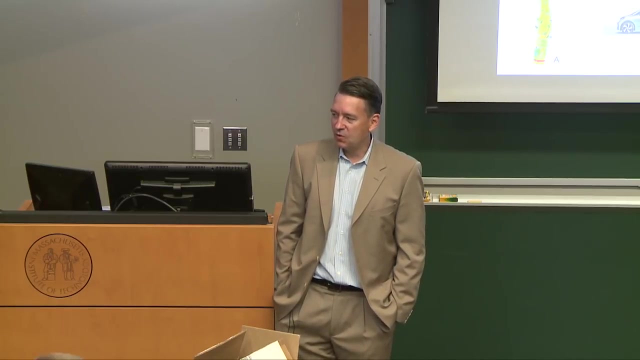 building that's been there. this is a very cool building. it's, it's, it's pretty unusual. I mean we have some very unusual buildings on campus to here, but you get a chance, it's pretty unusual, so let's hear from you guys. so what, what do you? 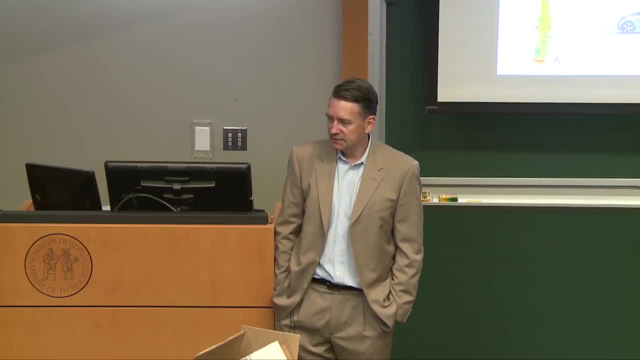 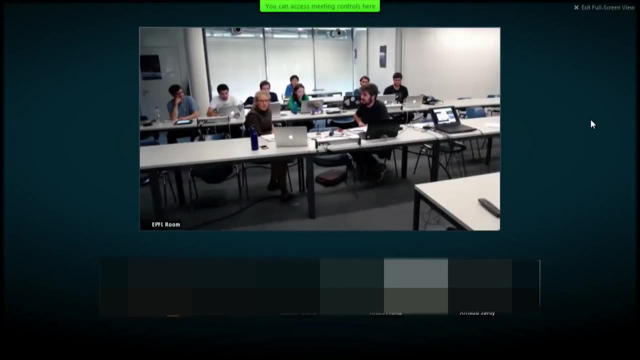 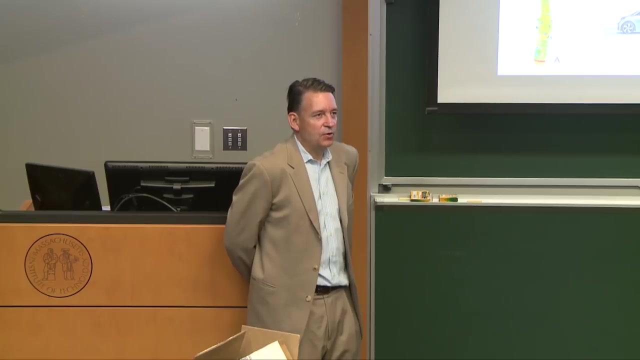 think was a requirement for the Rolex Center design. the building should be a recognizable structure that would be memorable for EPFL. ah, interesting, a recognizable structure that should be memorable. so that's I think I know where you're going with this, but it's a little, you know. 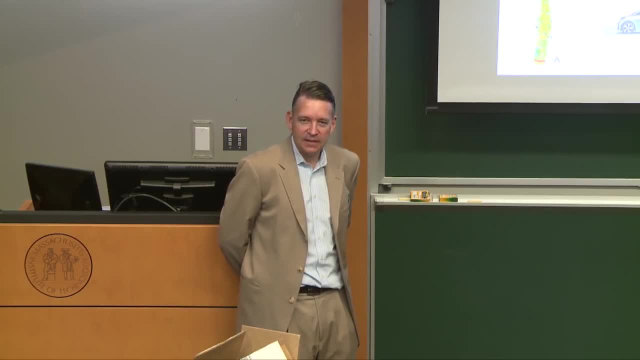 recognizable. every building is recognizable in a sense. right, I think I like it. I I know where you're going with this, but it's a little fuzzy still, right. so what? why? why do you think it has holes in it? what do you think? the holes in it might be a better word. and so she's. yeah, so there's, there's. that's really the. 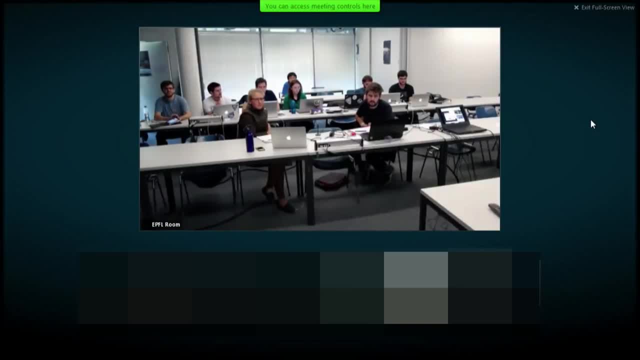 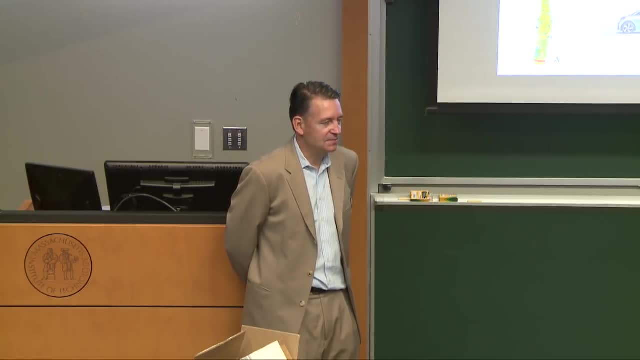 whole. the holes are in some sense inefficient, right, because you're putting holes in the middle of a building, but they provide natural lighting and there's a symbolism there, right, there's a symbolism, the Swiss cheese symbolism. so it, the holes, in the sense, have at least two functions. right, that's good. 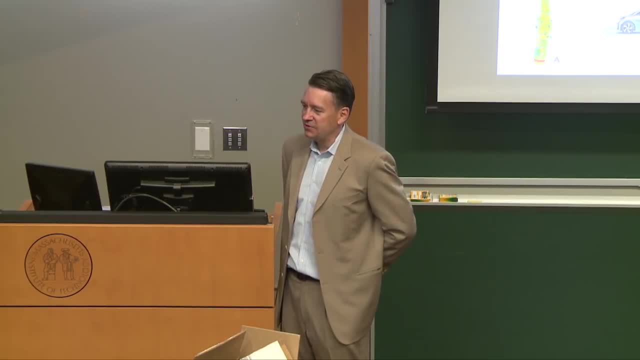 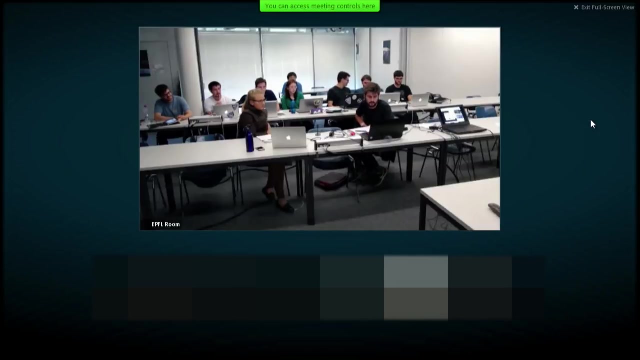 that's good. I like that. that's. that's very good. what out? what else? another example of a requirement for the Rolex Center: we've taken an exponential in each three imp. Benedict, That right and this shoulder has a library to cafe. behind Android, inemen direct the work, Rolex and Lefty. 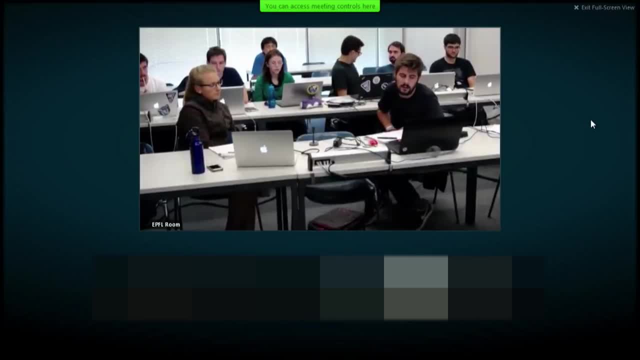 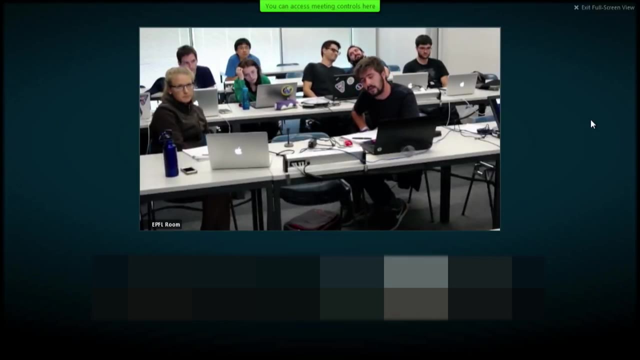 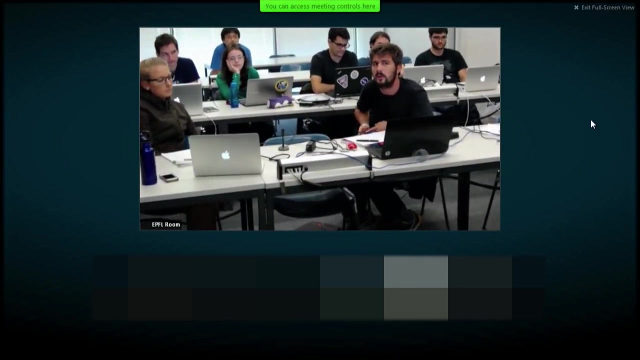 need energy to zum expectations in construction and The RELAX Center shall be accessible even for disabled people. interface and the RELAX Center shall interface with the existing internet network and I'm not going to say this because we do not have any clear requirements. 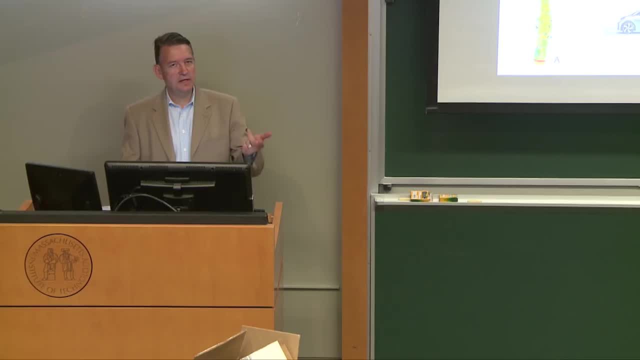 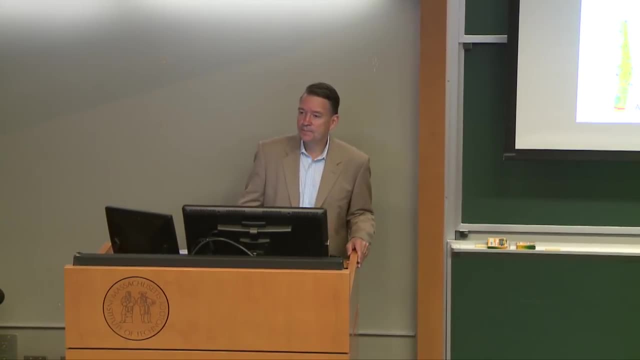 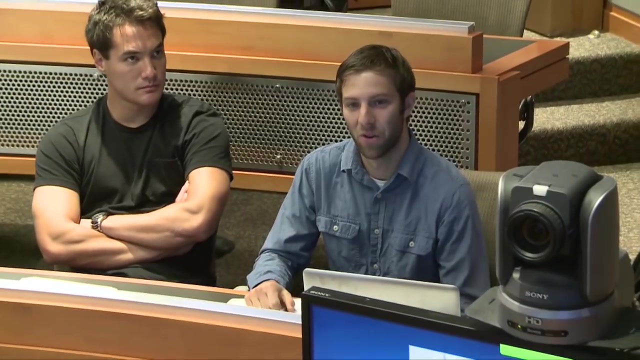 Good, No, that was great. So you had functional requirements, you had interface requirements, you had a lot of those six categories we talked about. right, Very good, Excellent, Yeah, go ahead. So how do you write a requirement about something aesthetic in a way that's not fuzzy, or is? 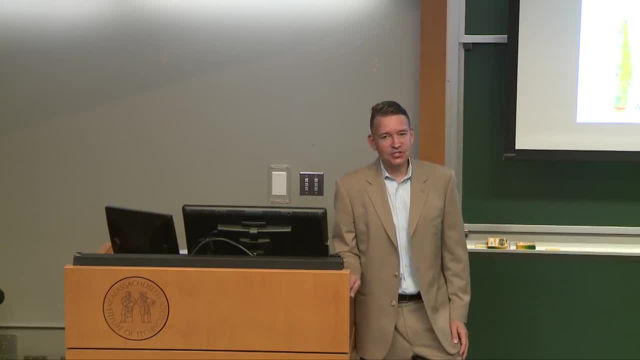 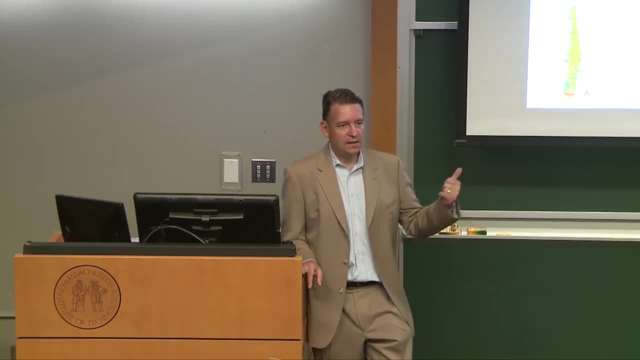 there a way to do that? That's really. that's a great question. I'm not sure I'm the best person to answer that. What I can tell you is, in the automotive world, the aesthetics of automobiles and how people judge, you know whether a car is beautiful or appealing. that's actually moved from being. 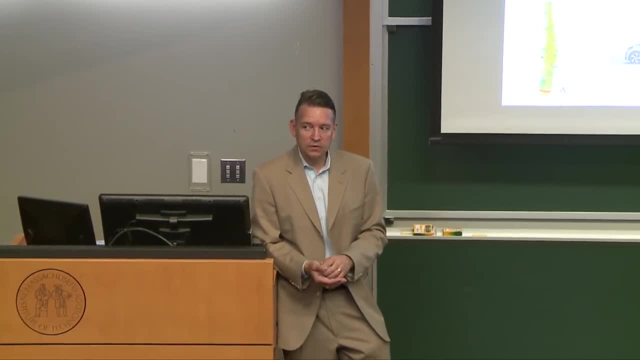 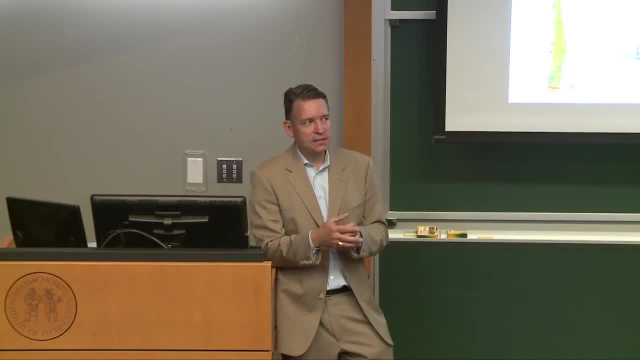 those things are. that's really a science today And eventually you know there's ratings. These are people rate vehicles for aesthetics and so forth, and usually it's a five-point scale, like a Likert scale, like JD. 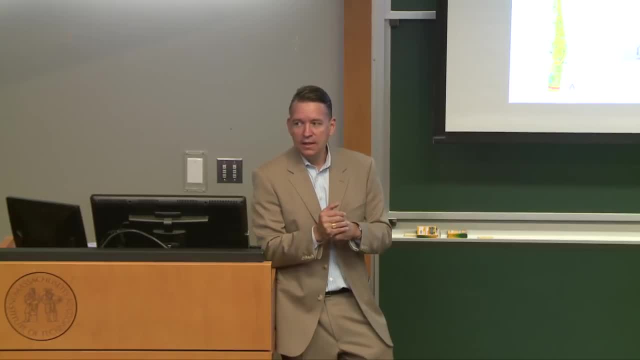 Power and Associates is a very well-known marketing firm and so they'll, you know they'll say, oh, I don't know, this looks, this will. they can actually, at this point, you can show them, not a sketch. 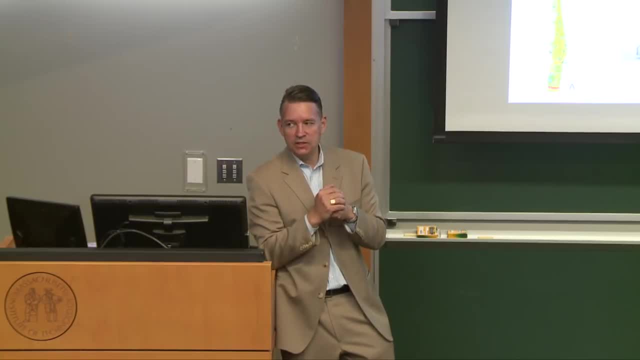 but a model and based on past data and information, they'll tell you this car will probably score between a 4.2 and a 4.4 on the five-point aesthetic scale- JE Powers scale. It's really pretty remarkable. 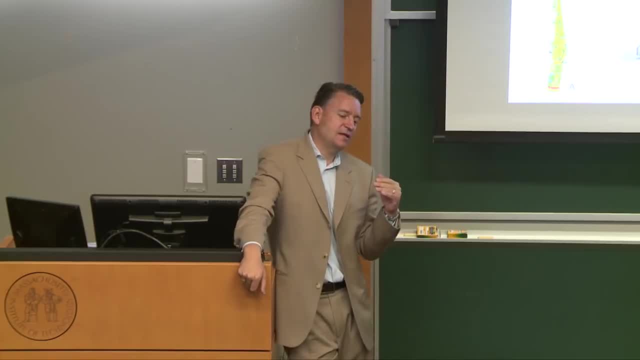 But I guess the bigger point is there's some, you know some things that really delight us, you know that have an artistic quality, surprise us, an aesthetic quality- and it's true that is one of the tensions- is yet a system engineering, should you know this? 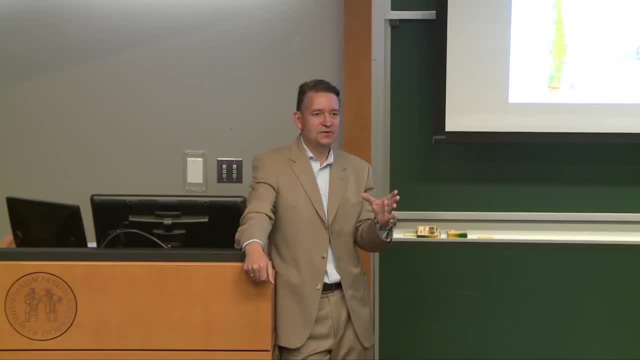 very precise, write it down, make sure there's no fuzziness there, or as little as possible. and then, on the other hand, we want delightful, surprising things right that have artistic, an artistic nature to them, and that is absolutely a tension, and we just acknowledge that. 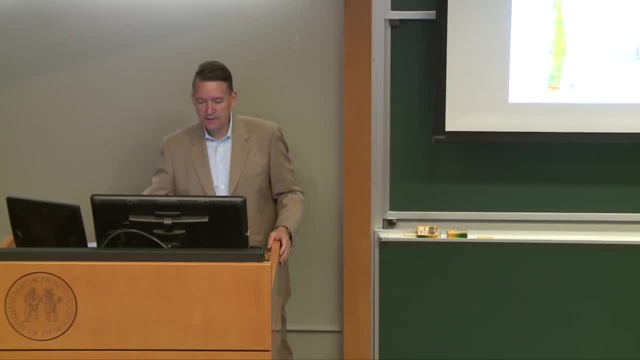 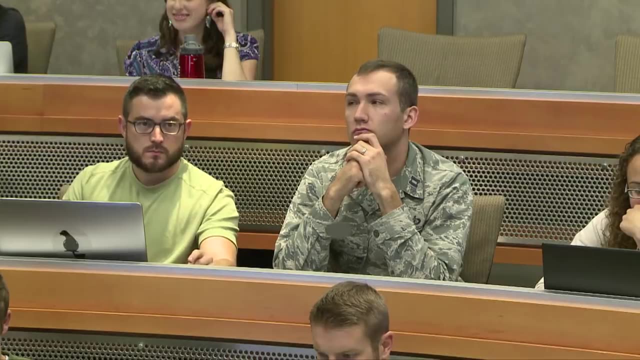 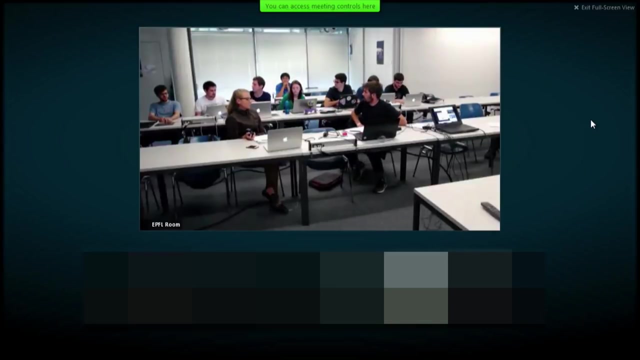 Okay, Uh, any any questions? comments before we move on. I had a question about: um, yeah, Just hang on. just one one second. Okay, go ahead At EPFL. Okay, Um, to which extent can we refer to norms and laws in the requirements? 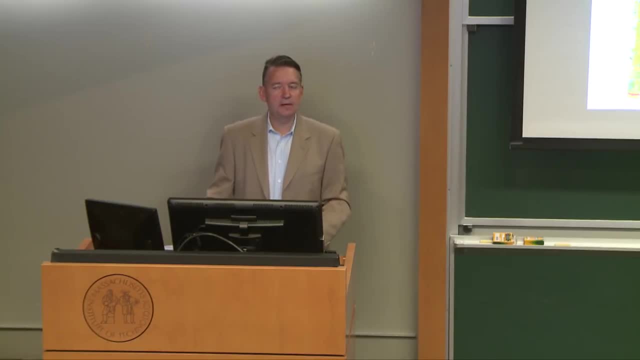 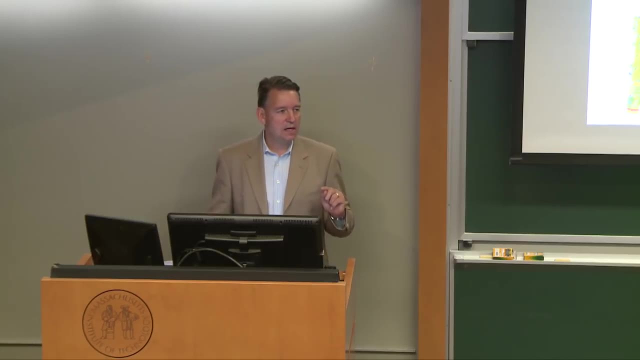 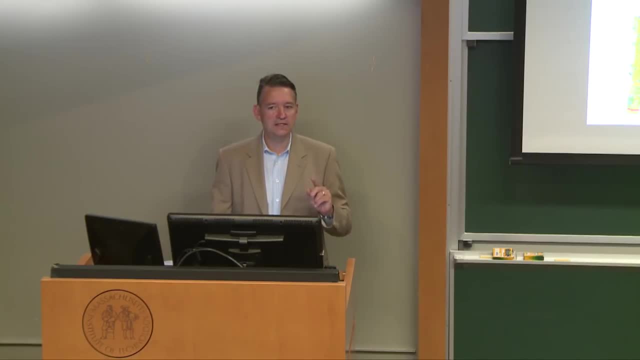 know an IEEE standard or an ISO standard. it's not a law, it's not a legal thing. It's a standard, is something that uh, uh, maybe a group of companies or a group of organizations have agreed to. this is how we will do it right. 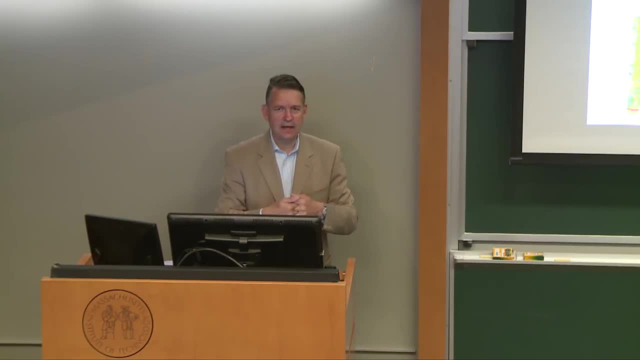 The, the IEEE Wi-Fi standard. what? what is it? 802.11g, right? That's a standard. that's not a law. that's a standard, and if you're gonna be 802.11g compliant, you write that in the requirements. 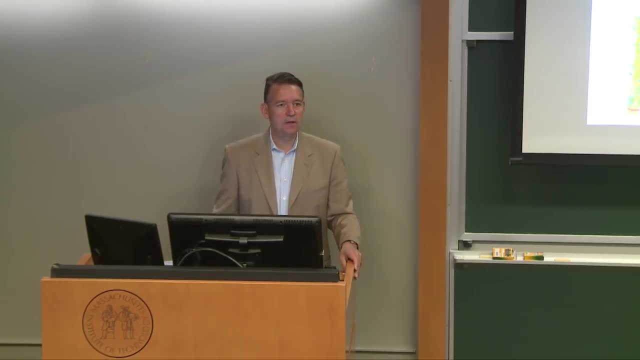 Uh, the environmental emission standards we talked about, those are actually uh laws. If you are going to sell a vehicle in country X, it has to comply legally with these regulations. But you're absolutely right, those are. if you need to comply with these things, it needs. 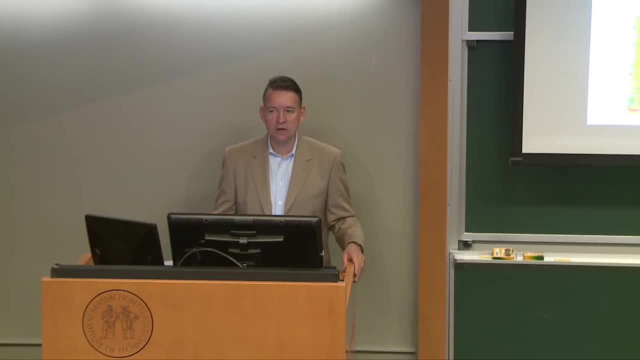 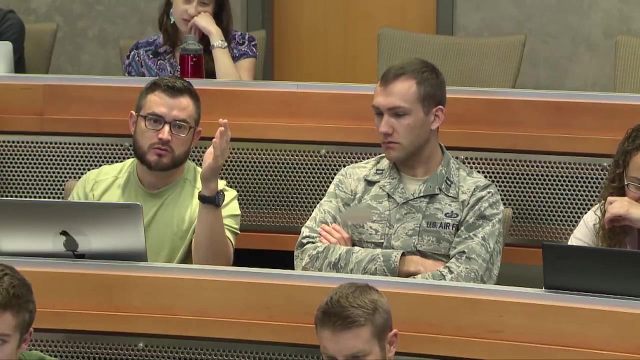 to be part of the requirements set, because otherwise it will not happen just automatically. Okay, Uh, Weston, Yeah, it's kind of along that vein. I mean, if you have to comply, say with ADA, Uh, is that have to be called out specifically? or do you say must comply with building codes? 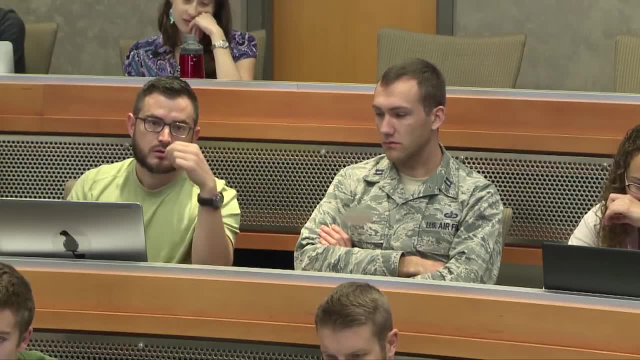 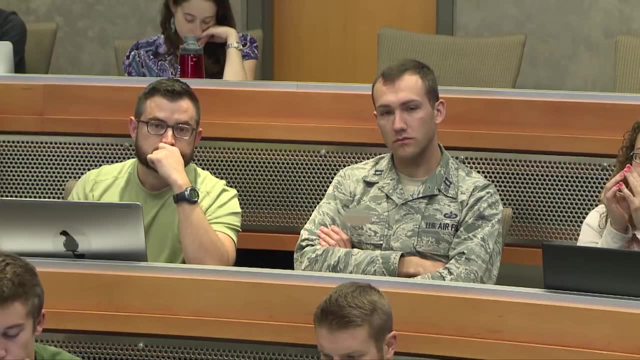 or building laws and and it's sort of a blanket requirement. No, you have to be specific, because you know building law, building codes are, first of all, a lot of these are local as well, and and it's it's uh, it's uh very chaotic. 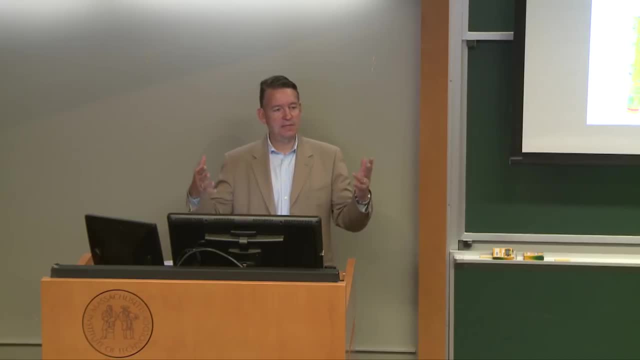 you know so. so, um, and some of these might be conflicting, so you should be as specific as possible. Okay, let's, uh, let's move on here. um, I, my sense is you're, you're getting a gist. 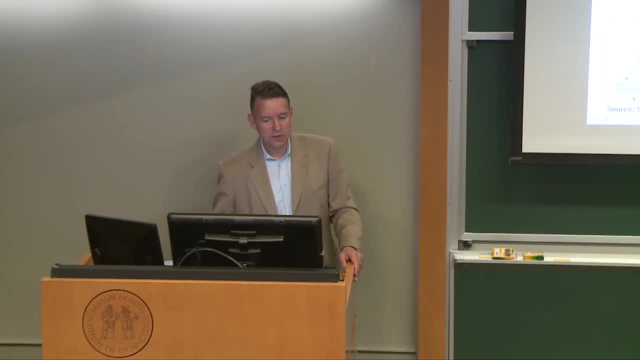 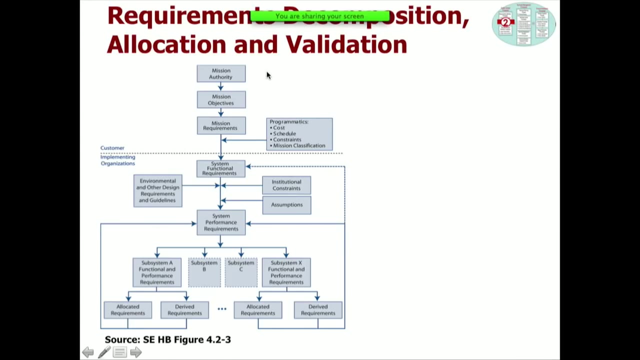 for what requirements are, And and and why they're important. So, um, let me talk briefly about requirements, decomposition, allocation and validation. This is a figure from the NASA handbook and basically what it what it talks about is. 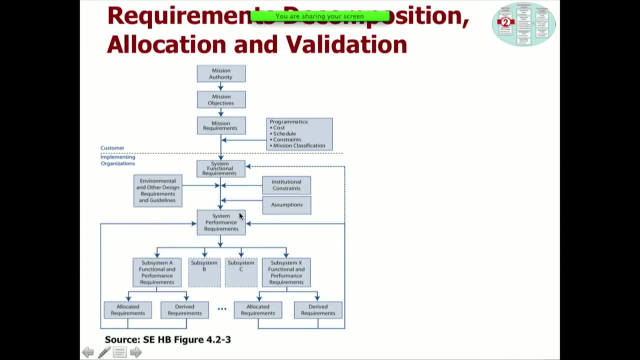 you know, the high-level system, functional requirements are broken down into the performance requirements, and then, as you make design decisions, as you decompose your system into different subsystems, each subsystem will have its own functional and performance requirements. And then, uh, the important thing is the difference between allocated and derived. 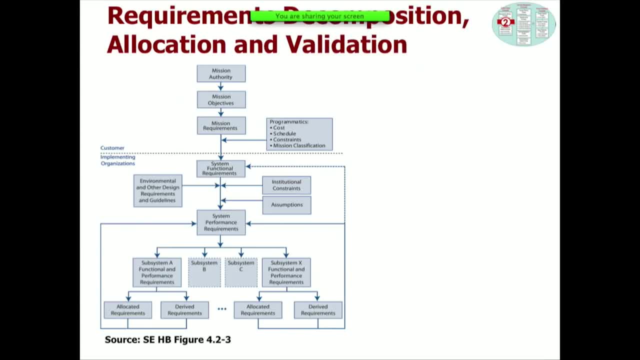 requirements. So allocated requirements are requirements that you choose. you choose to to um allocate and then derived requirements are calculated based on the they're dependent requirements, based on the allocated requirements, and I'll get into this into into in a minute. 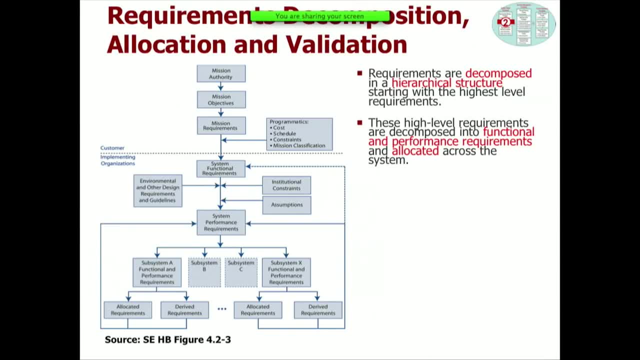 So requirements are hierarchical. we talked about this: uh functional and performance requirements are allocated, And then uh you choose to allocate, And then from these we can further decompose and derive uh requirements, And then the total set of these requirements needs to be uh verified and then validated. 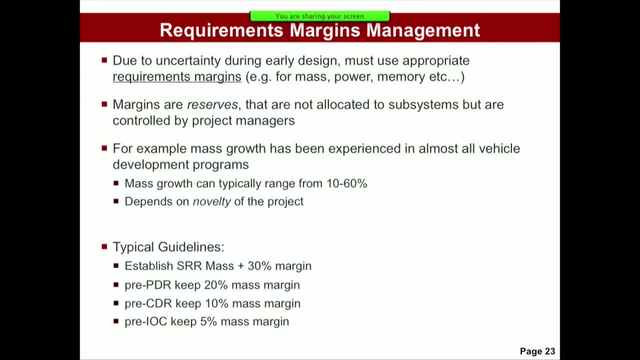 against the uh stakeholder expectations. Um so let me briefly talk about requirements, margins, management. So, because you don't know everything up front, there's uncertainty. we typically build in reserves into our requirements and those are called margins. So we put in margins for mass. 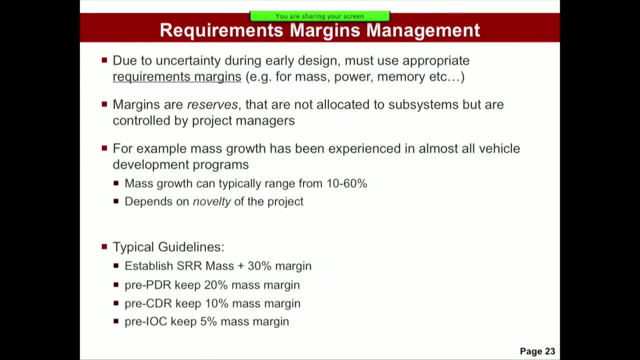 Power, maybe memory in computer systems. So margins are essentially reserves, uh, that are not allocated to particular subsystems but are controlled by the project managers or at the higher level. So the idea is that you write the requirement in a way that is a little bit more stringent. 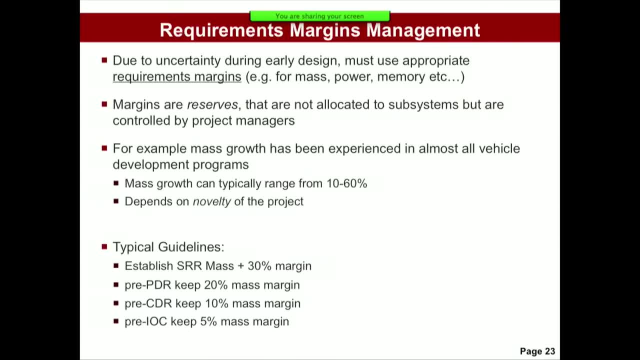 than it really needs to be. And then, by by being more stringent, you've built some reserve into the system to handle, you know, unexpected things. So I'll just give you the example with mass growth. You know this is very typical in aerospace vehicles. 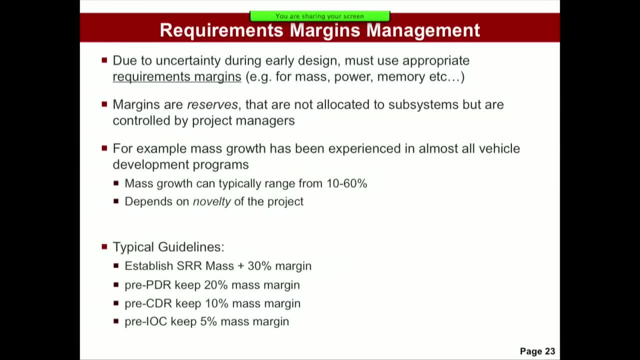 Uh, mass growth can range between, you know here, 10 to 60 percent. I'll show you some examples, And a lot of it depends on the novelty of the project. So a typical guideline specifically for mass margins is about 30 percent reserve at the. 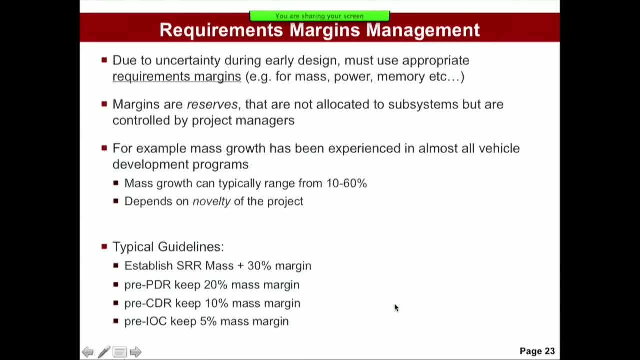 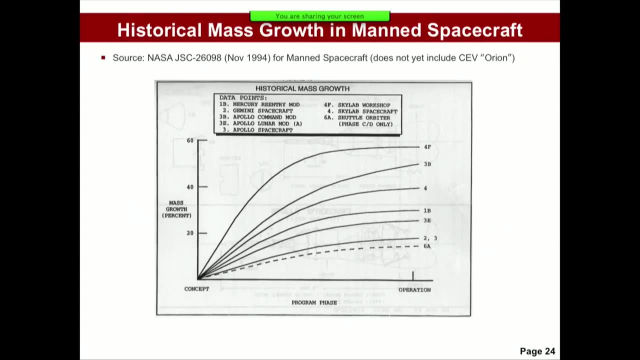 SRR, 20 percent PDR, 10 percent CDR and keep about 5 percent right before you operate the system. Uh, IOC is initial operating capability. So here's some historical data. Uh, this is for manned, uh, manned or crewed vehicles. 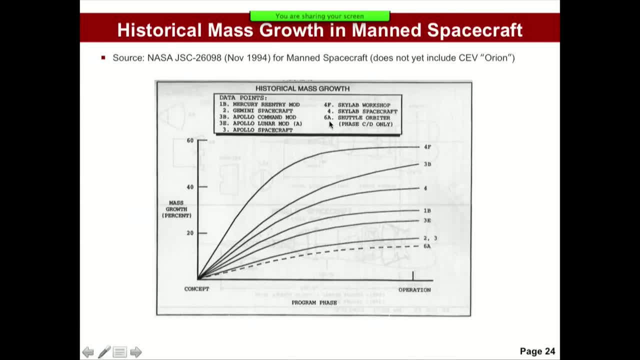 Uh, starting with Mercury, Gemini, Apollo Skylab and then the shuttle, you can see the mass growth. uh, from the concept stage, you know which is phase A or pre-phase A, all the way to operations. you know between 10 and 60 percent. 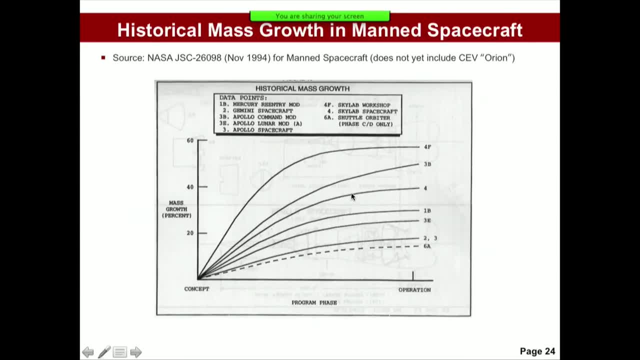 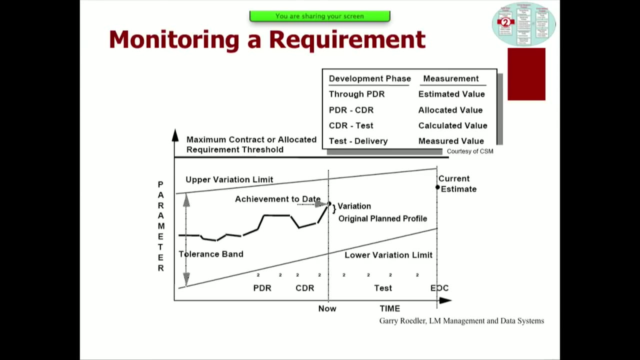 The new uh Orion spacecraft. It's not yet included on this chart. So what you do is you essentially write the requirement, knowing that this growth will happen during the design process. That's the basic idea of of margins. And then the next idea is that uh, you monitor the satisfaction of the requirement during 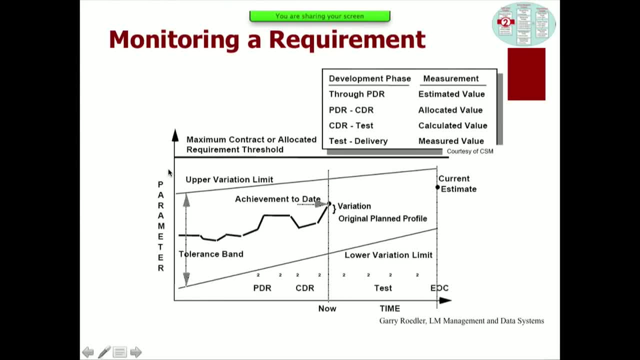 the design process. And so let's say you have in a performance requirement, you say that the system shall not emit more than X number of NOX right Uh emission, Or the system shall not be heavier than such and such. That's on the Y axis here. 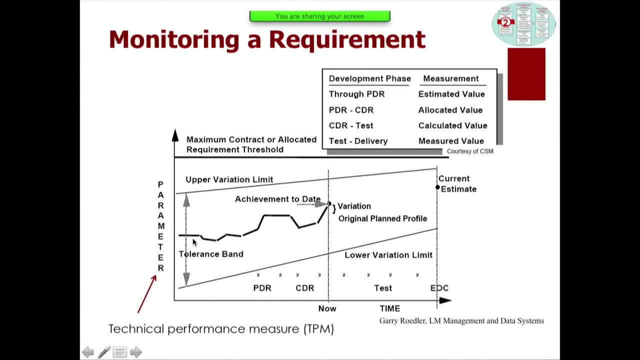 That's your technical performance measure. And then you move through time and you know, as the design gets more detailed, usually it gets heavier, you add more things, um, and you monitor that And then you have your, your final current estimate of where you will be at the end of. 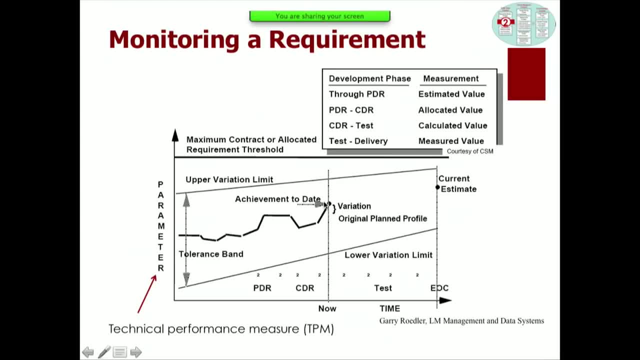 the project And, as you do that, your your limits, your reserves, your margins, and here there's an upper and lower margin. The lower margin shown is going to be um narrowing down, Um. I'll give you a quick example: uh, when I was at McDonnell Douglas, uh, the F-18 EF. 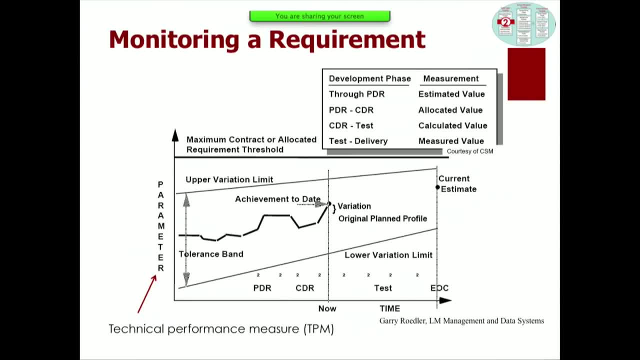 version. the Super Hornet was being developed And the key thing there was G-T-O-W, G-T-O-W gross takeoff weight. It's basically the weight of the airplane with crew fuel, any uh any payloads all. 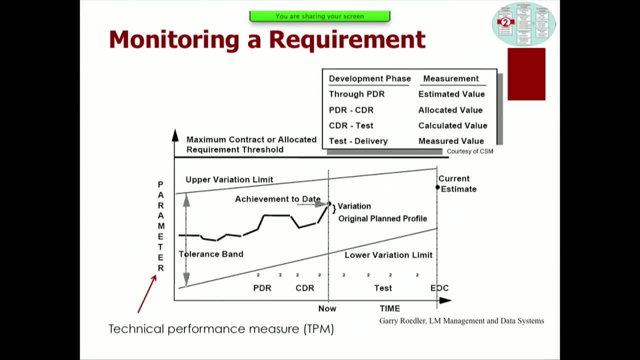 in The the gross takeoff weight of the airplane is very important because it you know, it determines the range, it determines a lot of things And the number not to exceed, number which is um shown here on this chart as the maximum. 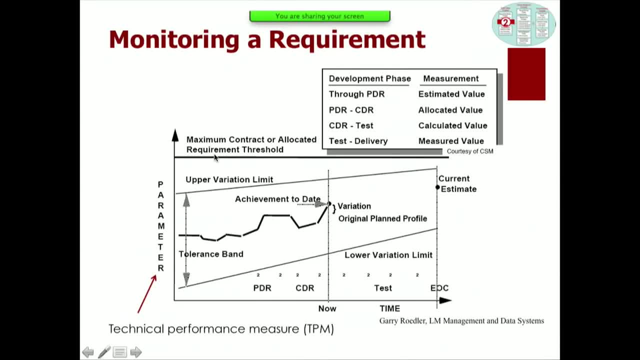 contract or or allocated requirements. threshold is was contractually specified. Not only that, but there were penalties, financial penalties, associated with every kilogram that that you would be over. So this was a big deal. And they had a huge wall chart in the hallway, the main hallway of the engineering building. 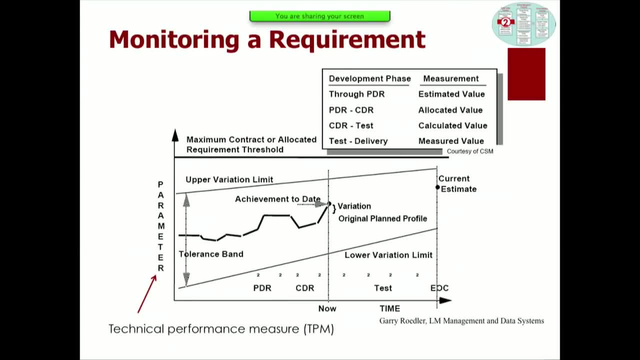 And every day somebody would actually manually update that day's best estimate of what the gross takeoff weight of the airplane would be. And it was like a Brownian motion thing and as soon as you hit some critical threshold you would see there'd be people would would come together and say we gotta take weight. 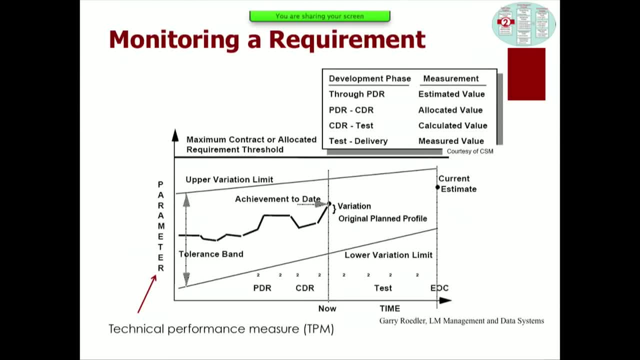 out of the airplane somehow again right and then and then basically try to get the design to comply with all the requirements, And you can't do that with too many of the requirements, but the most important technical performance measures. that's what you do. 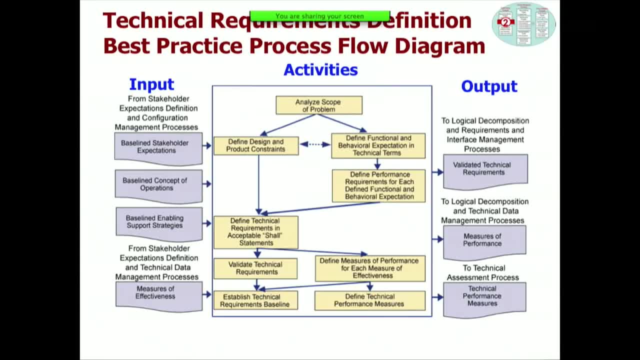 It's a big deal Um. so here's the uh, the flow chart, basically for requirements. I'm not gonna go through this in detail, but the basic idea is the inputs come from the stakeholder expectations, the stakeholder uh work we talked about last time. 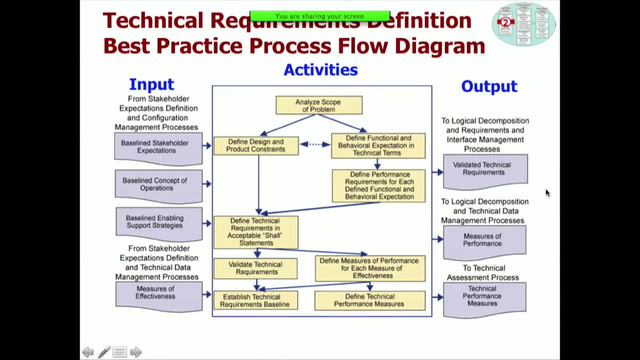 You go through the requirements definition process And out comes a value. It's a value, It's a validated set of technical requirements, measures of performance that you can measure, and then these technical performance measures that you can then uh, track and validate. 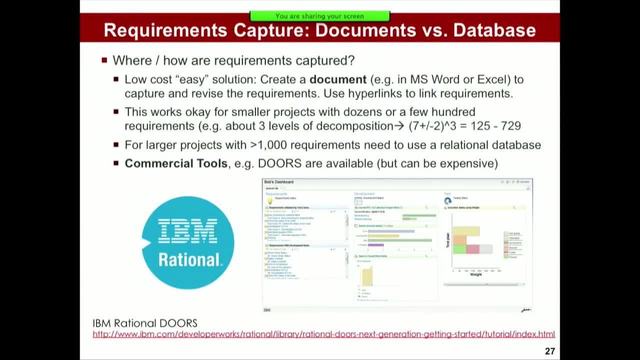 against later. Um, here's a question that I often get asked. Well, okay, so we write these requirements, You guys write them on paper or your tablet, but how do these requirements actually get, uh, recorded, right and managed? 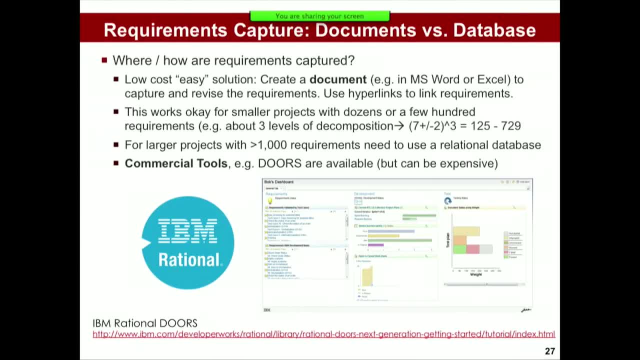 So there's, I would say there's sort of two: There's the low cost And then there's sort of the- uh, the cost, And then there's the, the professional version of doing this. The easy way to do it is you just write them, you capture them in a document. 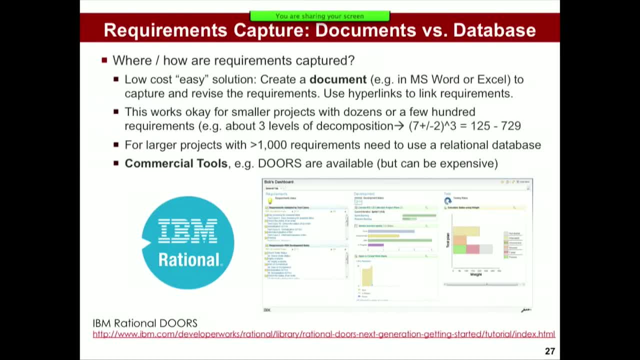 So that means you know Microsoft Word, Excel, you know Google Docs. uh, just a document, a well-written, organized document, And then you capture and revise your requirements, And the one thing I strongly recommend is using hyperlinks to link requirements. 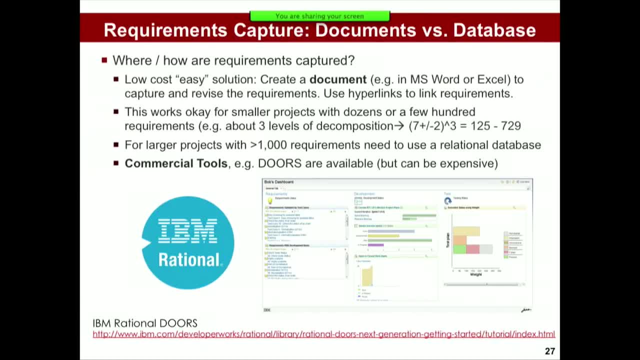 And that this is the idea that every uh, every requirement has to be uh, a, a, a. every requirement has to be linked to some other requirement. So if it's a low-level requirement, you want to ask: well, where does that come from? 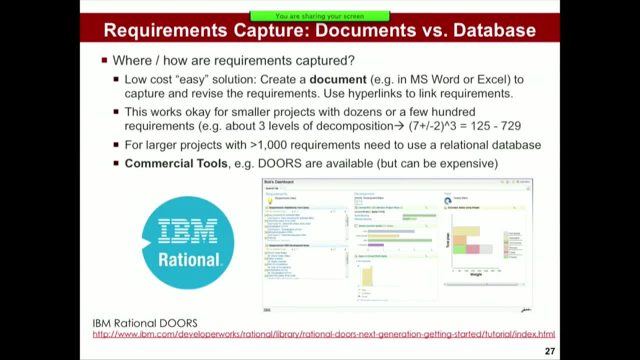 Why did we write that requirement? Well, it has a parent requirement, So you want to have a hyperlink there to get you from one to the other, And I have a a little example for that: Um and uh- and I think this is okay for smaller projects- uh, where you have dozens. 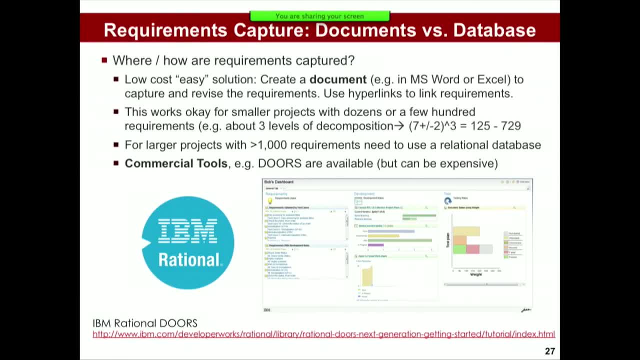 or a few hundred requirements. right, And This is my, my rule of thumb for this. Do you remember the magic number seven? So two we talked last time. you know where does the world of really complex systems start? And the argument was: well, if you need more than three levels of decomposition, what? 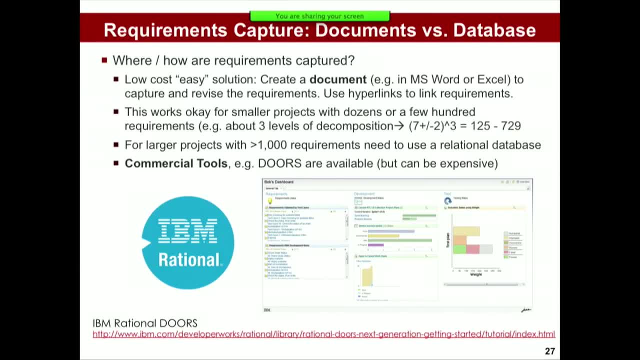 what does that mean? Well, seven plus or minus two to the third power is somewhere between 125 and 729,. right So if you're sort of in that world, or or fewer? right if you're a few hundred, a few. 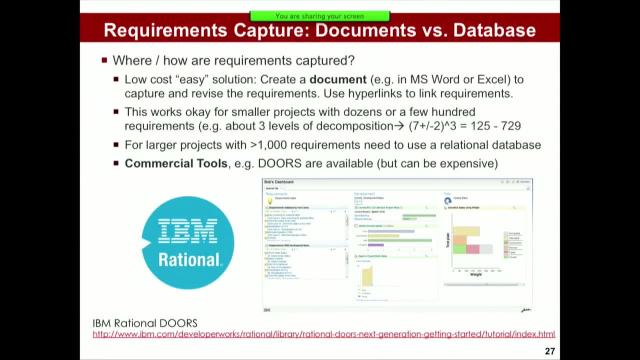 dozen or a few hundred requirements, Kind of what we have in CanSat. it's okay to do it this way, right, It's still going to be, you know, a lot of requirements and you have to do a good job, but you can do it that way if you have more than that. 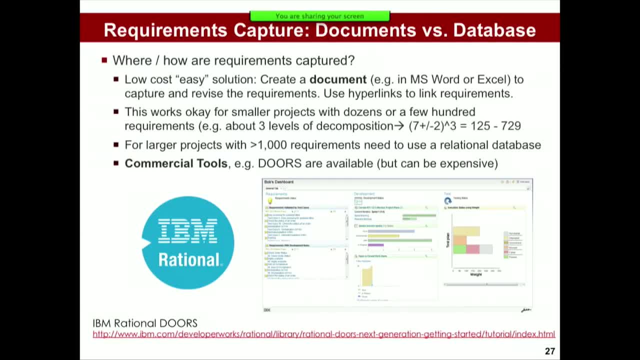 And that typically means more than a thousand requirements to handle, And there are big projects that have, you know, 5,000, 10,000 requirements. There is no way you can manage that effectively in a in a kind of document based way. 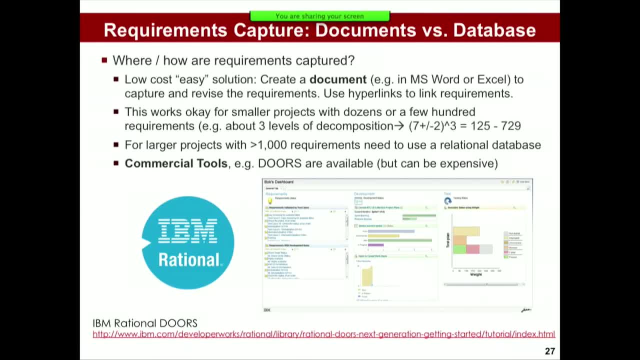 So what you need, then, is a data. You basically capture these requirements in a relational database where that allows you to link each requirement to other requirements, And so I'm not- this is not meant as an advertisement- but one of the most heavily used requirements. 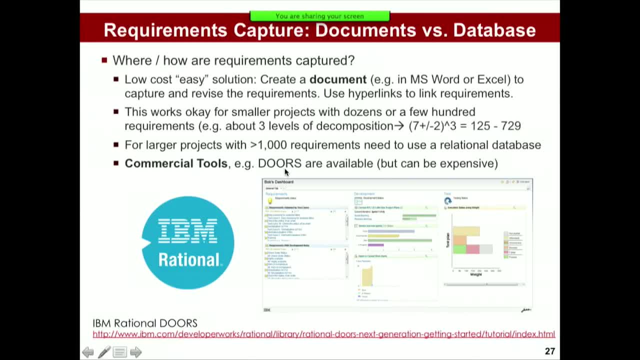 tools out there is called Doors, And this was relatively recently bought by IBM. This was a separate company. It was bought by IBM and included in a suite of software tools called IBM, IBM Rational for system development. And so Doors allows you. it's a database, relational database. 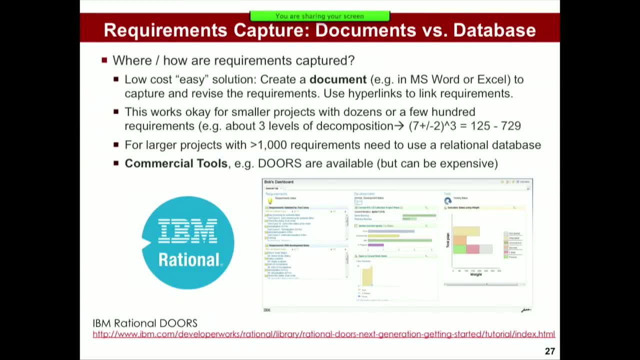 It allows you to write requirements, share requirements, and the latest version of Doors is actually web-based, So you can have people you know in India, in Europe, in the US. you're co-developing a system. You can all write requirements and manage them on this common database, right? 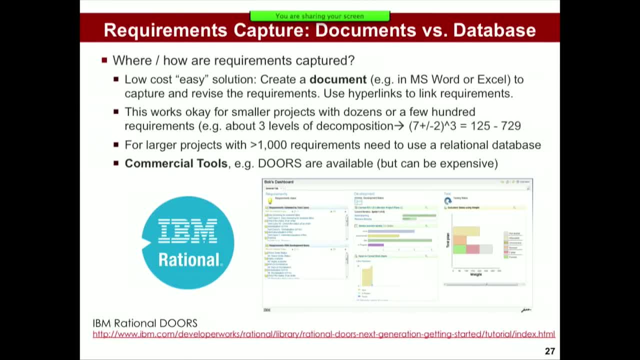 Because if you have a document very quickly, it's going to be confusing, as what's the latest version, Who has you know the latest update Version? management becomes a nightmare. So, just so you're aware of this, we're not going to be using Doors in this class. 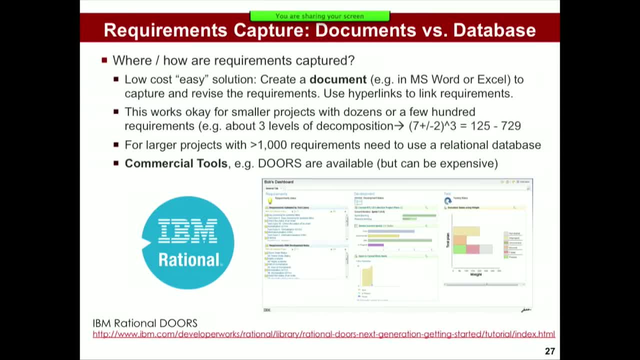 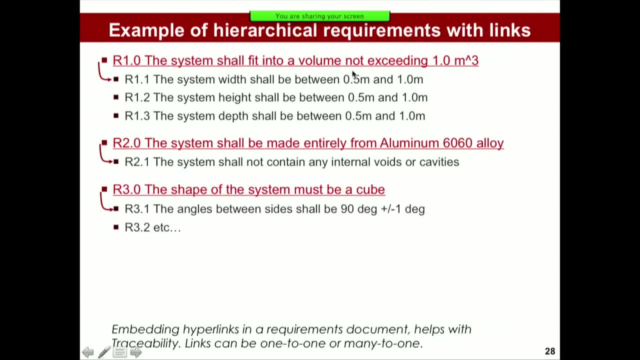 We'll just do it document-based. but you know the rule of thumb here is more than a thousand requirements, You've got to go to some professional solution. So here's a very sort of trivial example of hierarchical requirements with links. Requirement one: the system shall fit into a volume not exceeding one cubic meter. 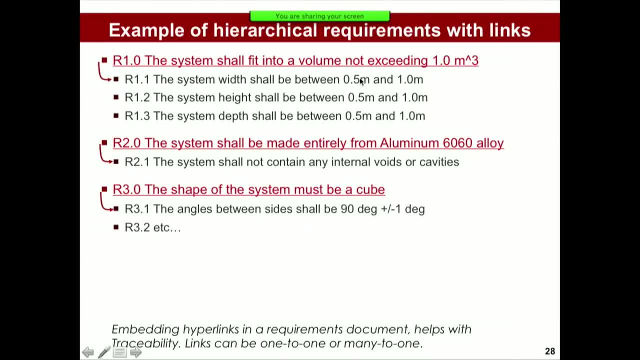 And then we have sub-requirements. The system's width shall not exceed one cubic meter. The length shall be between 0.5 and one meter. The height, the depth. The system shall be made entirely from aluminum 60-60 alloy. 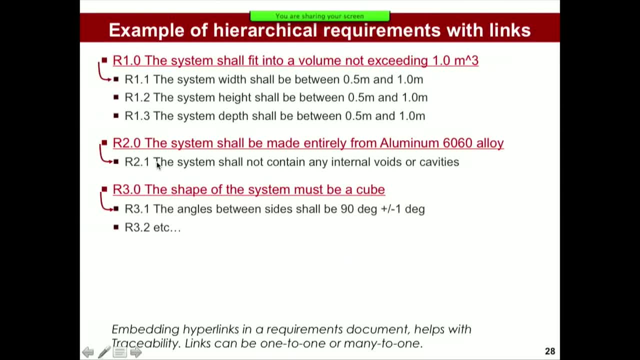 A sub-requirement here is: the system shall not contain any internal voids or cavities. Requirement three: the shape of the system must be a cube, And then a sub-requirement: the angles between the sides shall be 90 degrees plus or minus. 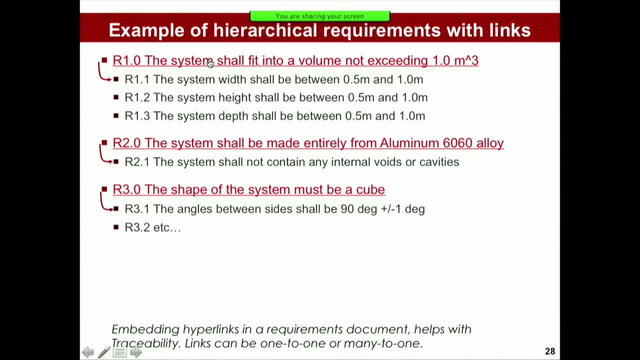 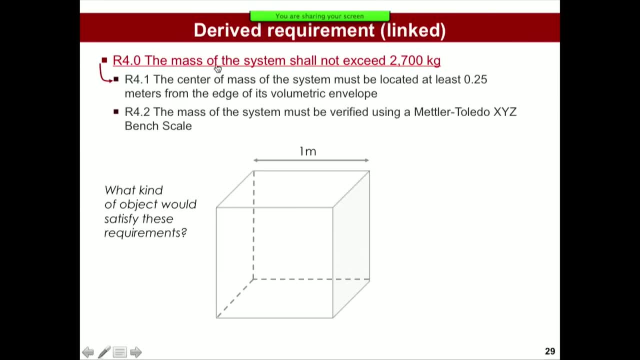 one degree And so- and I did this here just in the slides, But if you click on this It'll actually transport you to another requirement. This is requirement four: The mass of the system shall not exceed 2,700 kilograms. right, 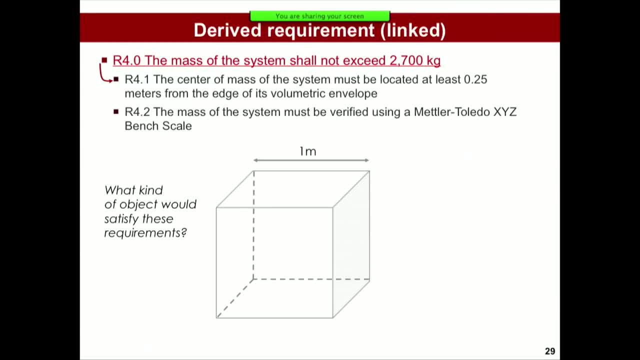 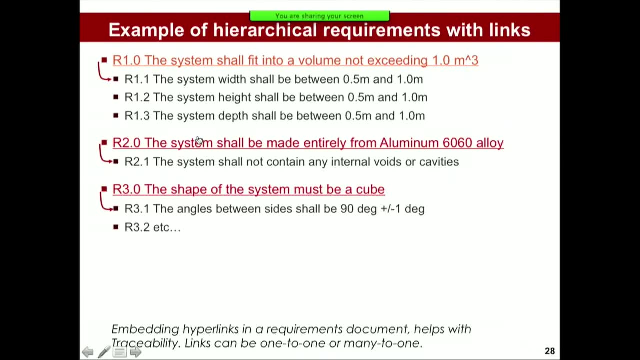 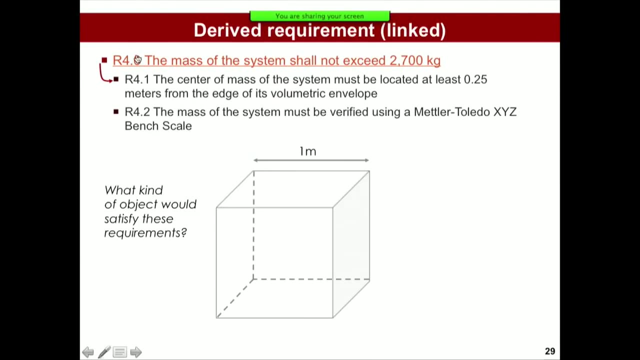 Aluminum has a density of about 2,700 kilograms per cubic meter. So if I click back, it transports me back to the earlier requirement, right? So the fact that it's made of aluminum and the volume cannot exceed one cubic meter. then this requirement four. 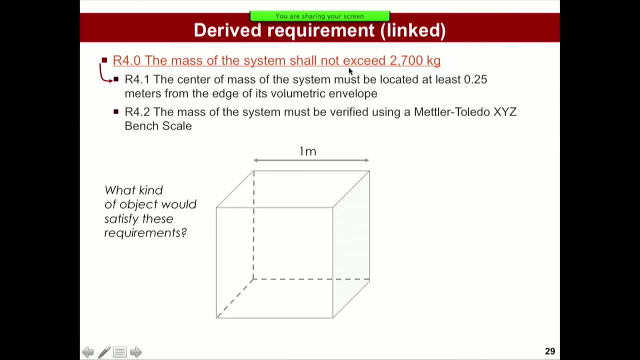 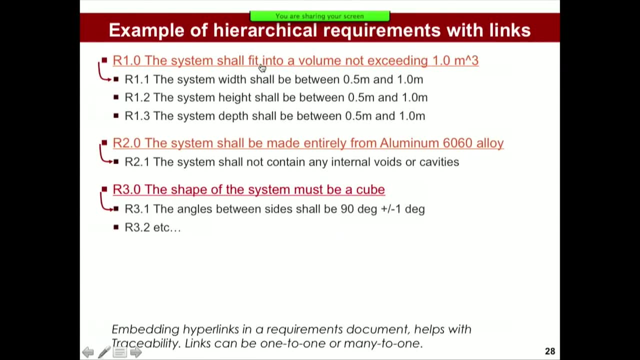 The mass shall not exceed it. It's not independent requirement. It's a dependent or derived requirement based on the first two And therefore they're linked. Do you see how this works? And to really manage requirements well and then link them, use these hyperlinks. 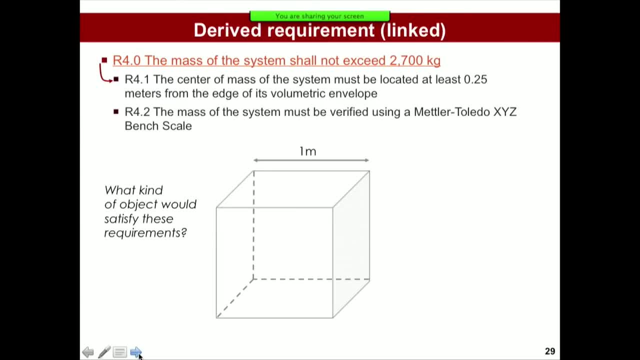 It's very, very effective. So what would be an object that satisfies these requirements? So here's our one cubic meter envelope, So an aluminum cube with a side length of 60 centimeters. This volume and this mass, This mass would satisfy the requirements. 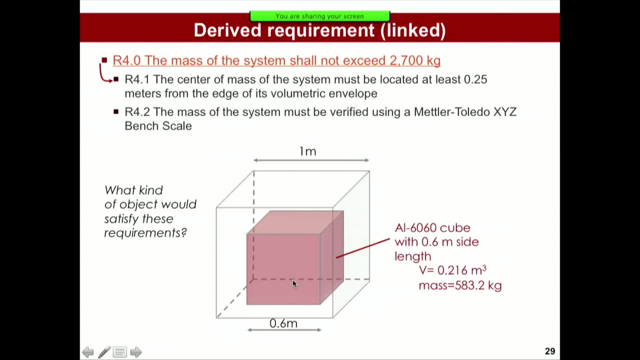 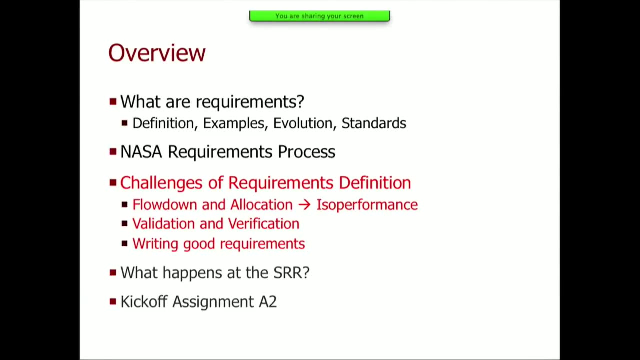 It's not the only thing. There's a lot of other geometries that would satisfy it, But this particular instantiation would satisfy these requirements. OK, So that's the idea of hierarchical requirements, linking them through hyperlinks. OK, so let me talk briefly about the challenges now of requirements definition. 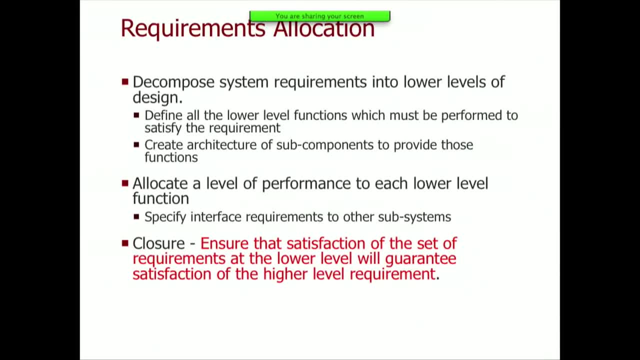 And this is not easy. There's a lot of challenges. The first one is There's the idea of requirements allocation, this decomposition and flowing requirements to lower levels, And the idea is that whatever requirements you derive at a lower level, if you satisfy. 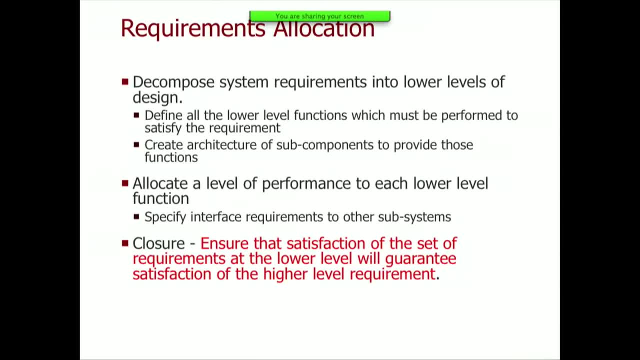 the lower level requirements. that should guarantee that you then automatically satisfy the higher level requirement, right from which the lower level requirements were derived. That's the basic idea of requirements allocation, And so the way you can think of this graphically is: 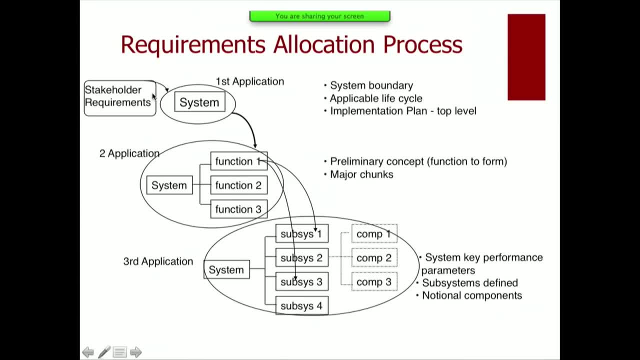 We start at the high level. Here's our stakeholders right Stakeholder needs requirements. This is level zero. You set the system boundary, What's the lifecycle, And then we apply it. That's our first application. And then we apply it by decomposing the system into its functions. 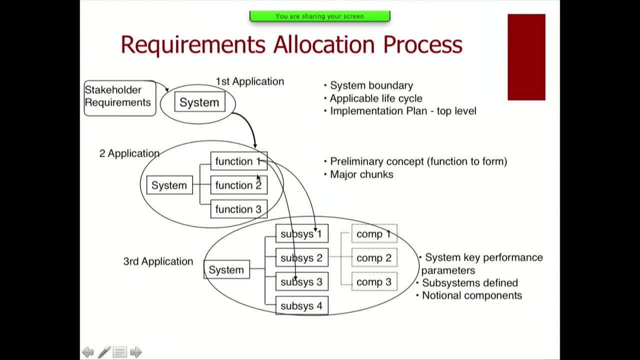 And so that's the second application. And then you say, well, how do these, How will these functions be carried out? So we define subsystems And essentially then the subsystem requirements are derived from the functional requirements and you put numbers: see key system. 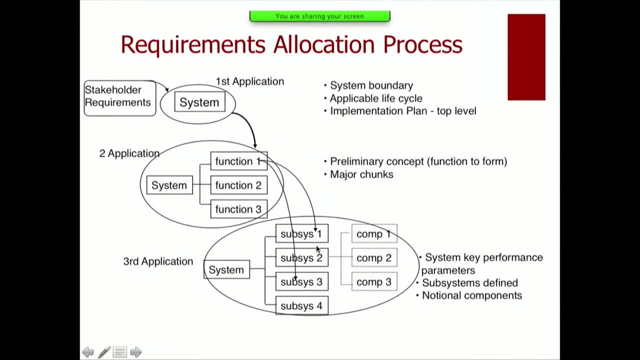 performance parameters behind these and, depending on the complexity of the system, you may have to go multiple layers down. but that's the basic requirements. allocation process. um, and i think i said this already, it's difficult to do and stay solution neutral. uh, the deeper you go into this, 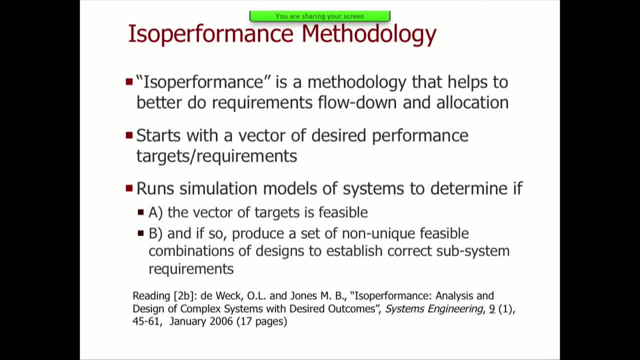 let me briefly mention, uh, this- this will not be, we will not sort of test you on this, but i want to make you aware of this- um a methodology called iso performance, and that's that was actually the the topic of my, my dissertation. um, how do you, how do you do, how do you allocate requirements? 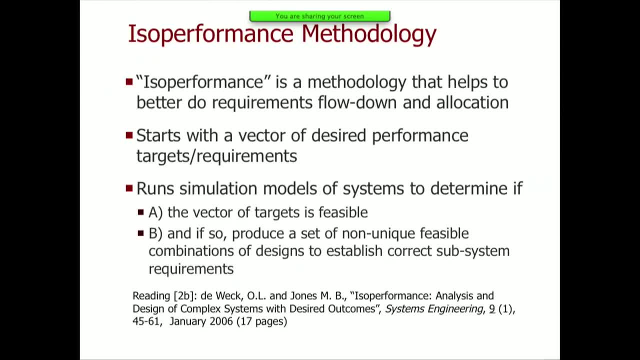 to lower level parameters or systems when the higher level requirement is is defined is clear. so the the idea is that you have a vector of desired performance requirements and you want to understand. first of all, you understand: are those requirements feasible? and if they are feasible, it usually means there's more than one way. 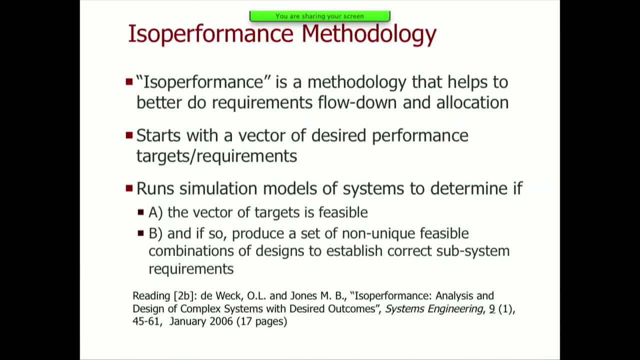 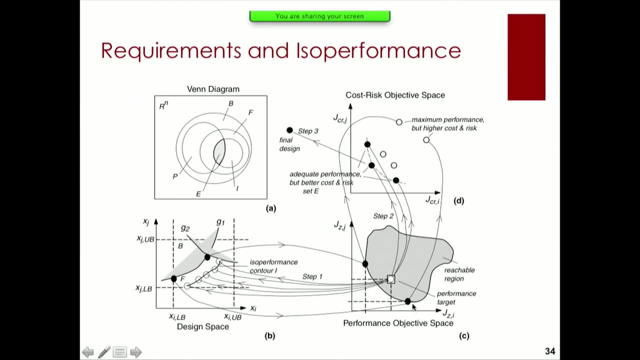 that these requirements could be satisfied, that the higher level requirements could be satisfied. so find different, non-unique feasible combinations to satisfy the higher level requirement. and so this is one of the readings. very quickly, we have our design space, we have our objective space and then we have this cost risk objective space. and so the idea is that in the performance space, 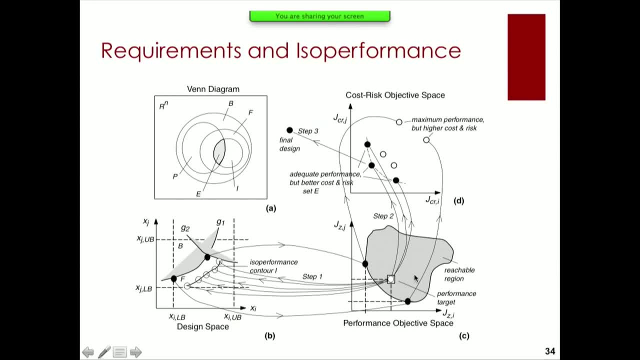 you have the shall statements, you shall perform at that level, and that's this point here, that's your performance target, and if it's in this, in this gray area, it's actually feasible and it usually means there's more than one way to do it. so if you can, then map. 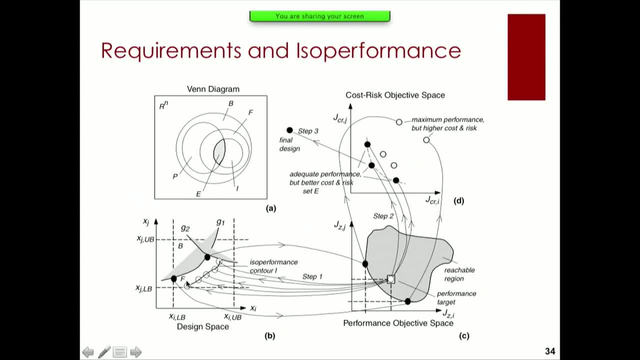 backwards to the design space. these points here are all iso performance, meaning they're all. they all satisfy and provide this level of performance, but they do it in different ways and and then, in order to select a final design or a final requirement set you want to look at. 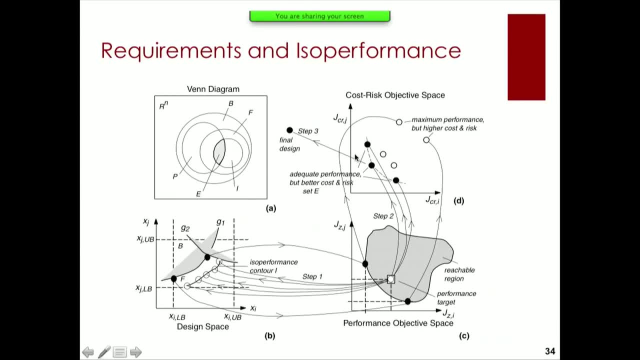 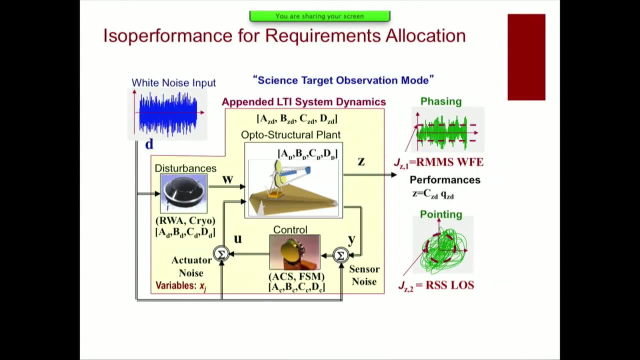 other objectives. this is where the should statements come in, and these are typically cost and risk related objectives. so let me give you um, this sounds pretty abstract and theoretical. let me give you a very specific example. this was my main case study: a space telescope. this is the. 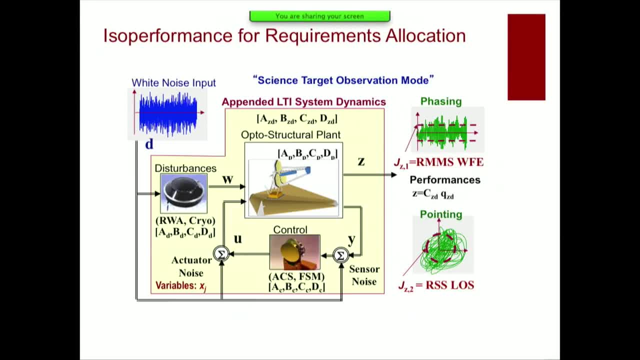 actually this has now become. the james webb space telescope hasn't launched yet. this is 20 years ago. right, we've been working on the james webb for a long time, but if it works, it'll be exciting because it's going to get us very, very close to the big bang. right, that's what james webb? 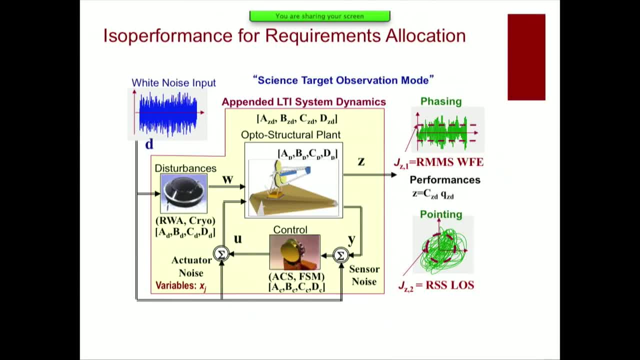 will look in the highly redshifted infrared to really see the formation of the earliest proto-galaxies in the universe. so if this works it'll be very exciting. so, essentially a model of the, the spacecraft, this is a precursor to the james webb and the big thing. 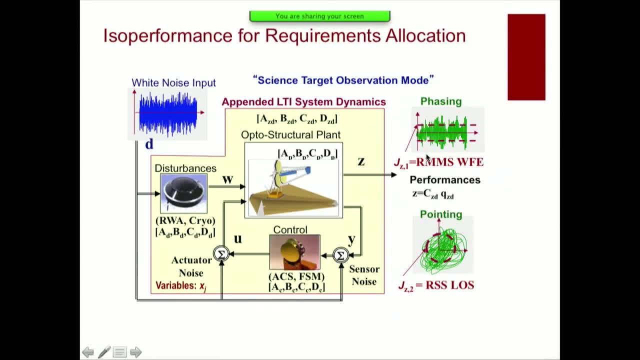 you need to do is you need to point. you need to point and be very, very stable for a long time to take in these very, very faint images. so we have wavefront error phasing requirements and then we have these pointing requirements. we've got to point very stably and in order to achieve this, 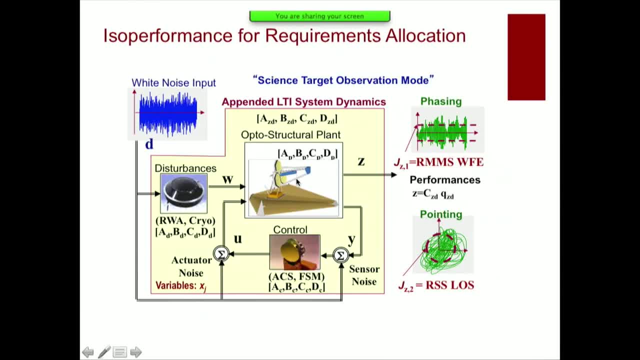 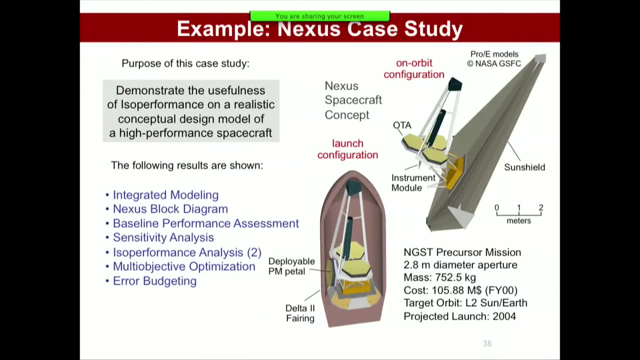 optical pointing performance. we have the dynamic structure of the, the spacecraft, we have reaction wheels, we have controllers and- and there's noise- different kinds of noise sources- that are trying to basically prevent us from pointing with this precision so very quickly. this is what this nexus precursor spacecraft looks like in the 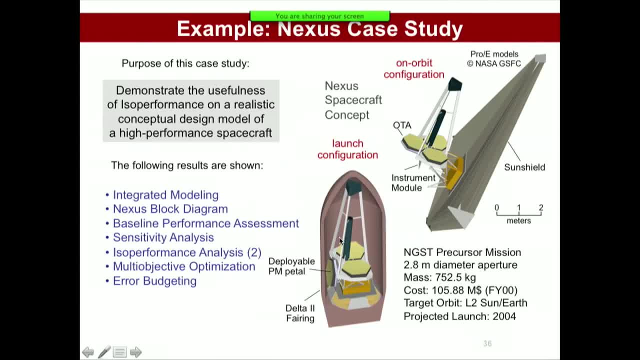 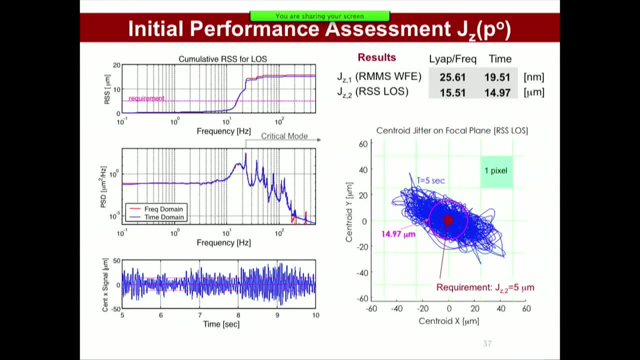 deployed configuration here on the upper right in the stowed configuration, initial performance. this is really trying to find the requirements for deriving the requirements for the structure, for the optics, for the controller, knowing that this is the point, if you want to have this science happen, you've got to point with that precision that is known. so let's. 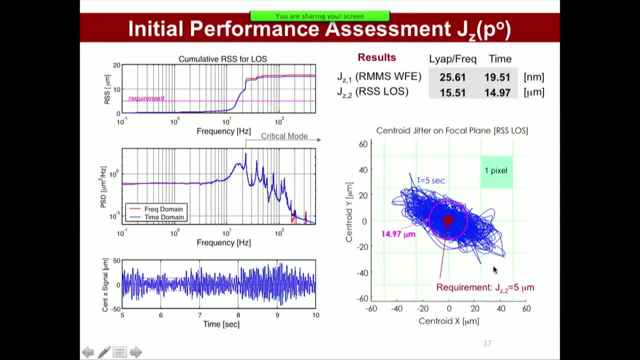 flow that down. and so if we look at the pointing, for example, here on the right, this, this kind of fuzzy furball, what does that represent? that's a time domain simulation of the centroid of the image. right, the telescope is now observing a part of the the sky, trying to get you know these early proto. 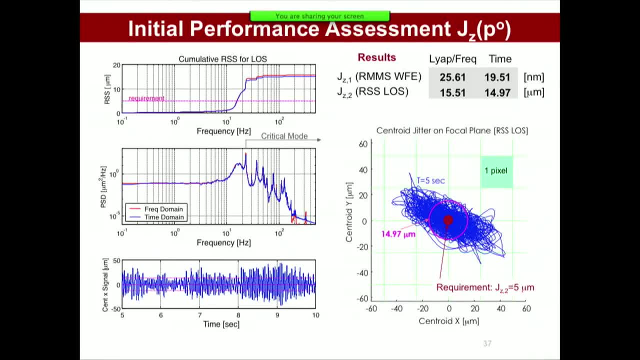 galaxies and it's- you know it's, it's flexible, it's a very lightweight telescope. it has these reaction wheels are turning trying to keep it stable. we have electronic sources of noise. so the blue fur ball here predicts that we would not meet the requirements. this is some initial 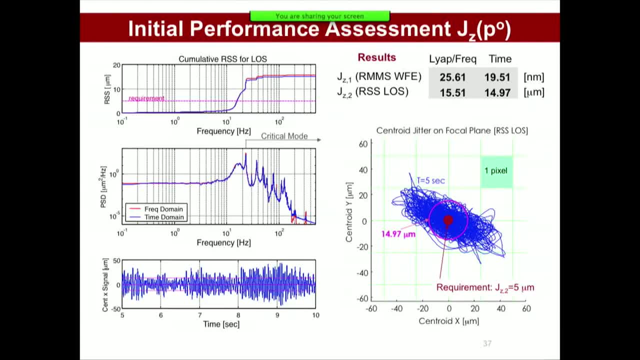 design some initial set of requirements. we need to find a way to get down to the point of the telescope. so this is about 15 microns root mean square error. so it's about three times worse than what we need to achieve and the requirement is we need to get down to five. 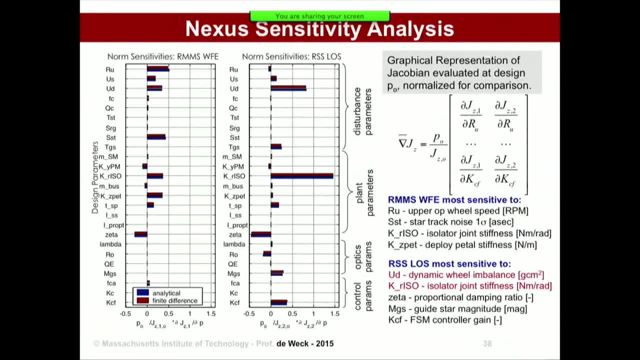 microns of pointing or jitter precision. so how do we do this? so what iso performance does is it looks at the sensitivities in the system. what are all the things that influence the pointing performance of the telescope? and you can see here these are the two key performance measures of the 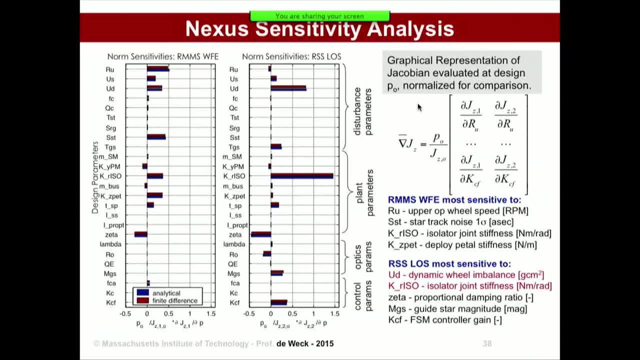 the left way, front error, and then line of sight, and the bars essentially tell you what are the really sensitive parameters that drive performance. so disturbance parameters, plant structural parameters, optics, and then control. so it's really multidisciplinary and what's neat about it is you can, if you know. 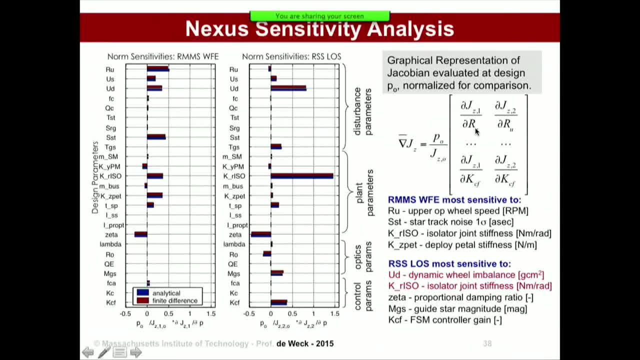 these sensitivities, you can essentially calculate the Jacobian matrix. the Jacobian matrix is essentially the partial derivative of your performance right, which is your higher level requirement with respect to these lower level parameters or requirements, and you can then find, using this, essentially the null space of the Jacobian matrix. that will tell you how do you move in that. 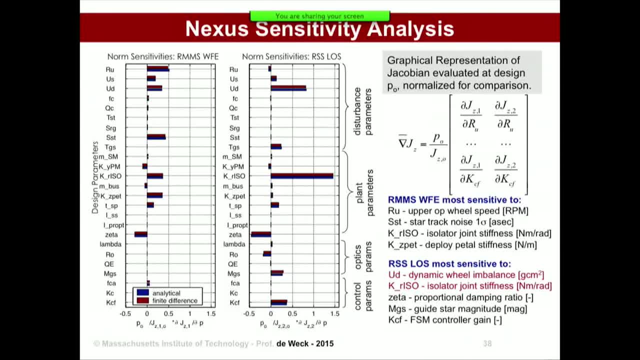 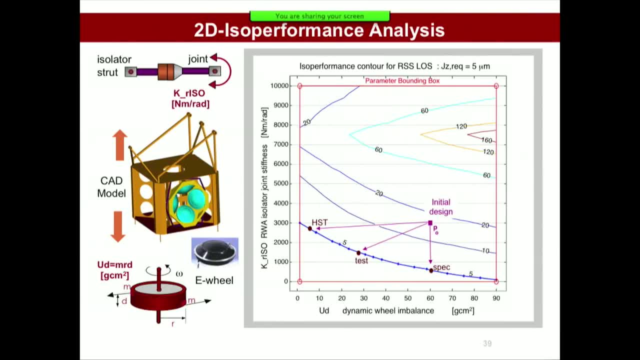 space to keep the performance fix at the requirement level. let me explain this just using two parameters. okay, and this was a big deal in the Hubble Space Telescope. so the two parameters I'm going to use is KR, ISO and UD, the dynamic wheel imbalance. so these spacecraft have 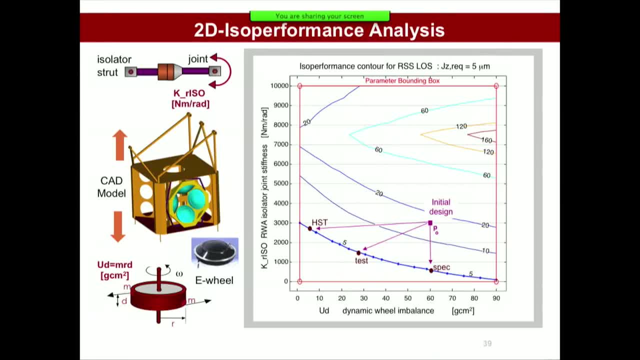 reaction wheels that are turning to point the spacecraft and counteract any momentum that you get from, for example, from solar pressures. so, UD, is the amount of imbalance that you have in these wheels right? if you have imbalance, that will cause chatter, it will cost torques which will cause that jitter, and then 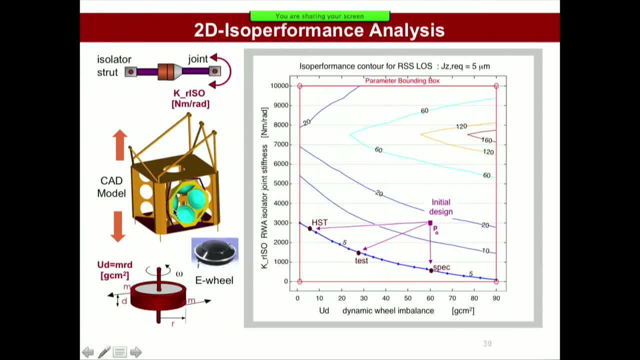 KR ISO is so, whose simpler number is 14. what will hp will charge? and so at this point, certainly, this baker selected- this is a geworden izing thing that it was still called to be till table, 여자, and then the problem really is to be okay. so from here let's come up to the next slide. this is a data. 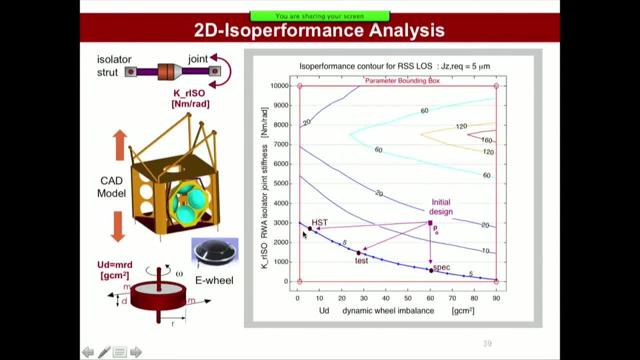 velocity data entry and these ISLE models extracted holon Davos' tables and durch fooled elevate pin. now partnership房 z listening. as we can see is that due to the error released you, We could go over here. This is labeled as HST. 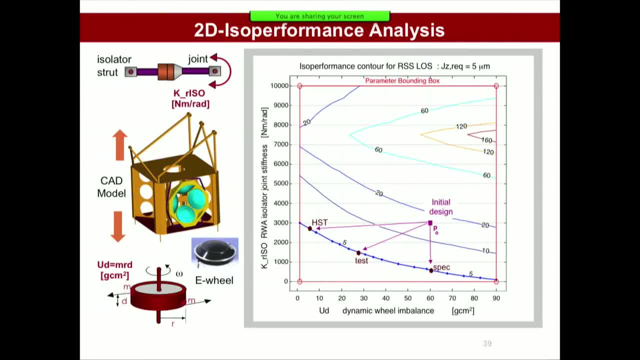 That's what Hubble Space Telescope did. The Hubble Space Telescope basically went for ultra, ultra, ultra quiet reaction wheels, Very, very low dynamic imbalance. So, Marissa, you talked about, you know, buying sensors from a supplier and putting them in. 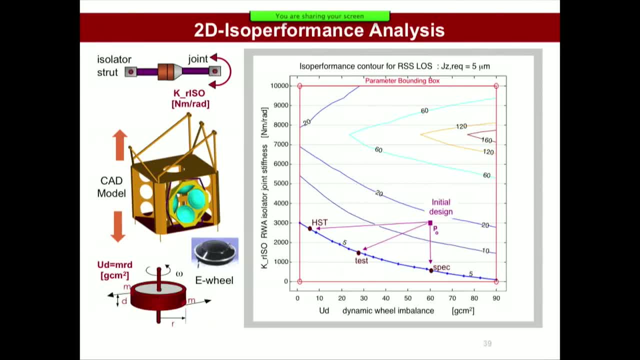 There's companies that really specialize in making reaction wheels and things like that. So if you're going to go for this point here, let me point that out again so you guys can see it at EPFL, If you're going to go, if you're going to derive and allocate this requirement, 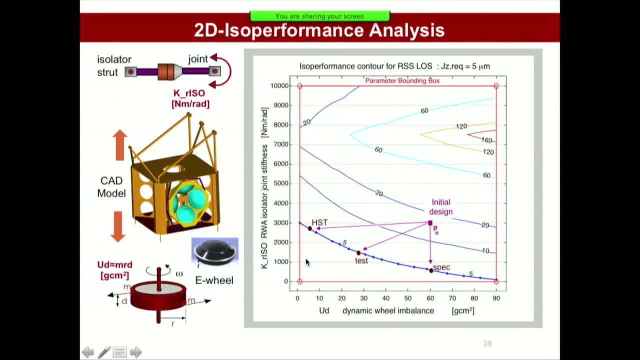 it means you put a lot of pressure on your supplier to achieve that level of dynamic wheel imbalance. If they can do it, that's great, but it could be very expensive. But it makes your job easier, right as the spacecraft integrator. 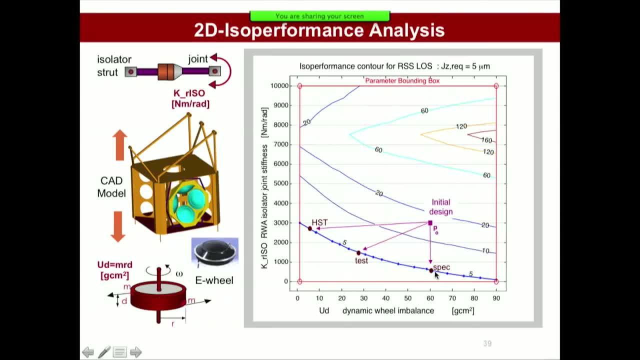 Or you could go straight down this point here called C, So you're essentially tolerating a noisier reaction wheel, but then you need a very, very soft, very capable isolation stage, Very soft isolator. What's the disadvantage of having very soft isolation? 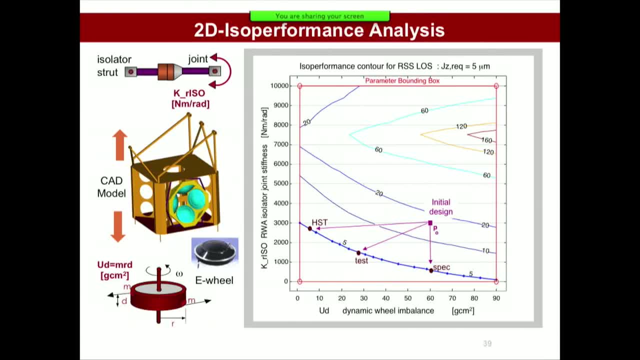 What do you think is the big issue there? So the launch: you probably have to lock it down during launch. You have big displacements. You need, you need- if you have a very soft isolation stage, you need volume, Because the isolator is going to move a lot right. 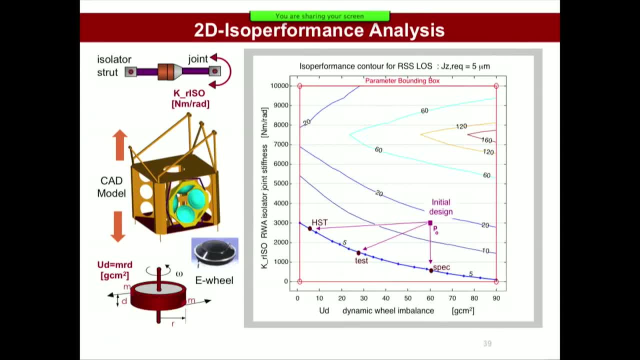 And you may not have that that volume, Or you could do a little bit of each. So this test point here means we're going to have quieter wheels, but not ultra quiet, And we're going to have a soft isolator, but we have the right combination of the two. 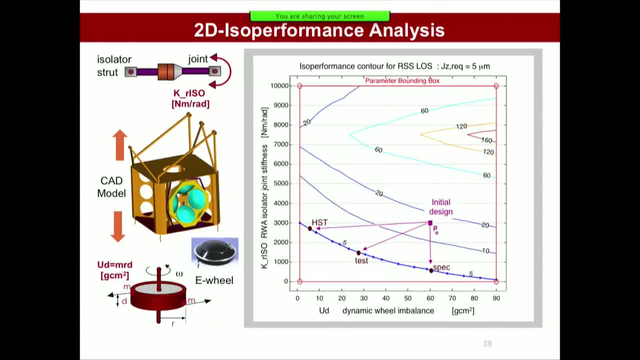 And we're going to go for that, that point there. So now, if you go for that point, you're going to satisfy your pointing requirement, but you've allocated the lower level requirement in this case to the isolation stage and the dynamic wheel imbalance in a kind of balanced way. 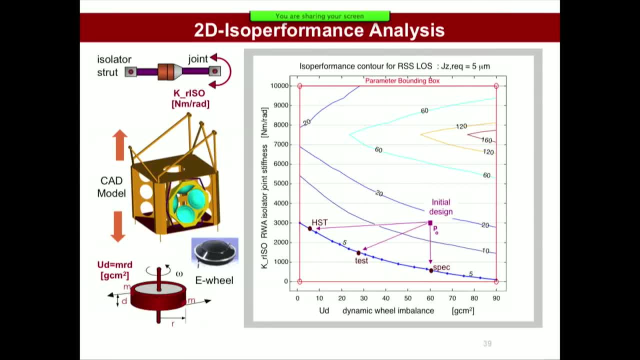 So everybody's job is roughly equally difficult. That's the sort of idea here. Yes, Does this model assume that all of these variables are then independent And, I guess, kind of continuous, in terms of you know, you can incrementally work better? 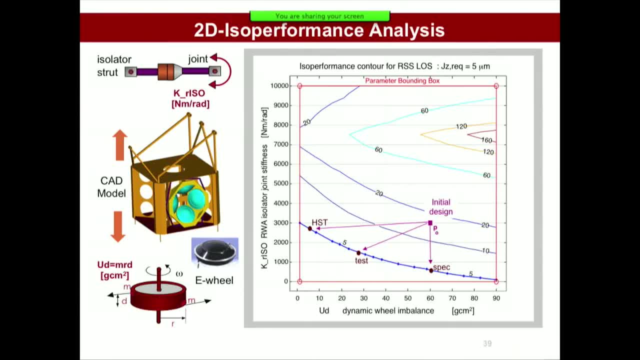 So they're not independent. They're not independent in the sense that they're coupled through the performance of the system, But you can choose. the assumption is you can choose these independently, But they're coupled because you need to achieve that requirement. And, yes, in this case they're continuous. but you can think of this as discrete as well. 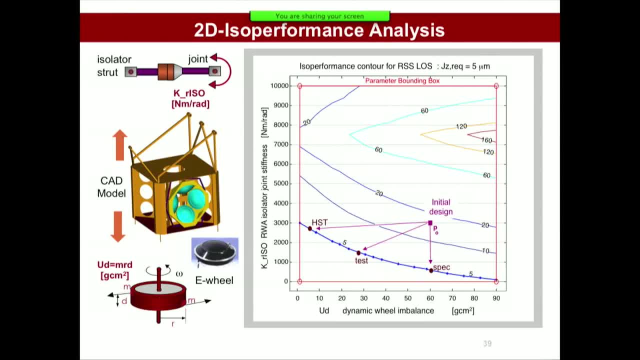 So, for example, the reaction wheels could be you picking from a catalog, for example, Right, In which case now you're really picking specifications for components that are off the shelf, Right? Okay, So let me. I'm going to skip here for time. 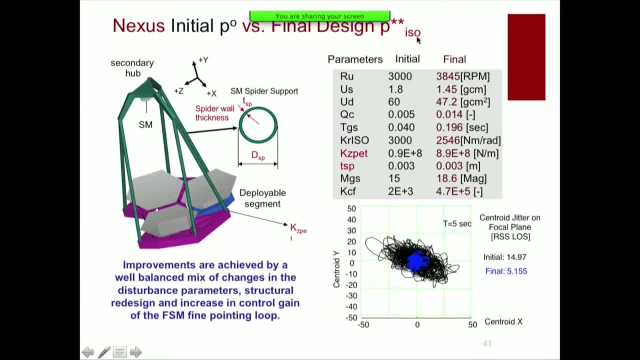 So basically, following this isoperformance process, you can go from some initial requirements, derived requirements that are infeasible to, and in blue here I'm showing you the results of this. It's very close to five. There's some numerical tolerance here. 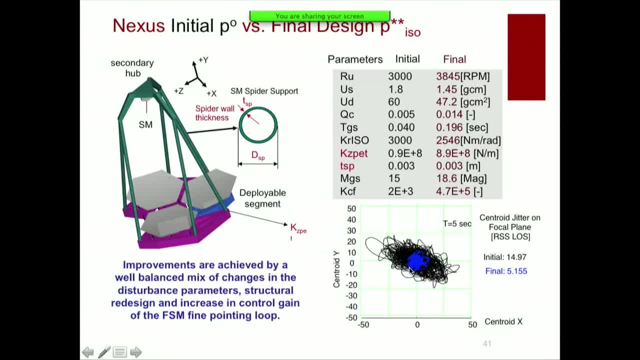 But by essentially rebalancing the requirements within the system we're achieving the higher level requirement, but in a way that it distributes sort of the challenge equitably across subsystems. Does that make sense at EPFL? Did you guys follow this? 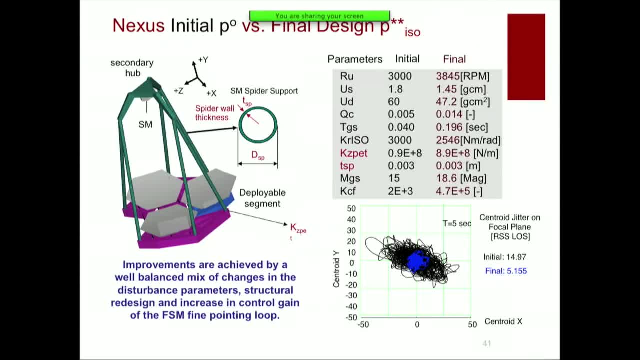 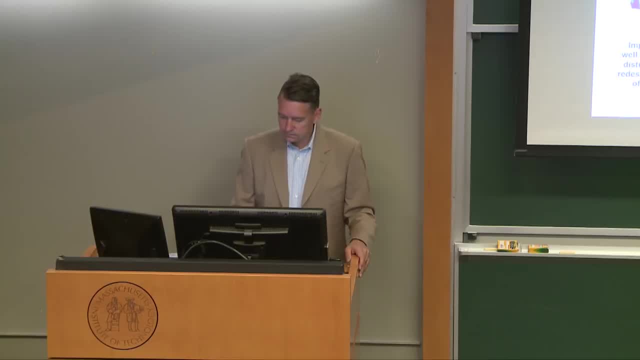 I know this was a bit fast, but that's the basic idea of isoperformance. Any questions on your side? No thanks, Yes, maybe I have one. So, given that you have different requirements and you probably have isoperformance lines for each one, 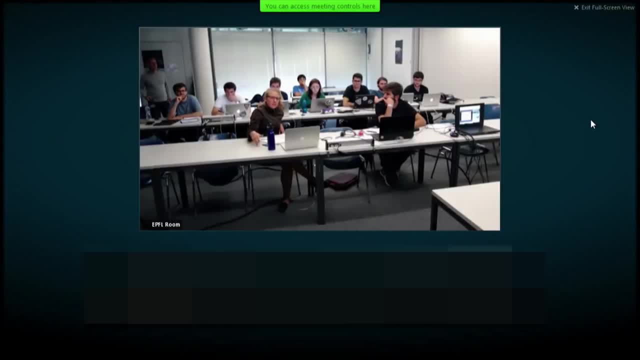 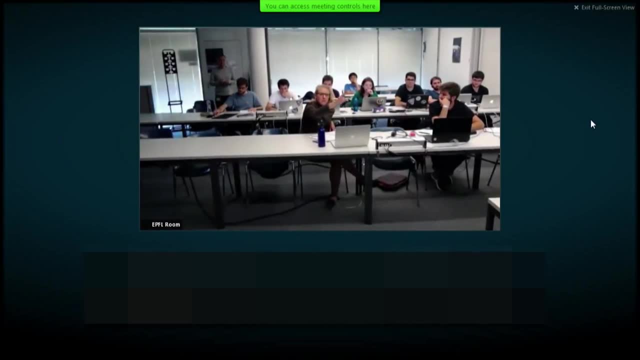 is there a way that would kind of integrate all those lines that you could see feasible in each of those You know you don't want? maybe it's a little bit soft, but maybe there's another requirement where that's a really sticky point. 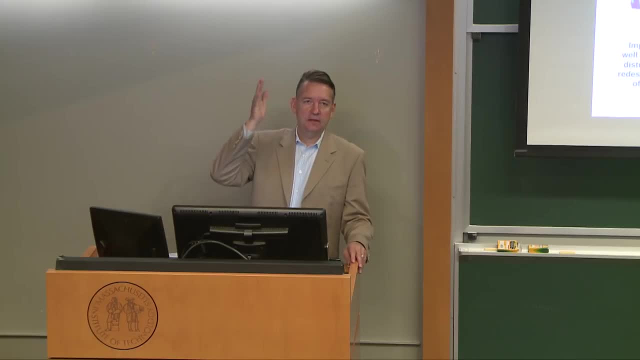 Can't hear you. We don't hear you. Sorry, guys ran out of battery here. Can you hear me again? Can you hear me? Yeah, So the question was: well, if you have multiple of these performance isoperformance lines, 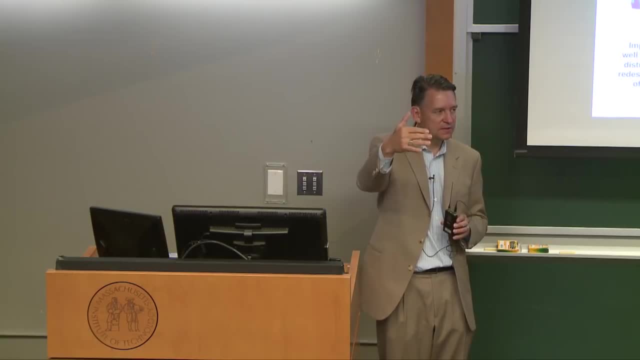 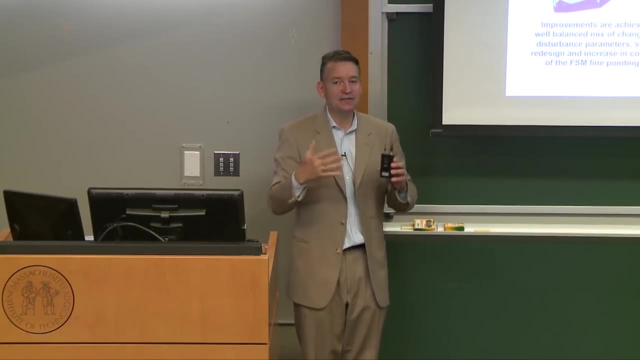 that's exactly right. If you have a vector of high-level requirements, you're going to have isoperformance surfaces, And so it gets you know. the more of these you have to satisfy at the same time, the more complex this gets. 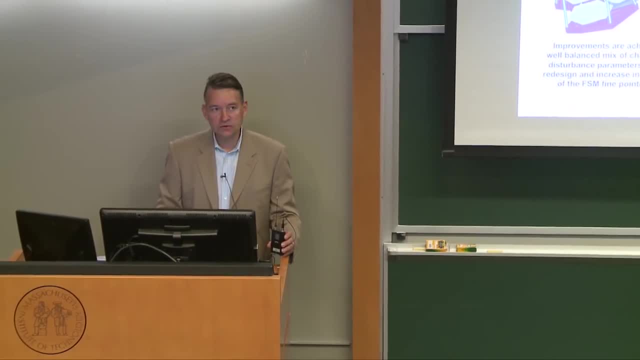 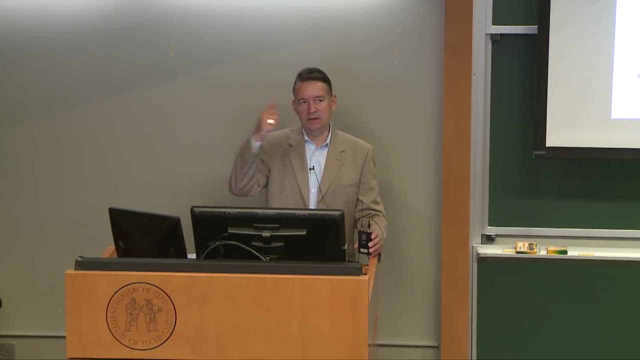 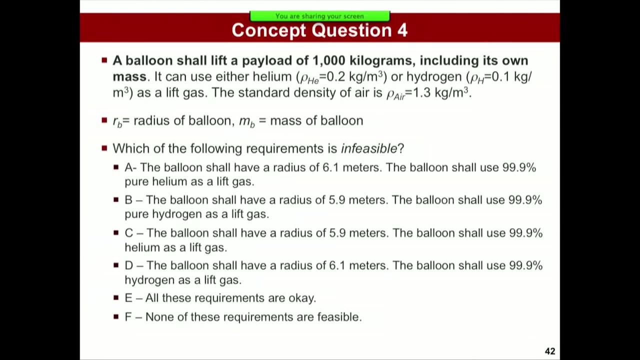 But you know we can handle that computationally. So you have to do some simulation and computation up front to make sure you pick. These requirements are not just wild guesses. They're actually based on some calculation and simulation. Okay, All right. 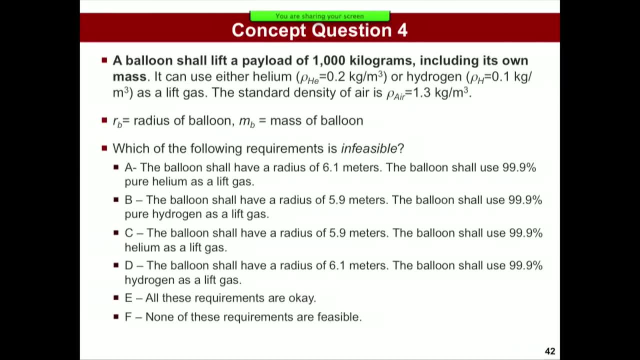 So here let's do this in a kind of simplified way. This is going to be our last concept question for today. Here's the higher-level requirement is a balloon. Those of you that have done unified engineering here, you've done this right. 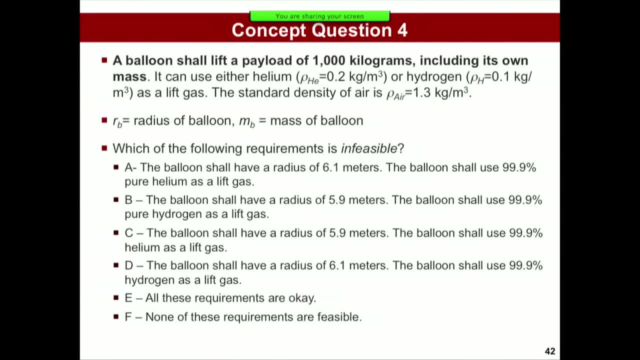 We did this in unified. A balloon shall lift a payload of 1,000 kilograms, which includes its own mass. You can use either helium, which has a density of 0.2, kilograms per cubic meters. This is in standard atmospheric conditions. 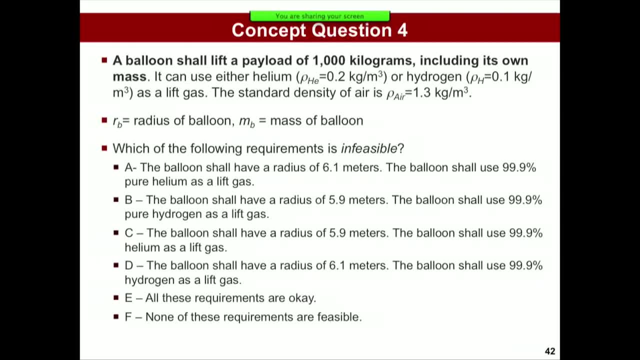 Or hydrogen, 0.1.. I've rounded these numbers. As a lift gas, the standard density of air is 1.3.. Which of the following requirements is infeasible? A. the balloon shall have a radius of 6.1 meters. 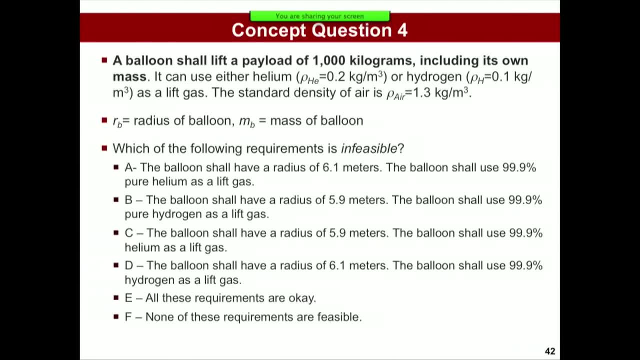 and the balloon shall use 99.9% pure helium B a radius of 5.9, and the balloon shall use 99.9% hydrogen as a lift gas And then 5.9 meters helium, 6.1 meters hydrogen. 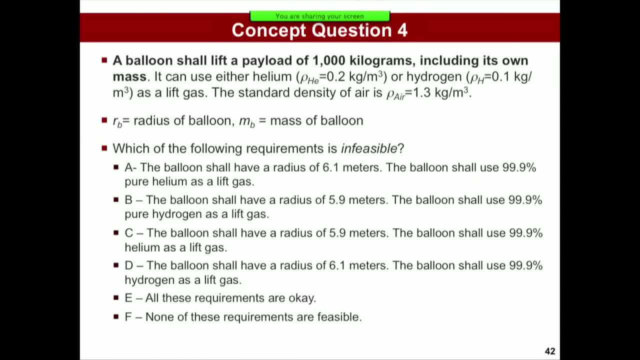 E. all these requirements actually are okay, Or none of these requirements are feasible, Okay, So I'll give you three minutes to try and figure this out And then I'll show you the solution. Don't cheat. Don't go to the next chart. 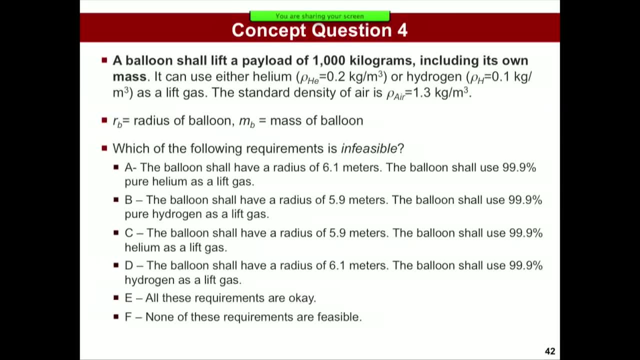 So think about this. The high-level requirement is the balloon shall lift 1,000 kilograms, including its own mass, And we're trying to allocate lower-level requirements for the size of the balloon and the gas that we're going to use. So try to figure this out. 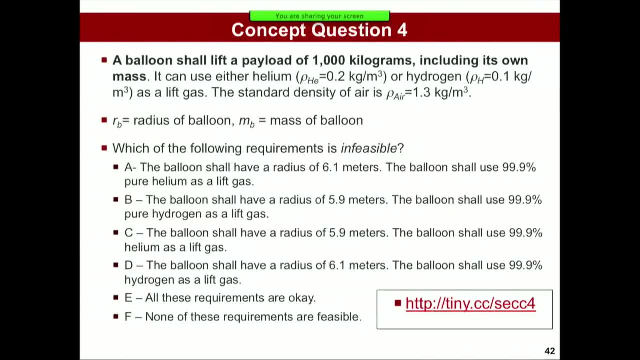 All right, I think we probably need Who needs more time for this? Okay, So we're going to leave this as a cliffhanger. Okay, We'll do the solution next time And take a little time to figure this out. 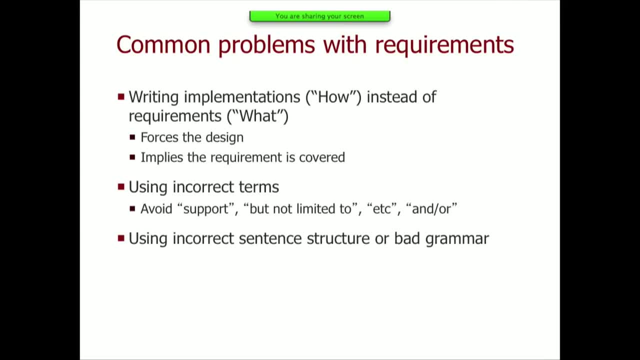 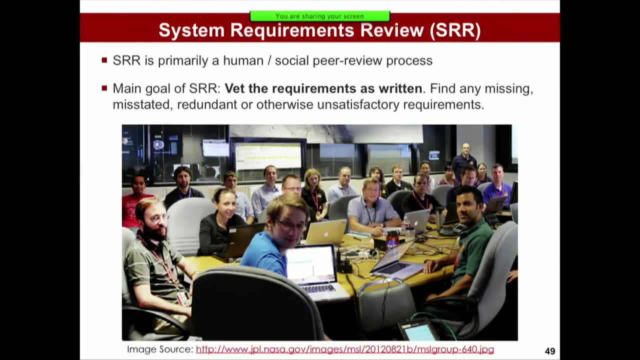 Try not to look at the next slide. Okay, So I'm going to skip this just for time, And I want to talk briefly about the SRR, what it is, and then kick off assignment two. So SRR, So the idea is: you've really been working. 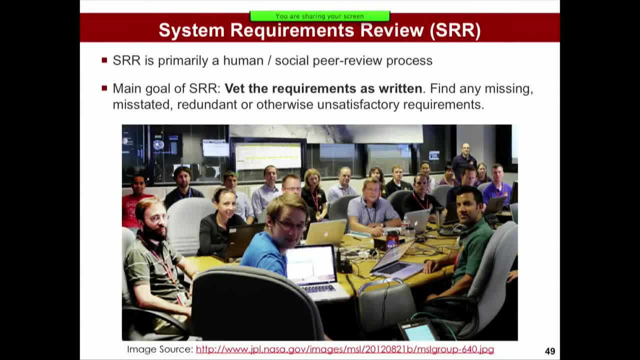 on these requirements hard, you know, as a team with your customers, And this takes. This is not a quick thing. This is not just two or three days Typically. writing your level zero, level one requirements is a process that takes weeks, months. 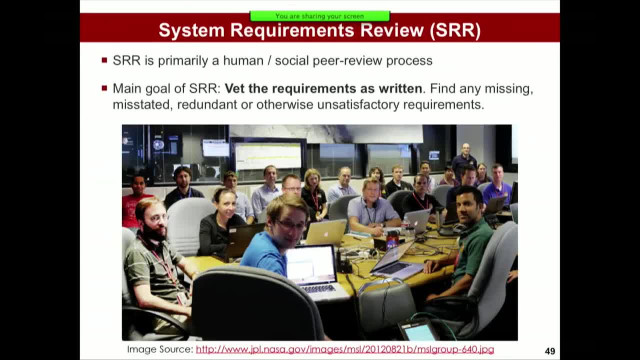 sometimes at least a year, But typically it's on the order of, you know, three to six months in many projects, roughly. And once you have your high-level requirements, SRR is the milestone where you review those Right. So here's an example. 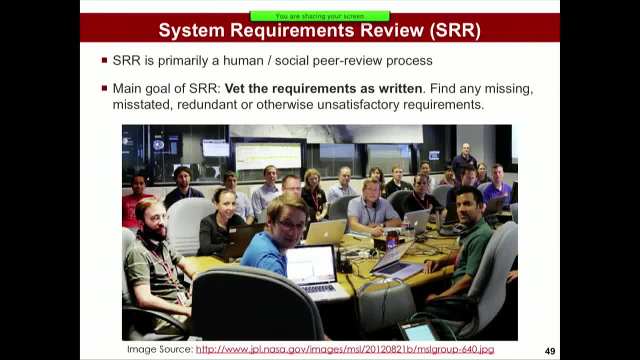 So it's a social, It's a peer review process And the main goal of SRR is to vet the requirements as they were written to see if you have any missing, misstated, redundant or otherwise unsatisfactory requirements. This is a picture from JPL. 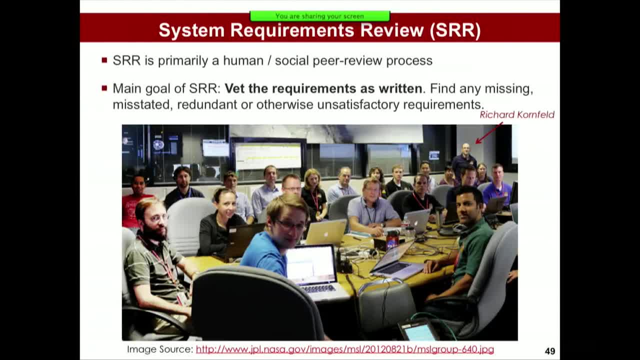 from MSL actually mission. And I want to just point out a good friend of mine who's a graduate here of our department, Richard Kornfeld Volker knows him, met him last summer. He's been working on three different Mars missions. 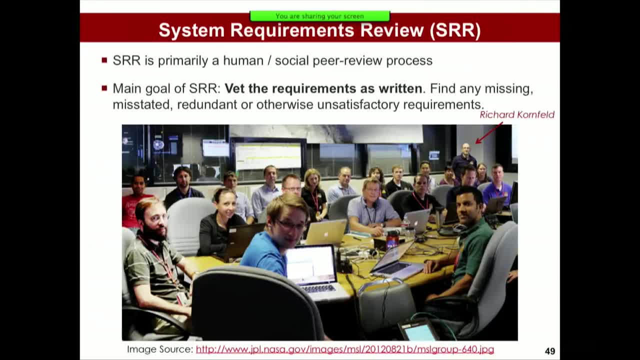 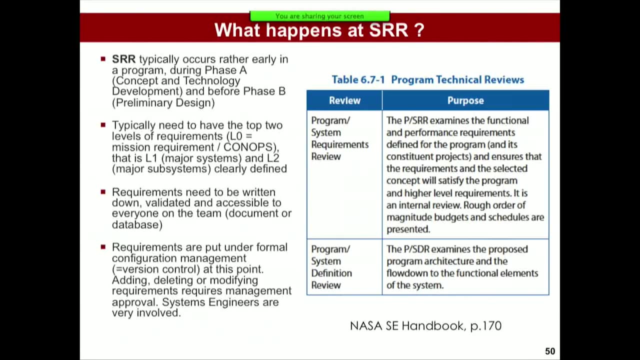 over the last decade And we're going to hear from Richard later this semester about verification of requirements, because he verified the entry, descent and landing requirements for MSL. So here's essentially what it says in the NASA handbook. SRR happens during Phase A. 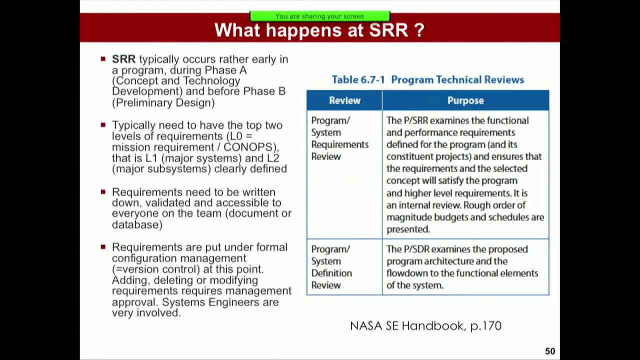 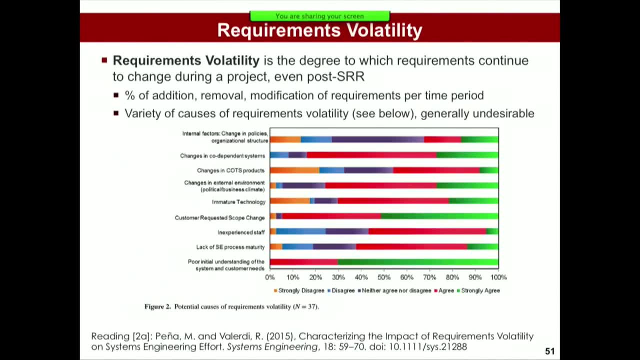 before you go into Phase B And you need at least your top two-level requirements written before you can do the SRR. I do want to mention the second reading post-reading. This is about requirements volatility. So just because you passed the SRR, 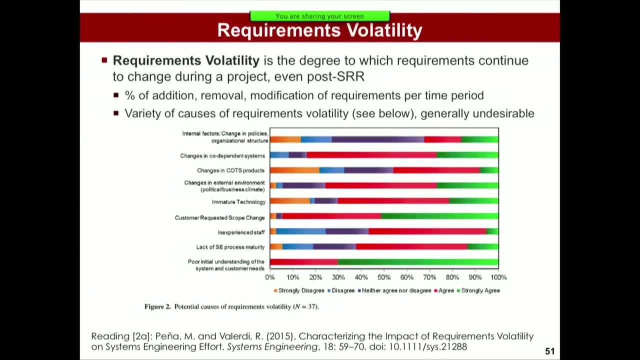 doesn't mean that the requirements are completely frozen. First of all, you don't have a lot of lower-level requirements yet. right, Those are going to be added post-SRR, And even some of the You pointed out, some of you. 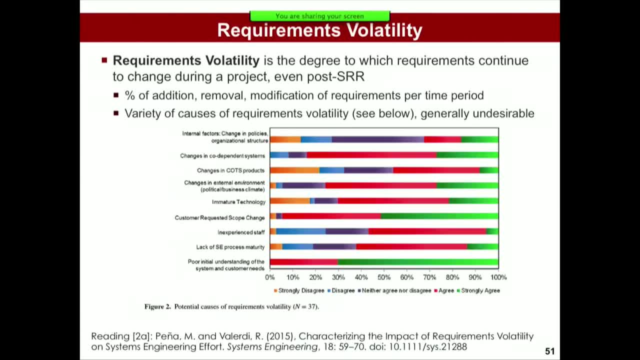 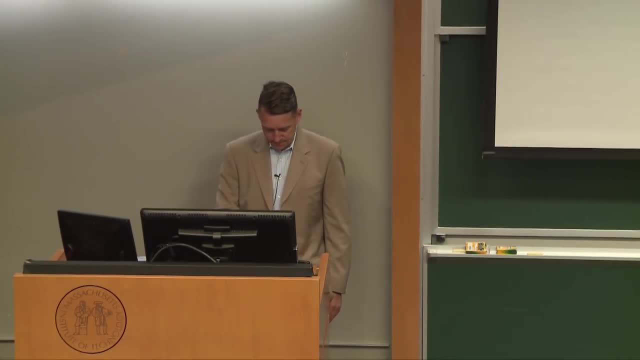 the requirements creep and these things. So this second reading is about requirements volatility, which you can actually quantify. What are the sources of requirements volatility? That's what this figure shows you, And then what is the impact of requirements volatility? What is the impact of requirements volatility? 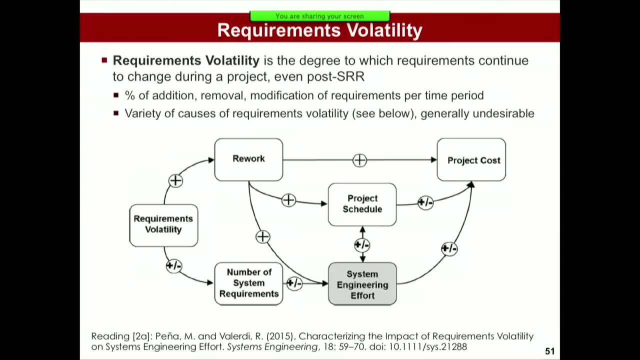 on a project, So specifically, you know, on the number of system requirements, on rework, on project schedule and so forth. It's really It's a very, very recent paper on requirements volatility. So let me just kick off Assignment 2,. 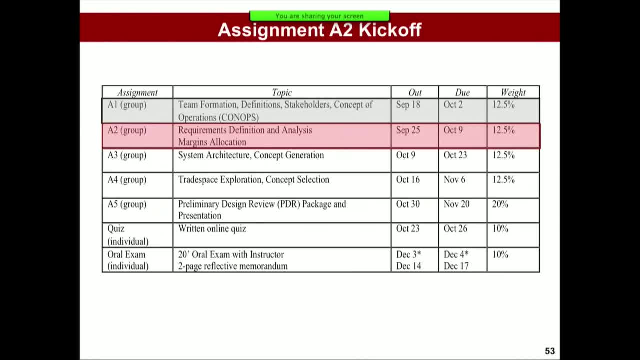 and then we'll be done. So Assignment 2 goes out today and is due in two weeks- so that's October 9th- And it's very focused on requirements, Basically what I want you, And it's the same teams that you're in. 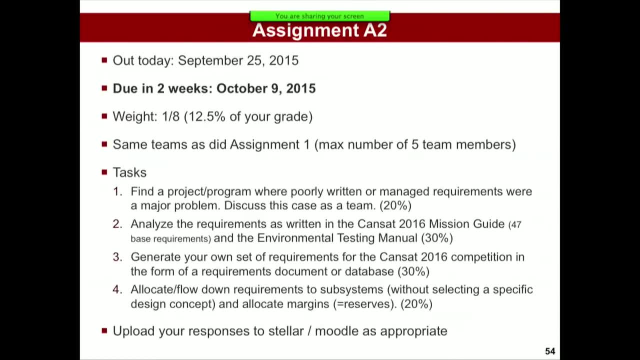 for all the assignments is essentially: first of all, the first task is find a project or program where poorly written or managed requirements were a major problem. So, as a team, discuss an example and discuss that example as a team. The second task is: 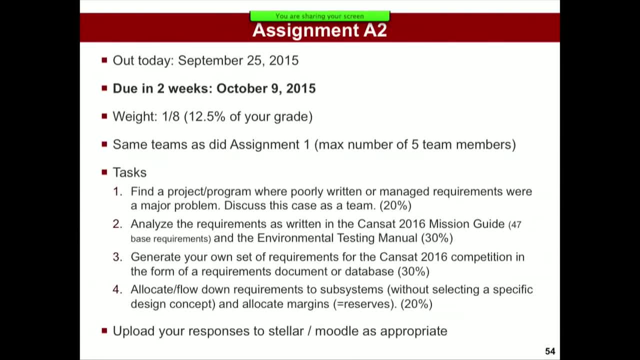 look at those CAN-SAT 2016 requirements, those 47 base requirements, and analyze those critically. So that means you know are they feasible, Are they well written, Classify them. You know what type of requirement is it. 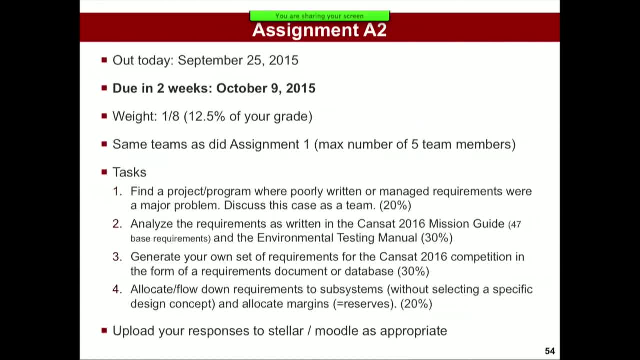 Is it an interface requirement, Is it a performance requirement? And then figure out whether there's a hierarchy there And basically then from that generate your own set of requirements for the CAN-SAT competition. So you're going to either rewrite: 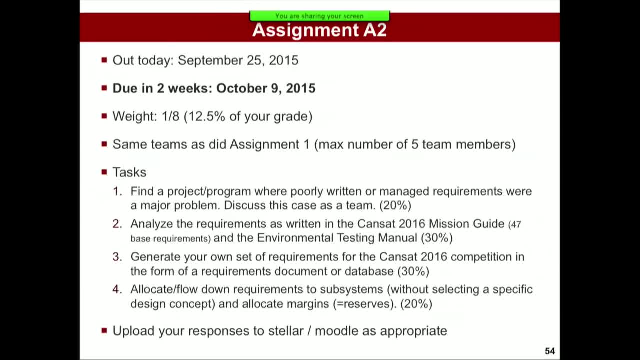 or reorganize these requirements in a way that's better and that works for you as a team. And then the fourth requirement is to figure out where you want your margins, where you want, Where do you think you need to have reserves and margins in these requirements? okay, 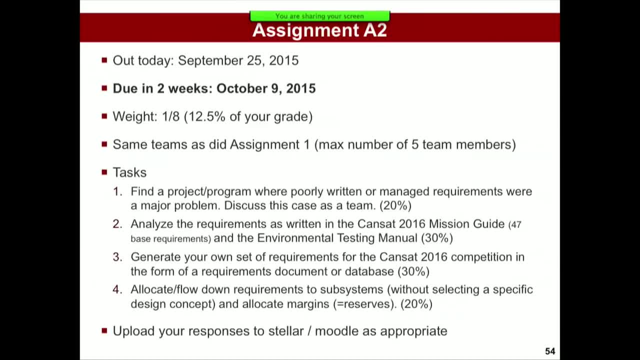 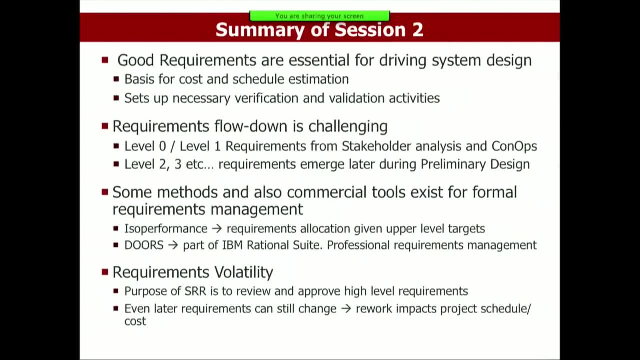 So it's very much looking and reorganizing and critically analyzing the CAN-SAT 2016 requirements set. So let me summarize: You know good requirements are really essential. It's the starting point for system design, system engineering. It is a challenging thing.